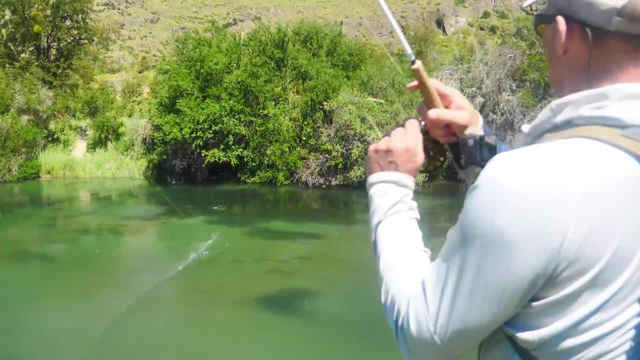 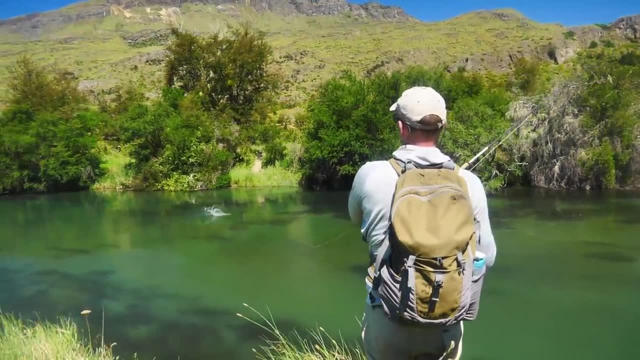 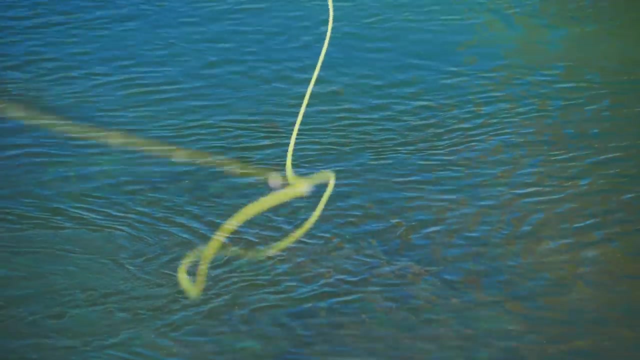 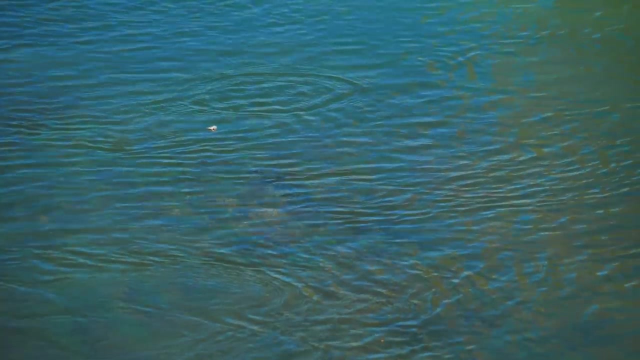 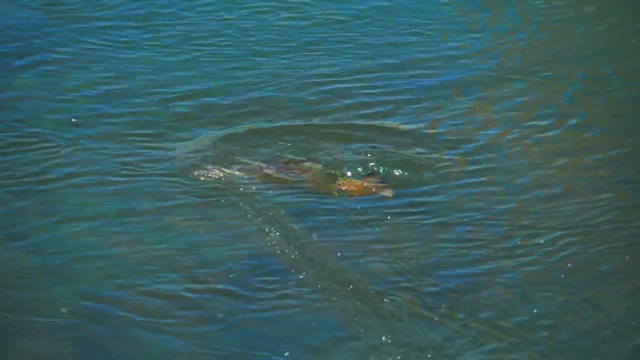 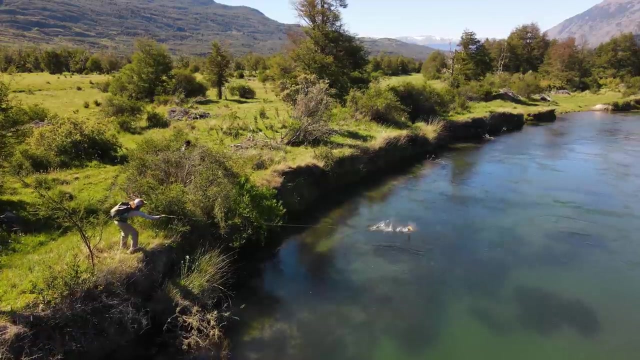 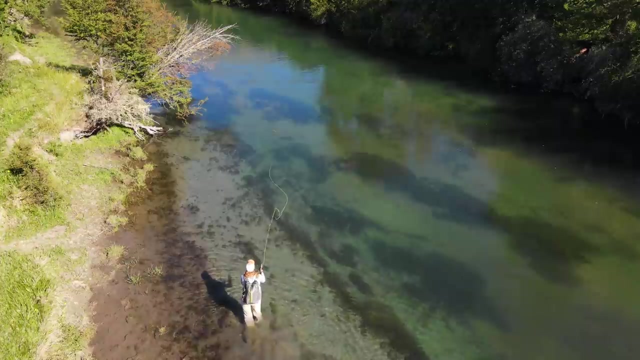 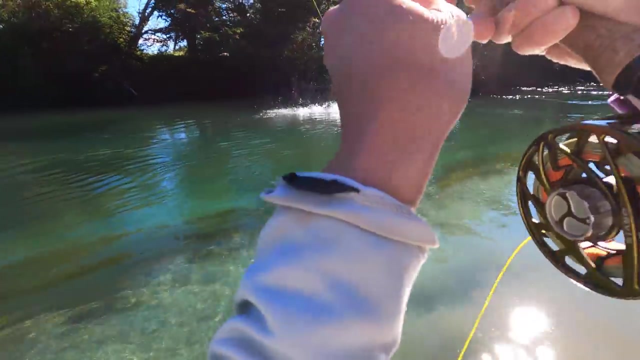 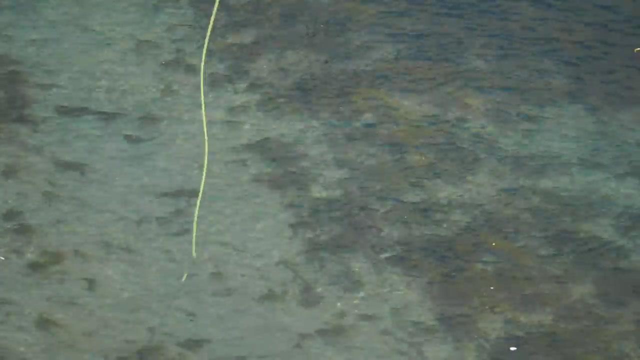 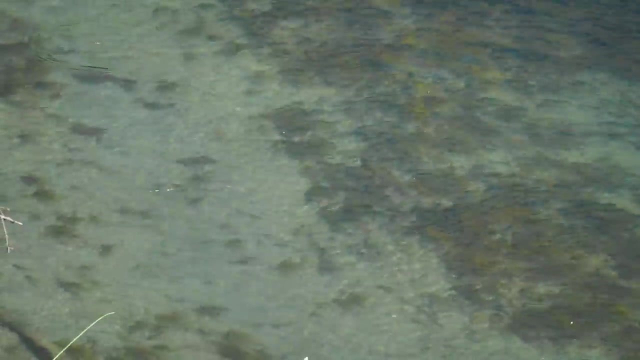 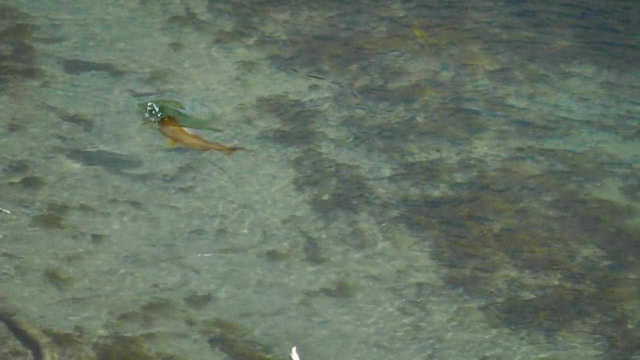 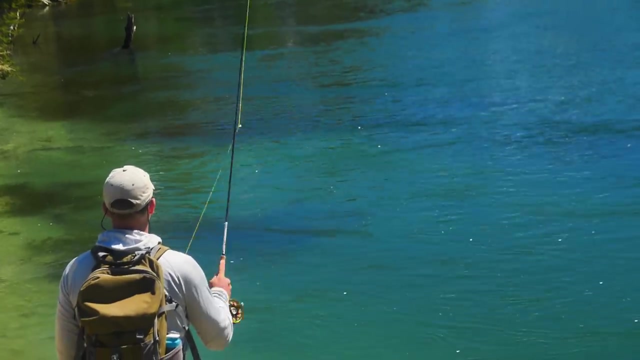 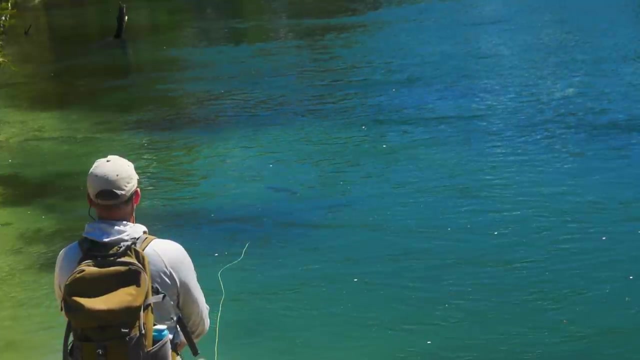 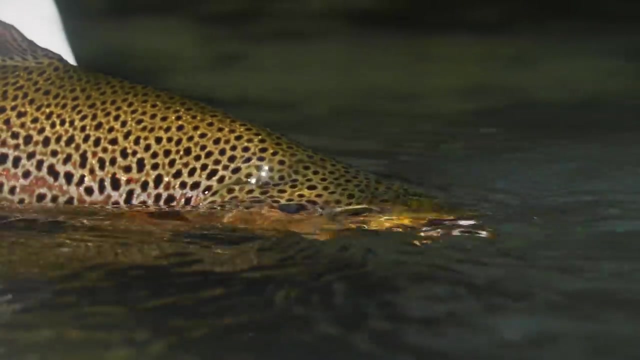 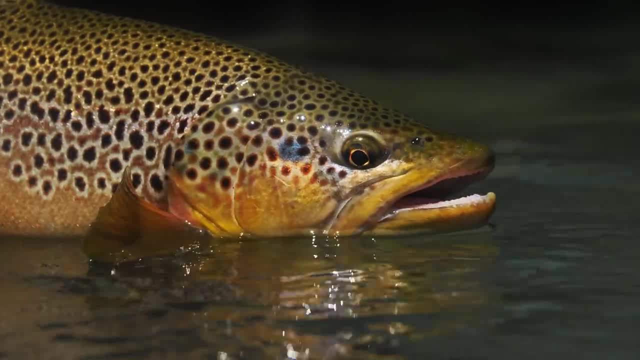 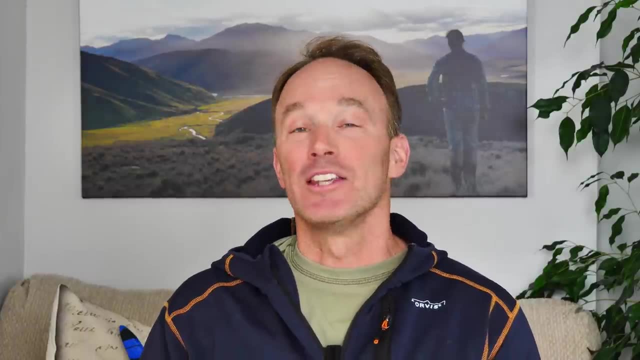 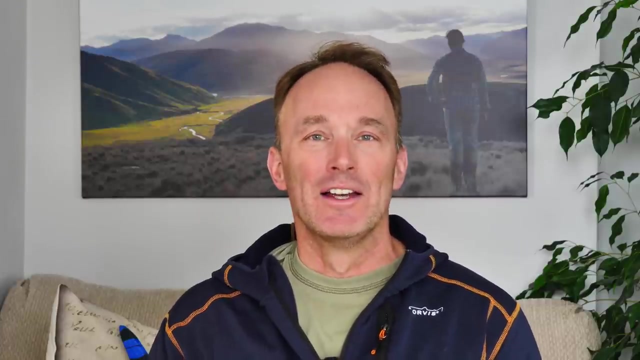 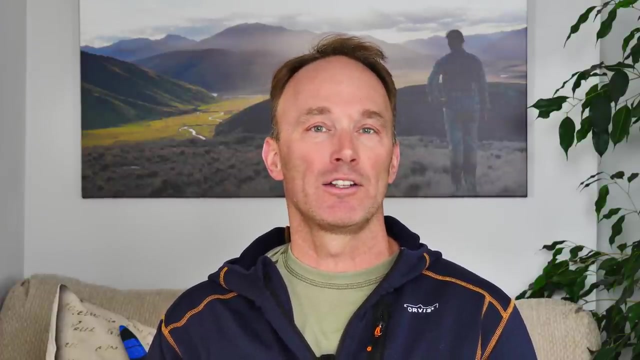 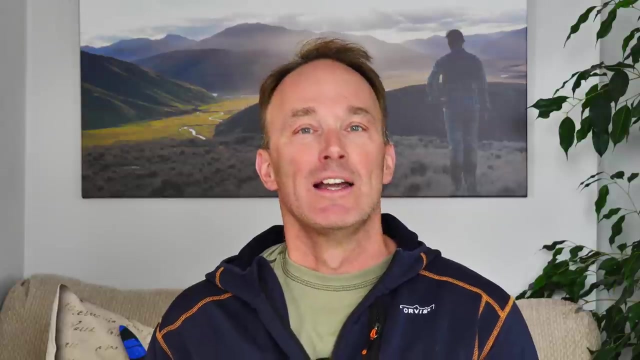 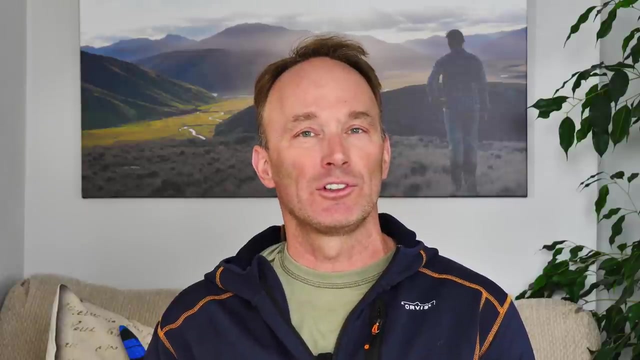 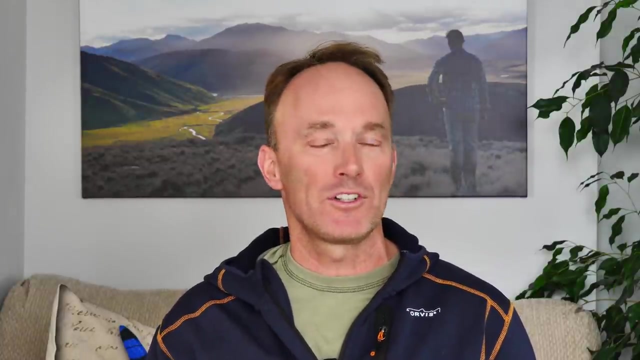 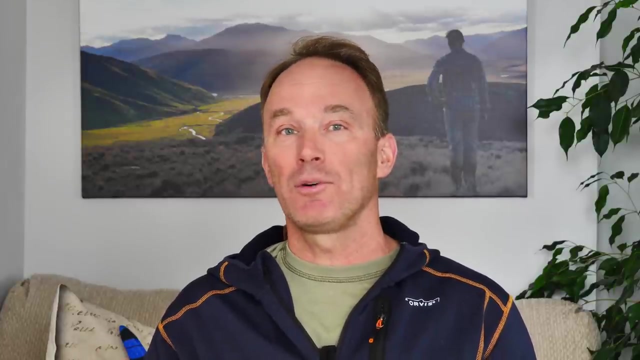 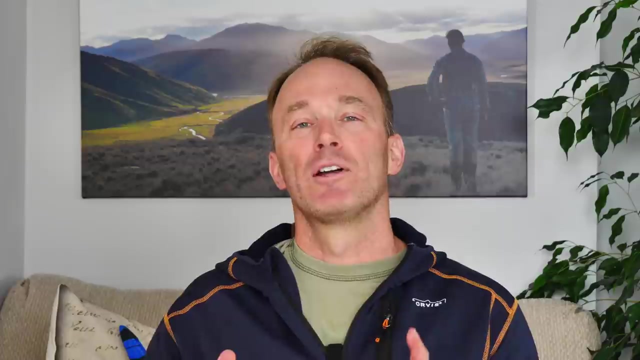 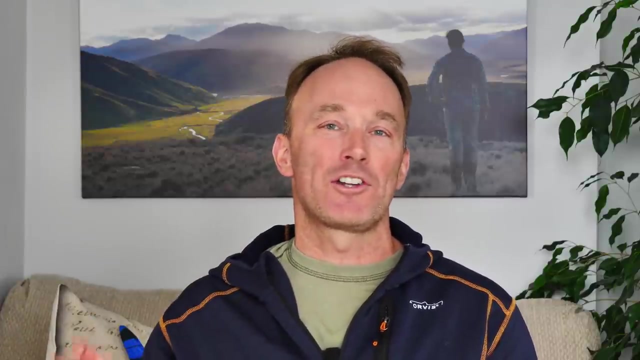 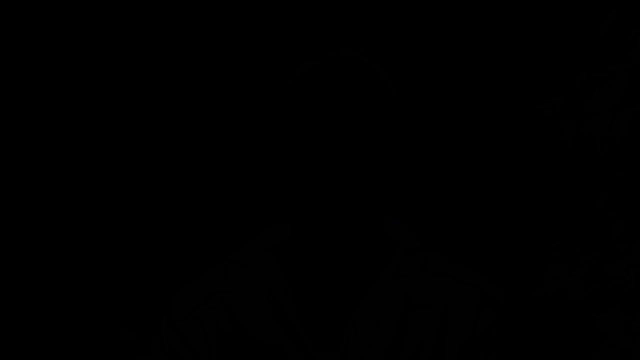 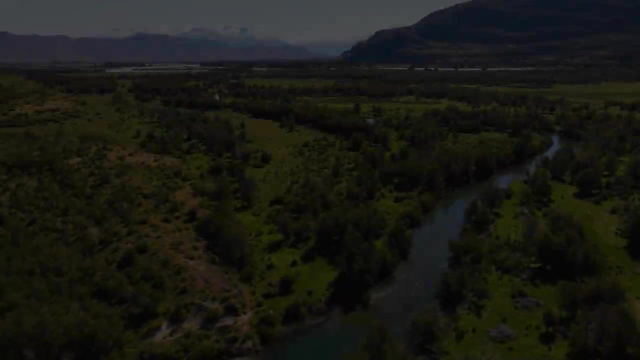 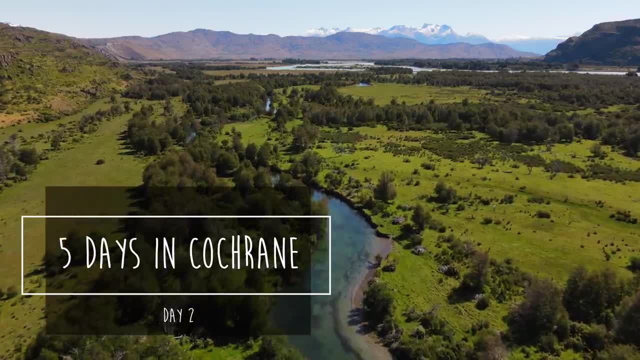 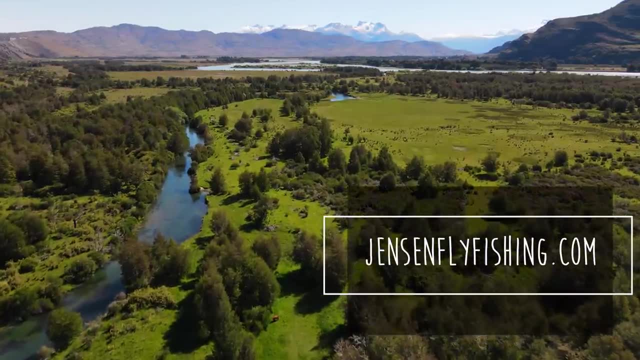 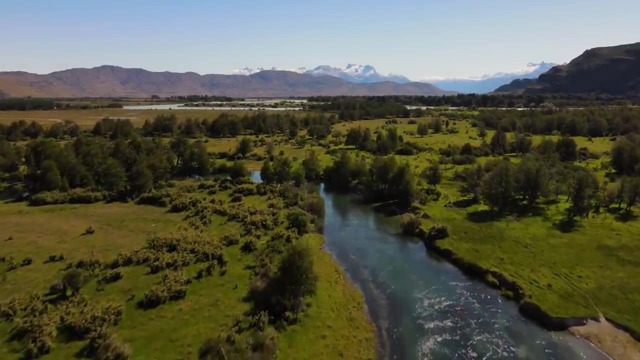 The second day had a feel- Waking to clear, calm skies and no wind in Patagonia is special. We've seen this exact day so many times and each one is magic. You don't forget them- Where yesterday was a day of working to get fish of interest on camera. 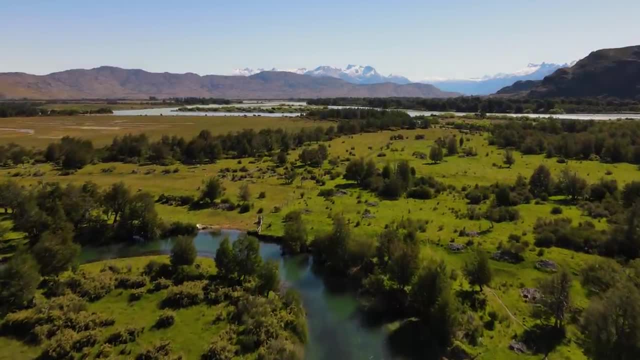 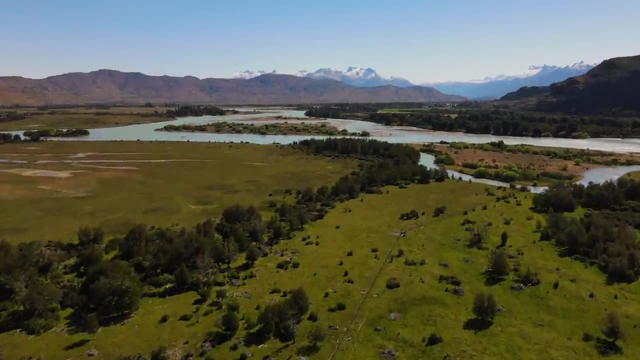 today. well, today was simply a day where Marcelo could spot brown trout and we'd catch it, See it, film it, catch it magic. We stuck to our guns all day. We didn't make a cast unless we found a fish that was able to be filmed and cast to. 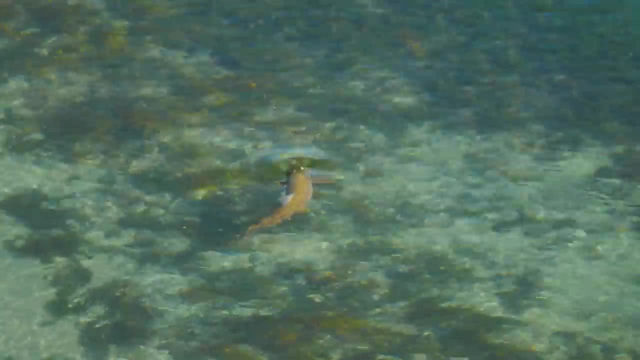 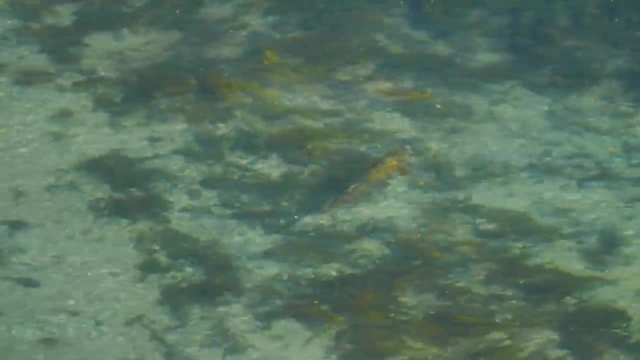 If it wasn't a neat video fish we moved along The river was exactly what we knew about brown trout. This was the day we'd been waiting for the entire trip, While we loved being on a different water every single day of the trip for 10 weeks, 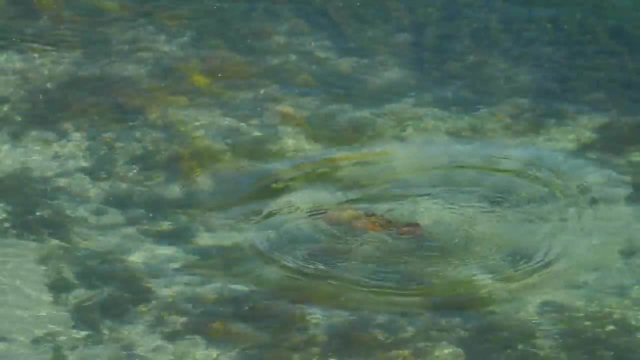 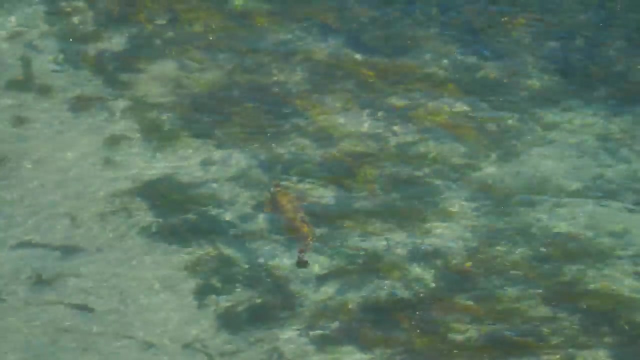 this was our day to dig in and do what we do. We were simply looking to dissect a brown trout river. We did exactly that. It was nice to be back at the beach at the Betty podcast show where we talked about the美味 theflavor that white shark did with its u, According to what I heard. 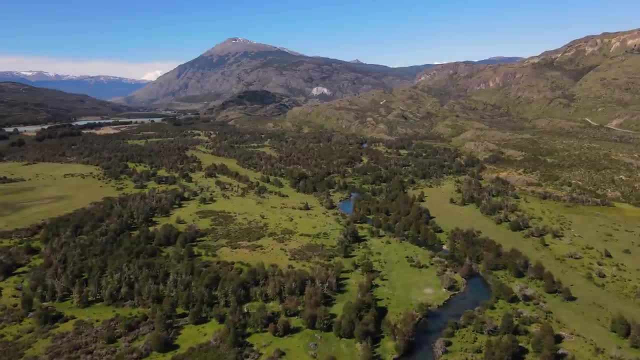 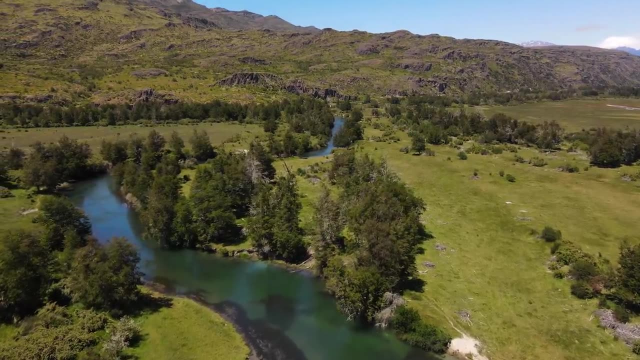 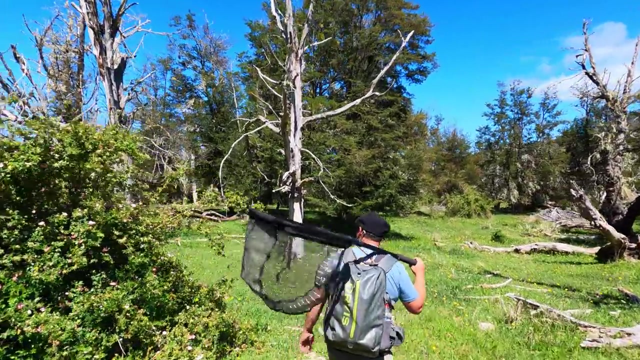 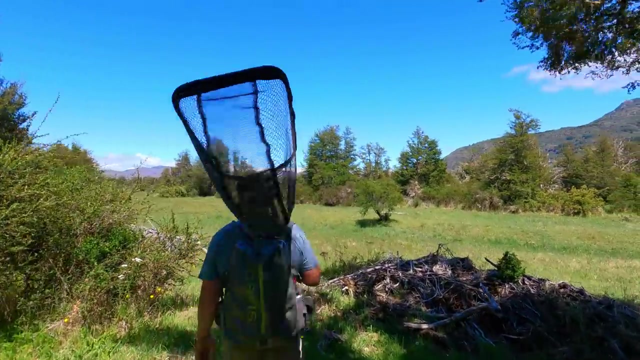 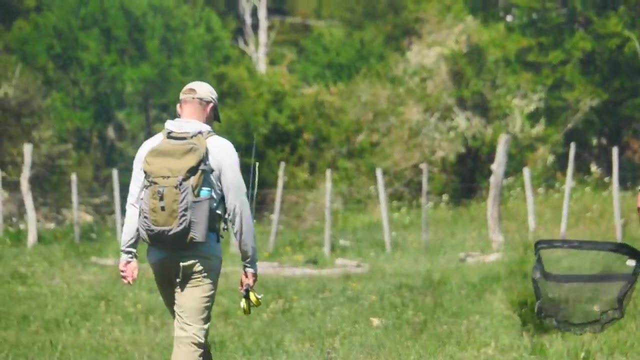 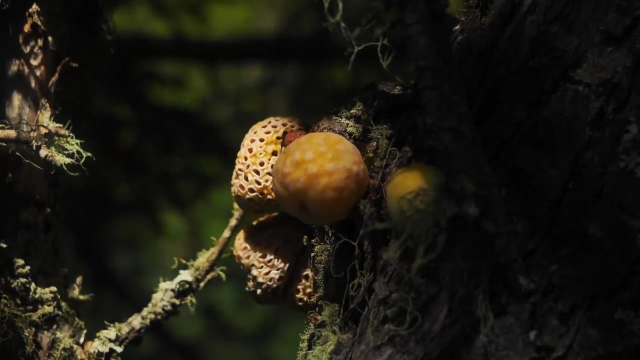 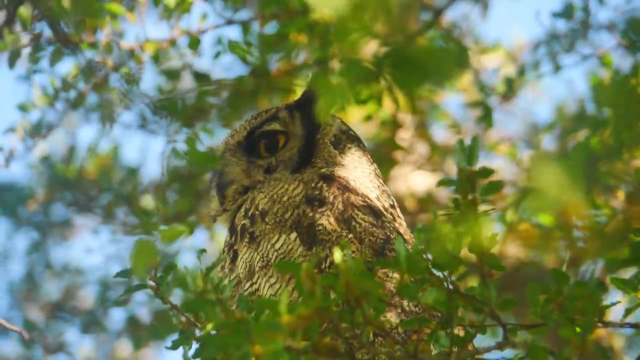 it was jokes, but lovely. I've learned from the rest to live together, to know one another and to be together as well. But and then we didn't hang out over dinner all together. It's okay. It's okay, I don't know. 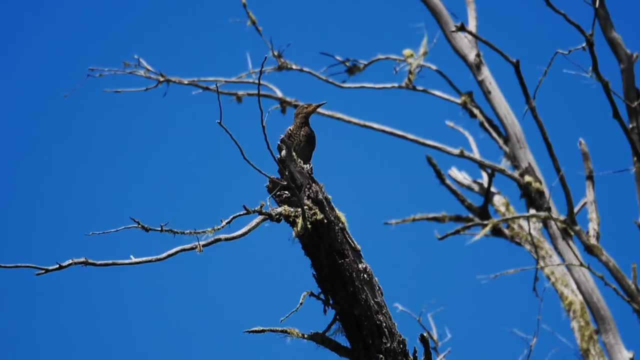 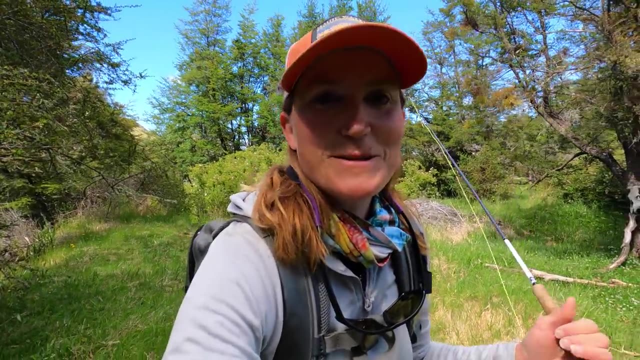 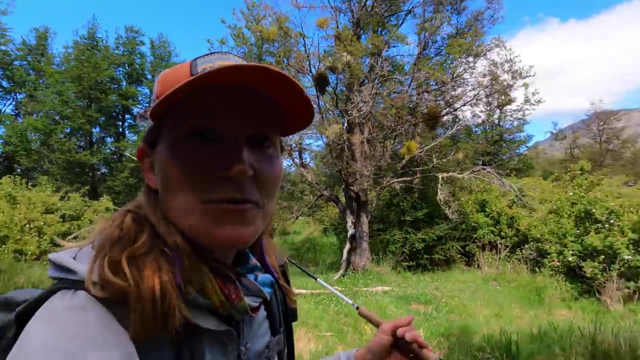 You guys. so we've got a brown trout that we spotted here from up on a high cliff bank right across from me up in there, And Dave's actually up there filming right now, And I've just come over with Marcelo and we're getting into position. 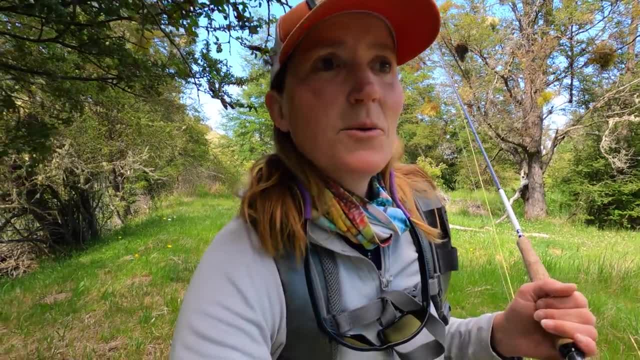 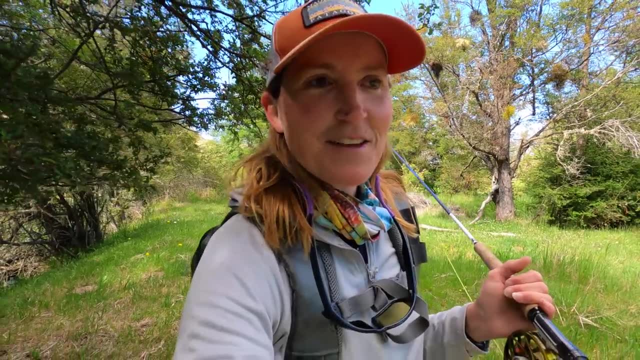 seeing if we can see the fish first ourselves and then we'll get into position and give them a try. Here is the first one of the day, A little different day than the other day, a little cooler morning, And he's risen. I guess a couple times we've seen. 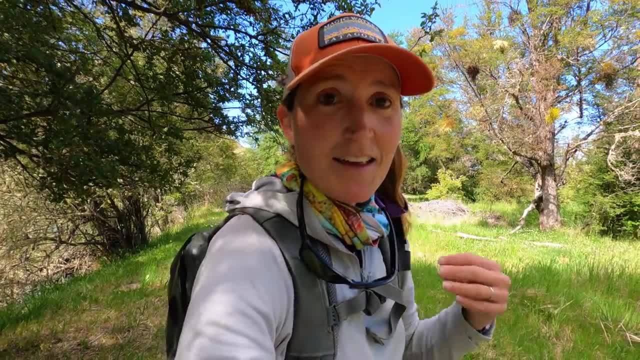 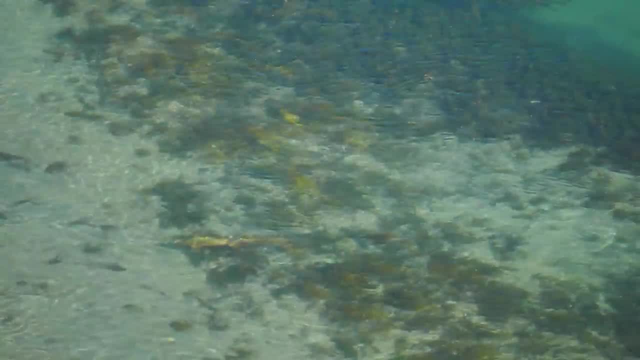 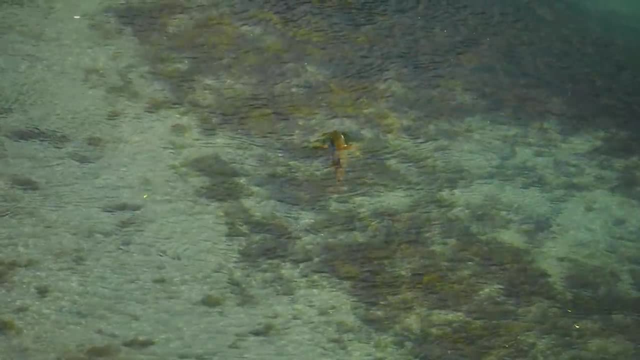 and Dave can definitely spot him from up on the bank. So I'm going to see what I can see from my vantage and then we'll go from there. We're going to go up to the lake and then we'll head back over into the river. 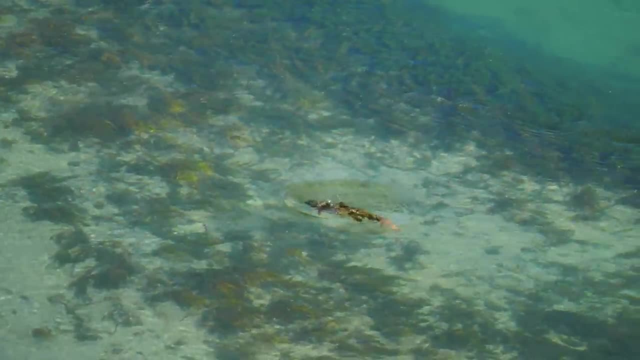 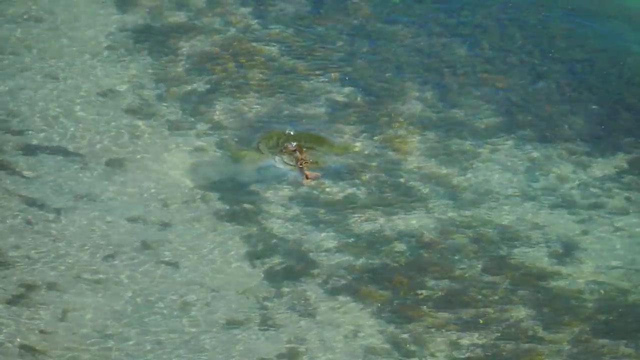 And what we can see is the tide being very low and we can see the lake age, And then we're going to take a short walk and then we'll come back here and we'll come back and see what a beautiful lake it's been. 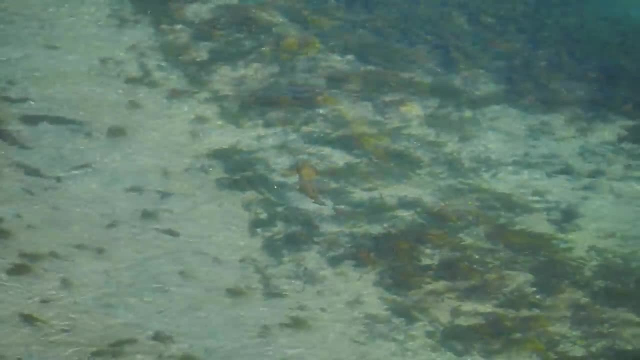 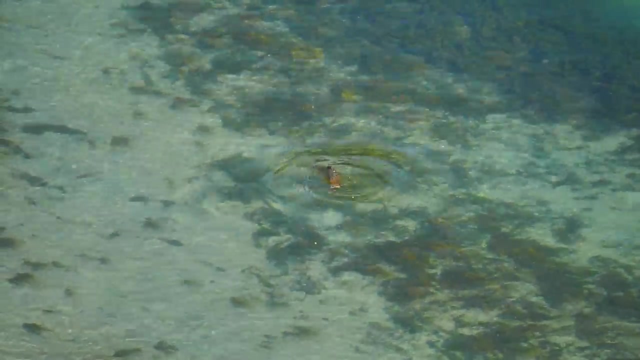 Oh, we can see the white trout. We can see the white trout and the white trout, and the white trout and the white trout, The red trout, are the fish? Yes, they are, They are. They're making their way back up into the lake. 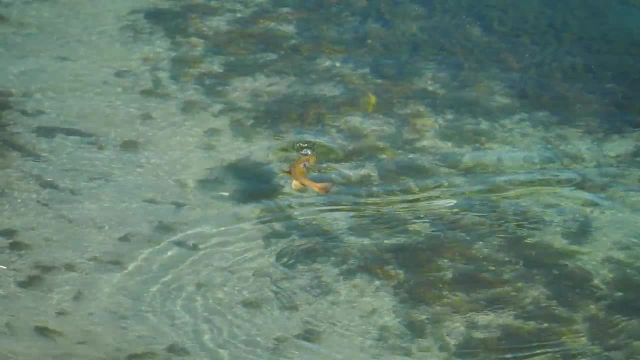 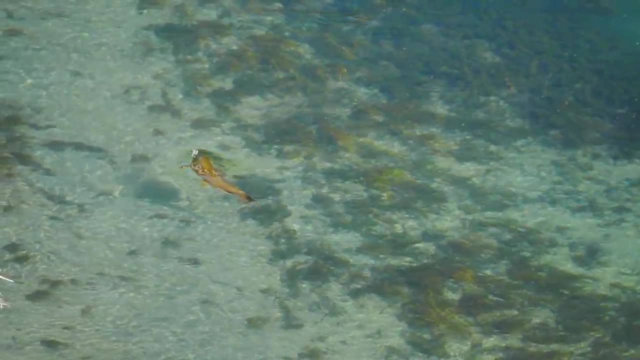 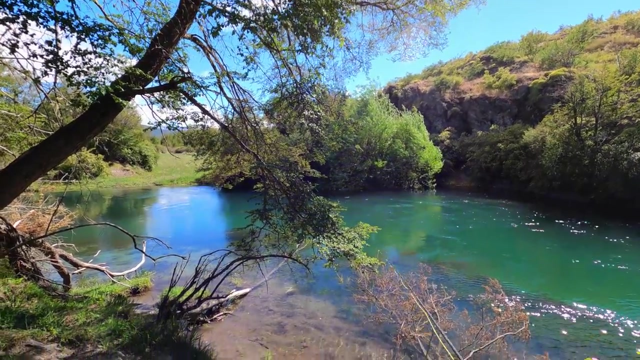 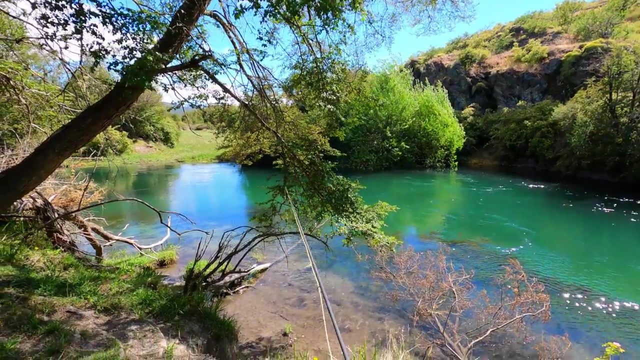 They picking the fish up. Yes, Yes, Yes, Yes, Yes. okay guys here, so i'm going to get into position. um, we figured out the spot that we think we need to be and hopefully it won't spook this fish. getting into that position should be okay because 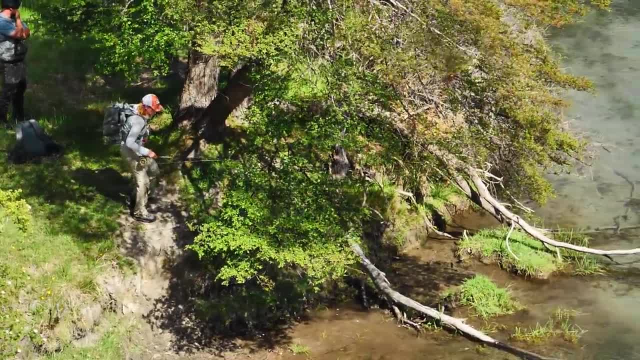 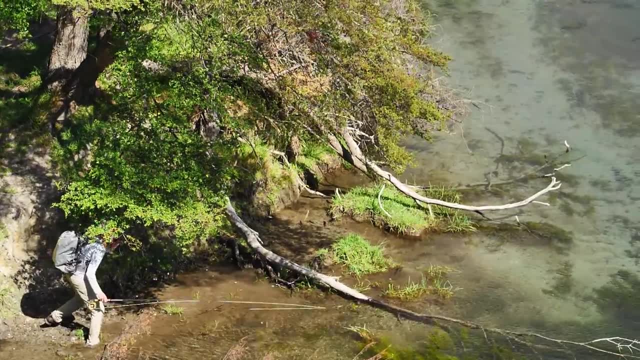 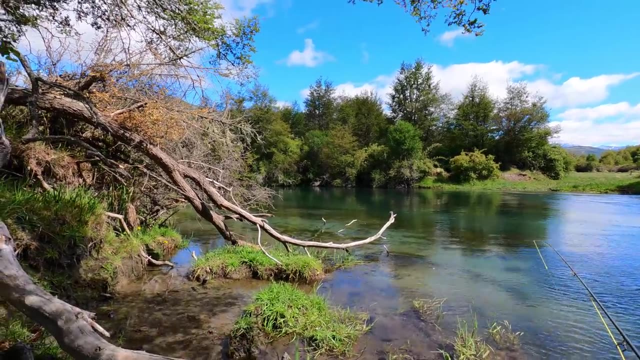 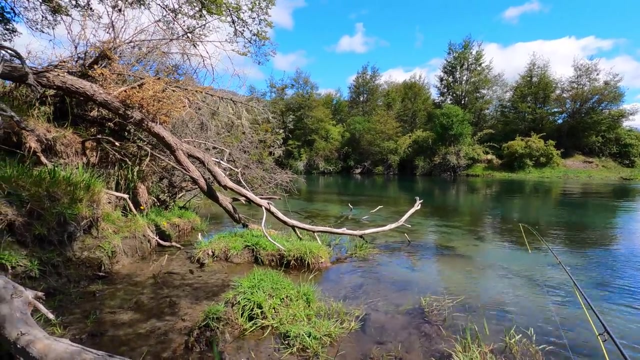 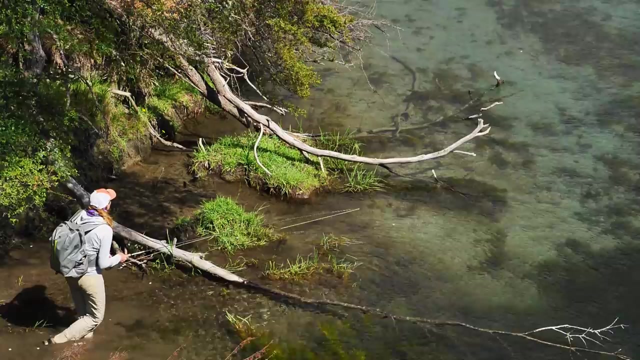 i know i'm well behind it. i think i see its tail just gonna get up. can i step a foot forward? yeah, yeah, i see its tail. rose petal is on its head now. okay, not doing much, but we'll see. so this fish isn't too far away from me, guys. i'd say it's you know, again maybe. 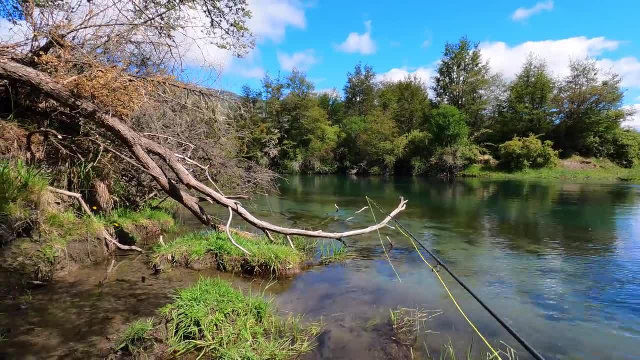 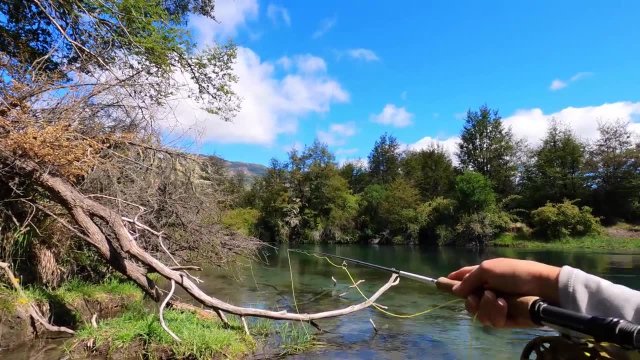 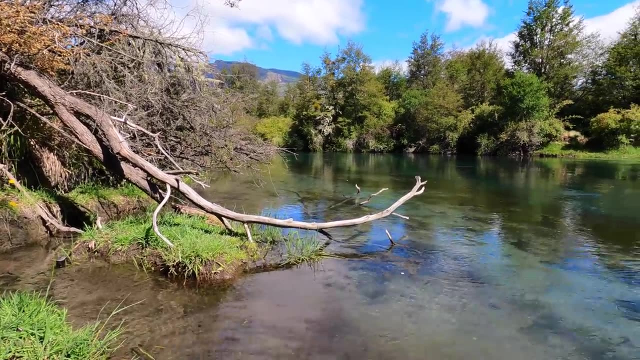 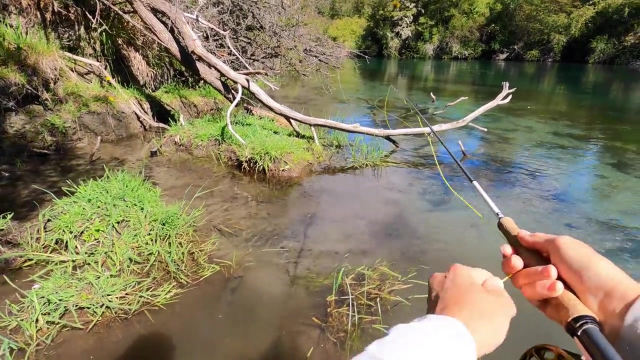 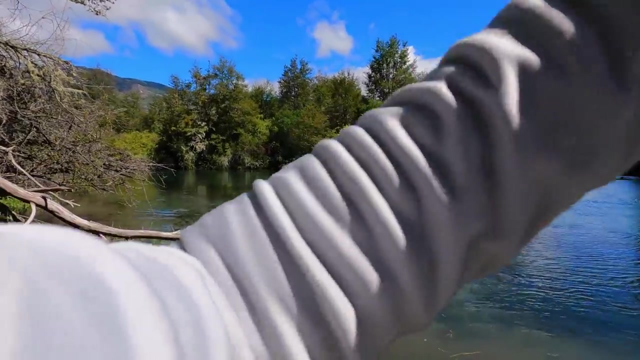 two and a half, three rod lengths and i've got to try to cast up to its left and i've got to make sure i don't hook this overhanging stick here. dave, these bunch of sticks off the bank, i'm going dave. yes, got him. nice, nice, nice. come on, fish, come on, i'm going dave. 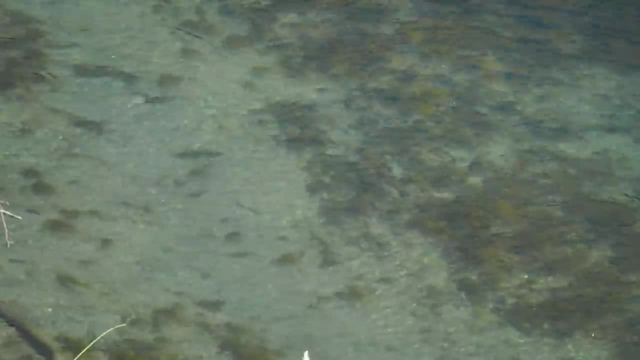 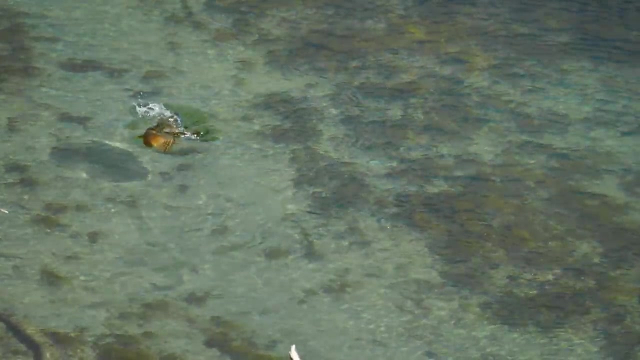 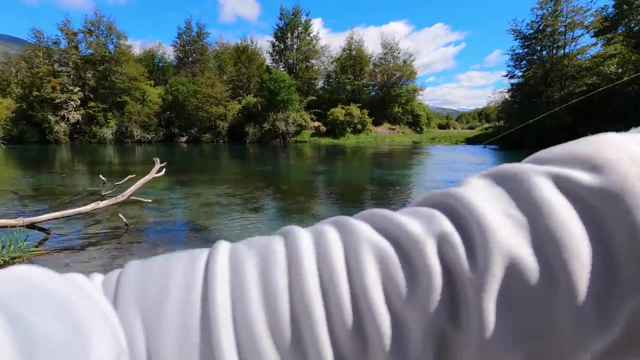 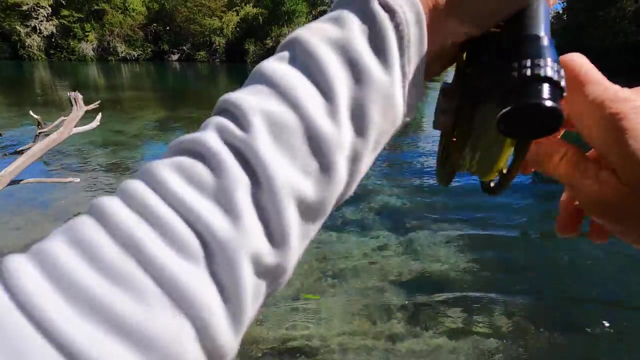 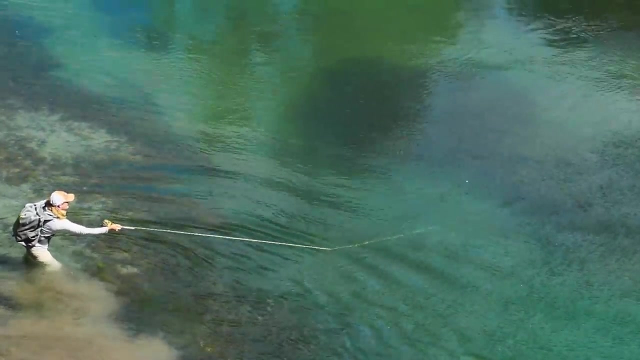 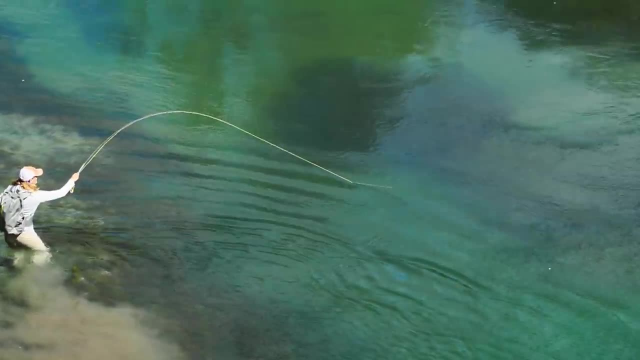 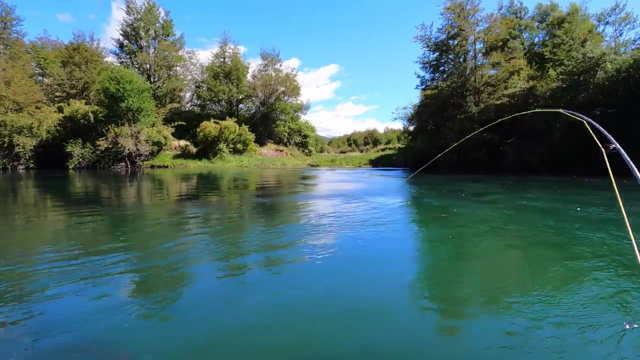 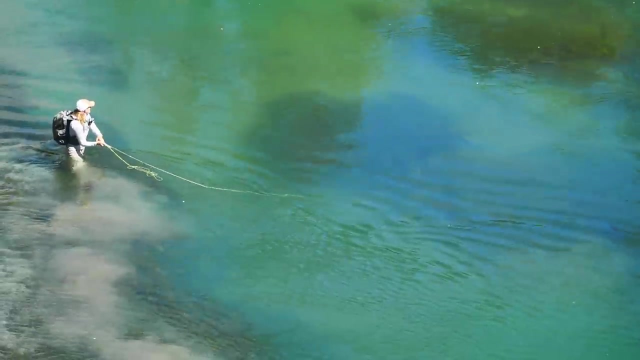 yeah, it's probably a non-starter getting this fish guys, because he just tore into a big weed bed over there and i can't feel like. all i feel is a ton of pressure, the weeds, the current. i still feel him, he's, i know he's wedged, when you know a fish is rather wedged. 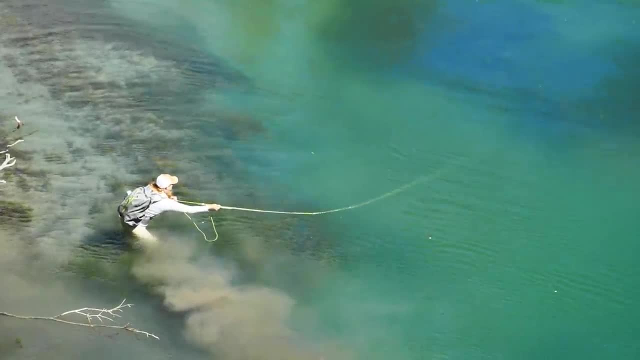 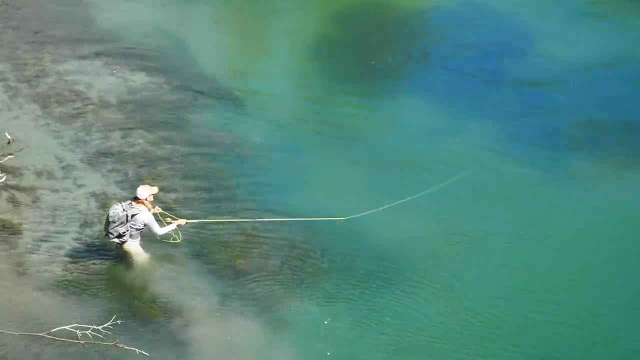 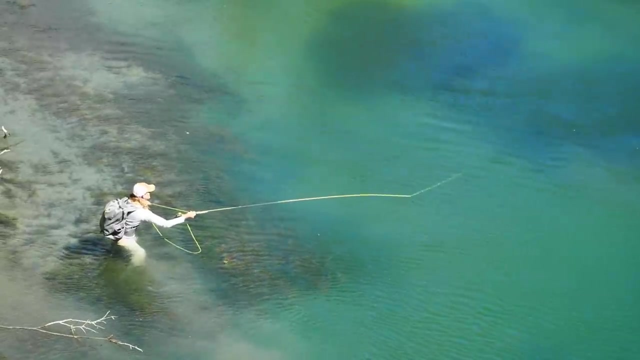 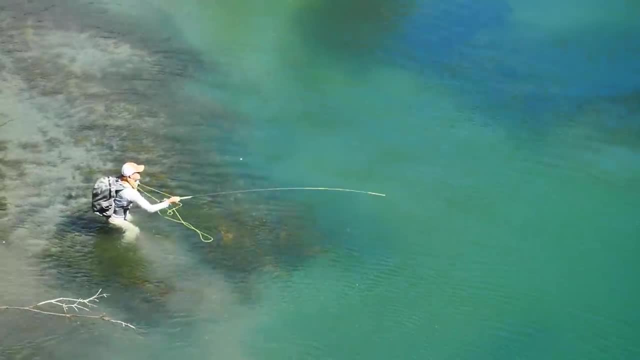 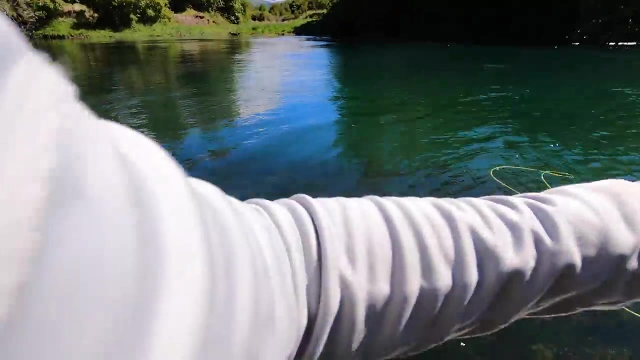 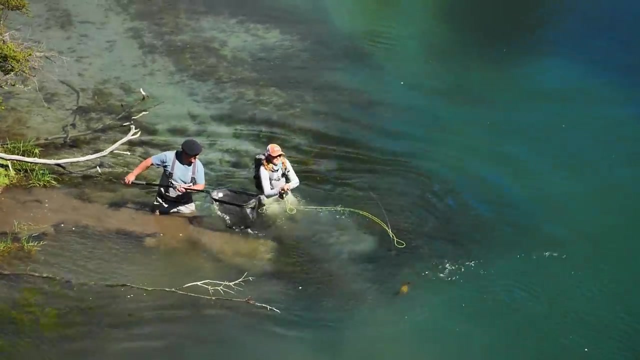 yeah, come on out, come on out, okay, okay, okay, we have a chance here. I don't want them too close in these weeds. no, no, no, no, no, no, okay, okay, okay, I try, hang on, let's try to bring them in here. okay, here we go. here we go, dig, dig, dig, dig. 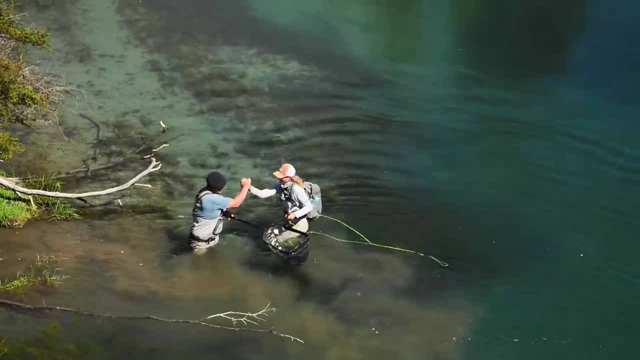 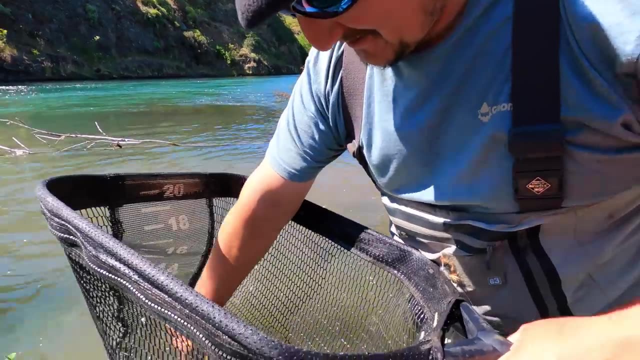 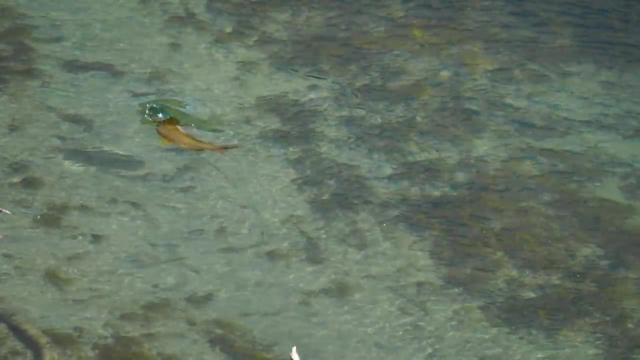 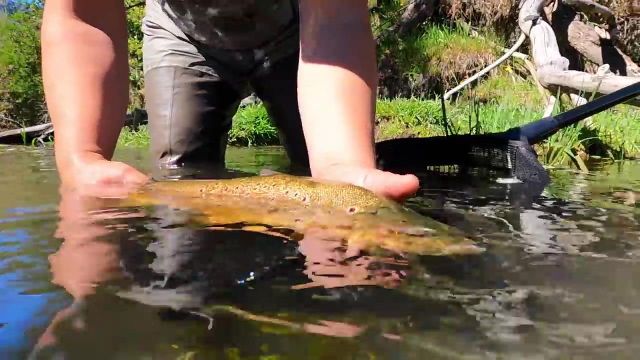 yes, Marcelo, thank you. yeah, man, patience, patience for me, patience. guys, you slowly want to come out. oh, that's awesome. yeah, what a fish, what an awesome brownie. love that eat. bring them out here. just bring the head out. beautiful, beautiful head up for me, yeah, gorgeous, I'm super stoked about that. 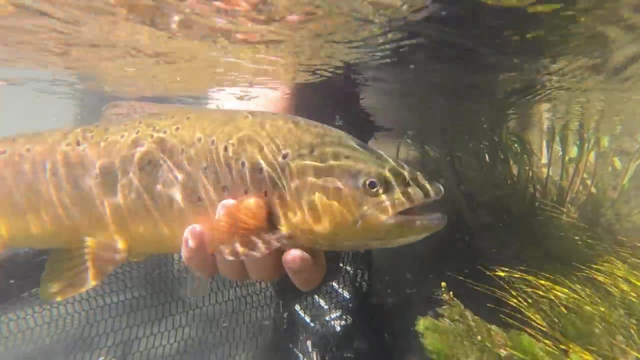 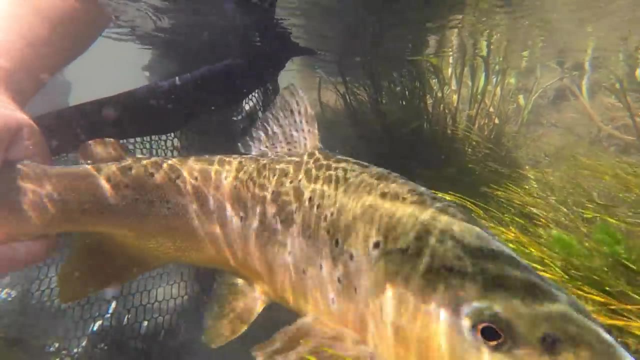 guys. what a beautiful place to get into position, only a couple rod lengths downstream. and then Dave and I had talked and, hey, I wanted to put my fly to his left, make him come to the fly, because it was on this beautiful light marl and and yeah, it worked out great. biggest thing, though, on that fight is 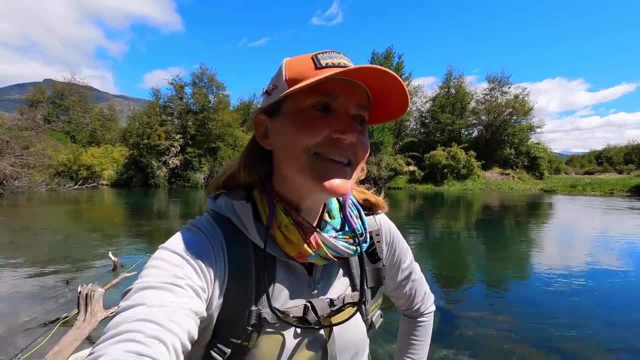 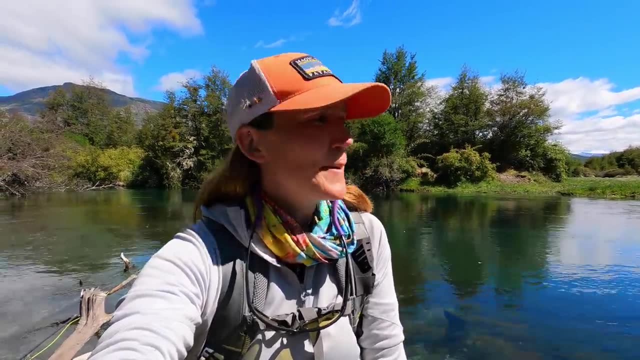 the patience thing. I got a little antsy after waiting for what felt like a little bit of time where my rod was downstream of that weed and I had kept the pressure and I could still feel the fish. you know, I'm not sure if that's a good thing or not. I'm not sure if that's a good thing or not. 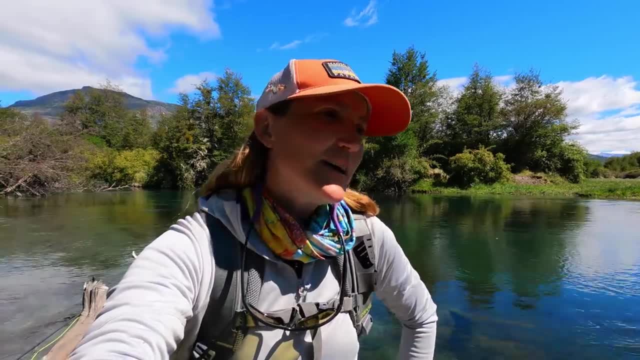 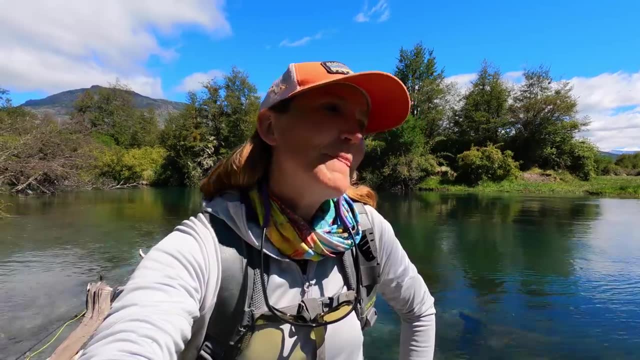 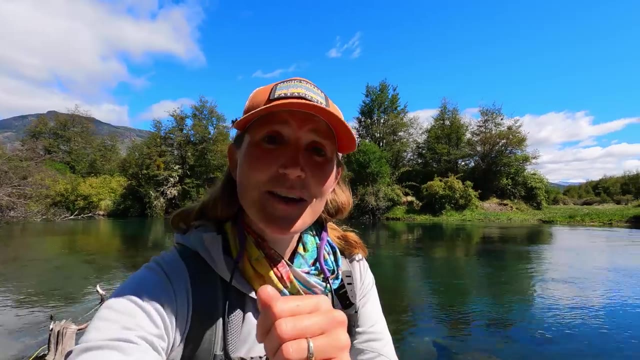 but it wasn't budging, nothing was happening and I thought, well, maybe if I try to get upstream of it, I knew you know you heard me saying that's probably not gonna get landed. well, no, I needed to give it just that much more patience because, eventually, what happened? I kept pressure, I kept lots of pressure on the 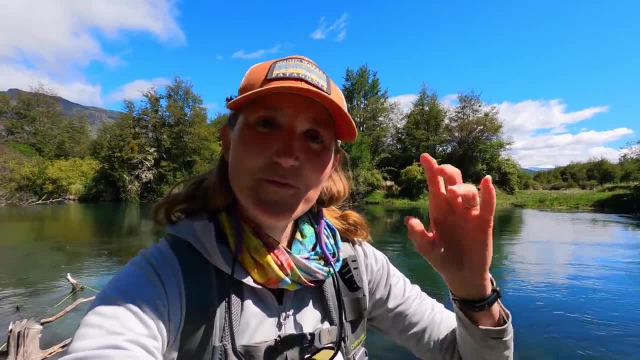 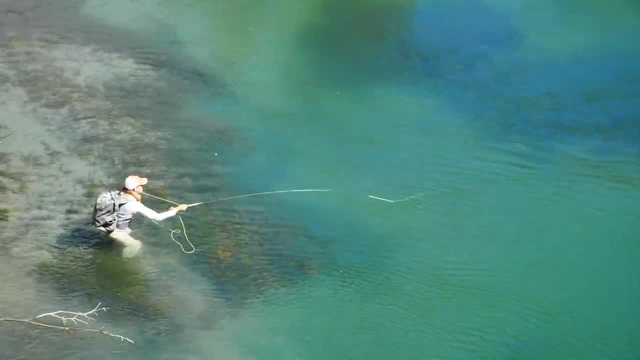 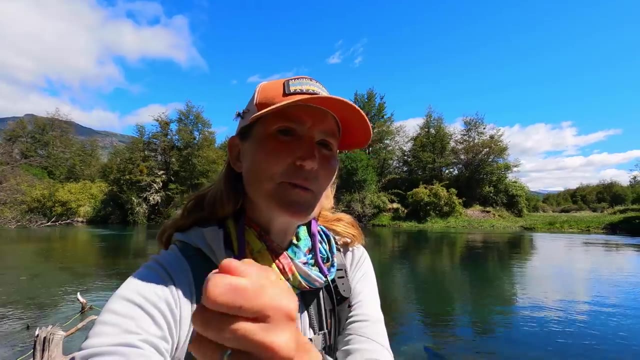 rod and the whole line and everything, and I eventually could feel that fish move and as he moved he was kind of loosening the weeds around him and I just kept keeping pressure, keeping pressure and, and as he moved I kept adding a little more pressure backwards, straight out from whence he came into. 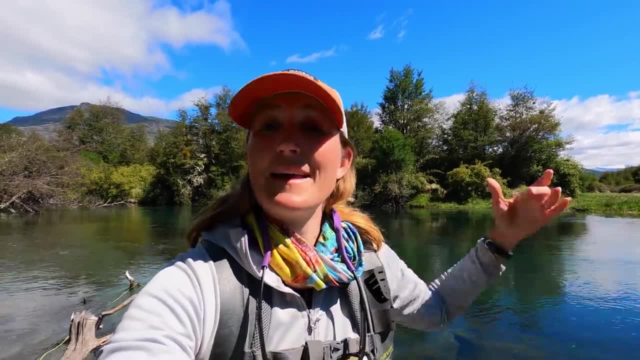 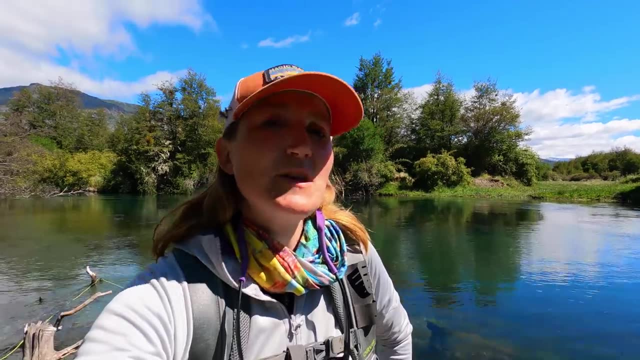 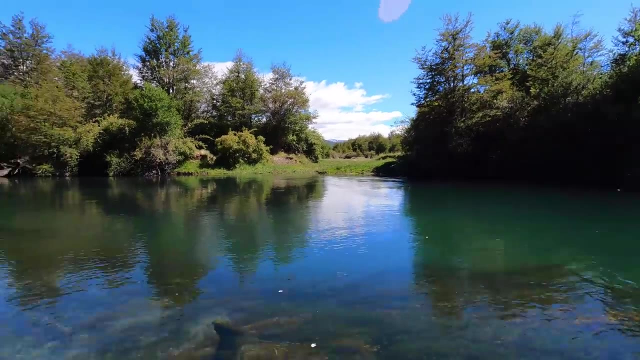 the weeds, because if you, if you try to do the angles against the weeds, it often doesn't work. sometimes you have to change position, but in this case those weeds are there. they're a big stretch of weeds that are just like this that you're looking at, but further out there and now that's. 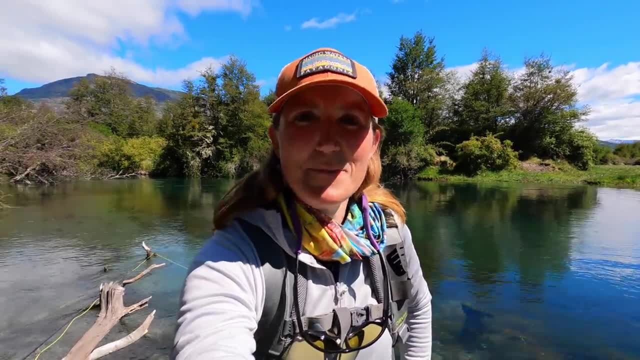 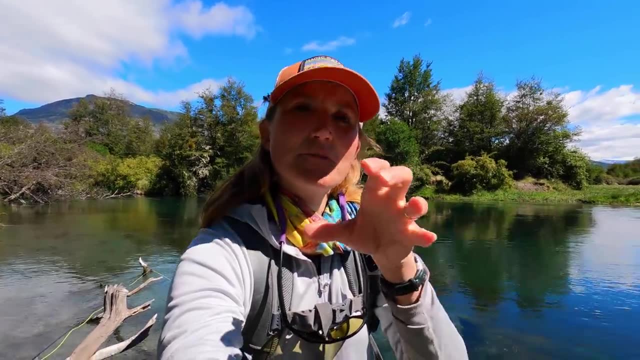 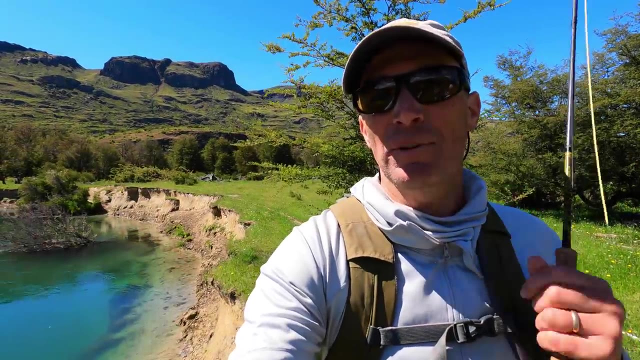 that fish was wedged in there and I just had to keep that pressure and slowly, more pressure, more pressure, as he's, as he's wiggling, then releasing, letting me give more pressure, and eventually he came out, okay, guys. so I got a same pair of fish that Amelia had to go at a skinny post spawn kind. 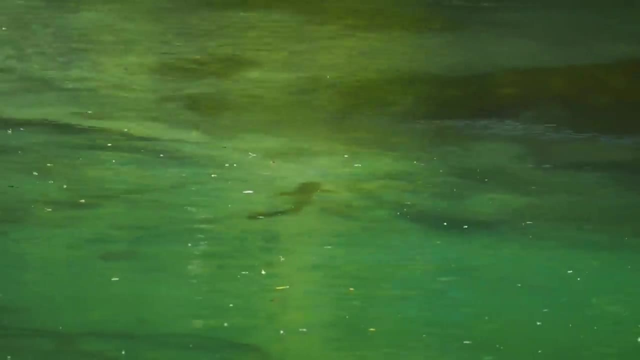 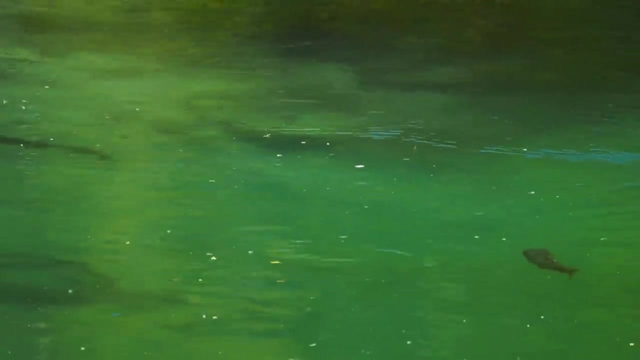 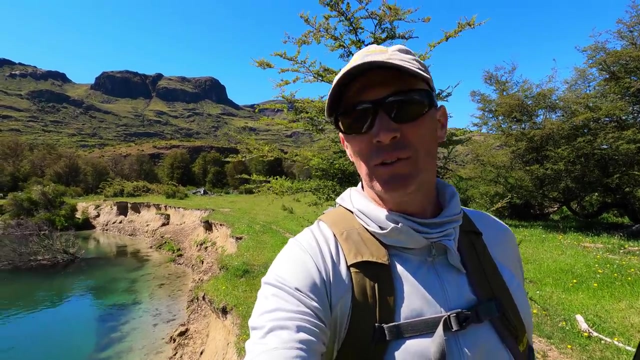 of hurting rainbow on the shore and a chunkier, shorter brown trout looks like a female brown trout out in the seam. neither one of them's doing a thing. so this is this is fun, but I'm gonna go at it with 15 foot leader. 3x, I think. no, it's 4x to a double-legged. I call it all blacks, it's just a. 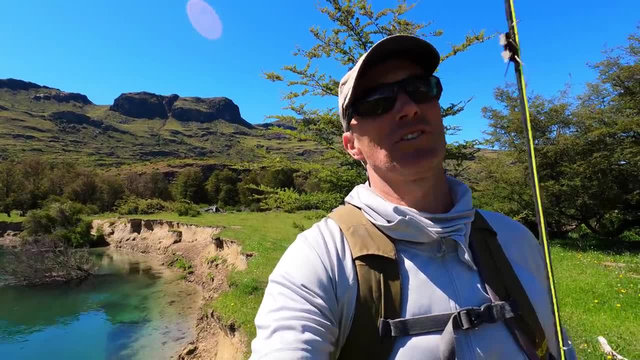 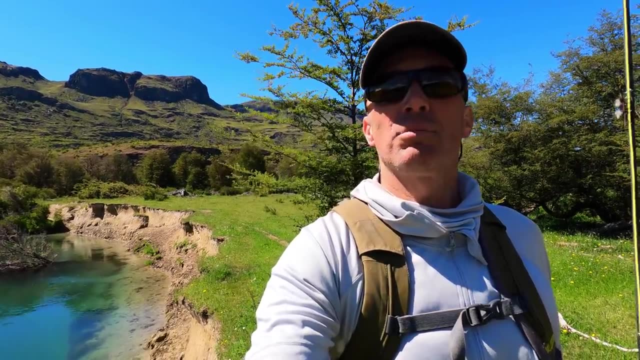 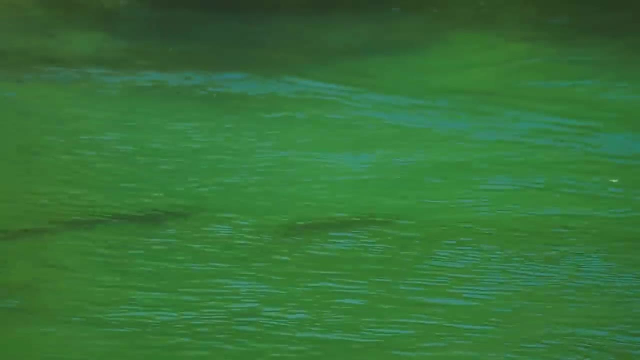 black foam pattern with lots of legs and crystal chenille underneath it. nothing special. I'm gonna try that. it might not work. it might work, we'll see. but the problem up the shoreline here is that the rain- oh there it comes out charging out. you wouldn't see this on this camera. but, Amelia, get the gh5. 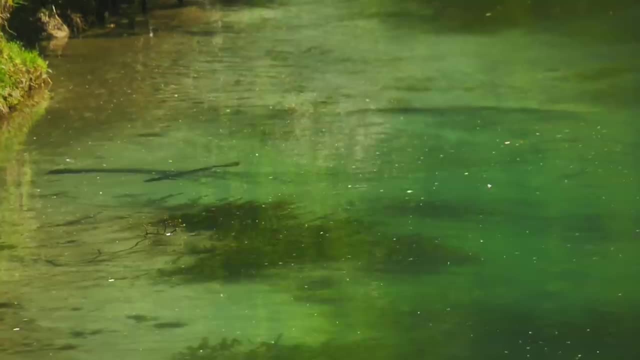 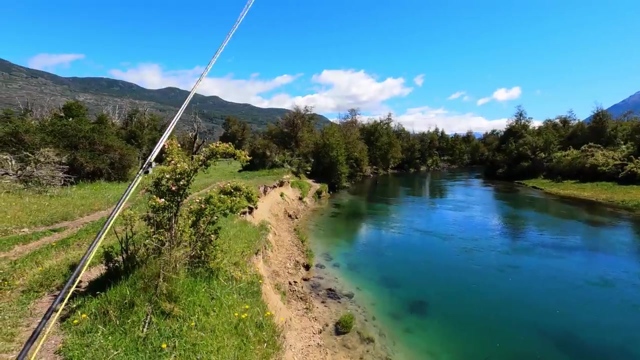 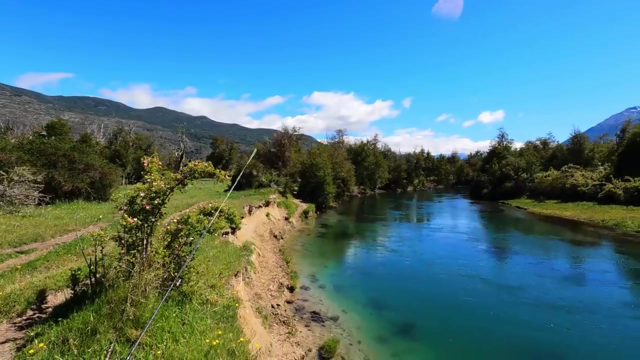 going. the rainbow is facing us, along the bank facing us, and the brown is just in the seam, a rod length out and facing the other direction. so two fish doing two totally different things, and now I don't see the the brown. of course, why? why would I expect anything less? but oh, no there. 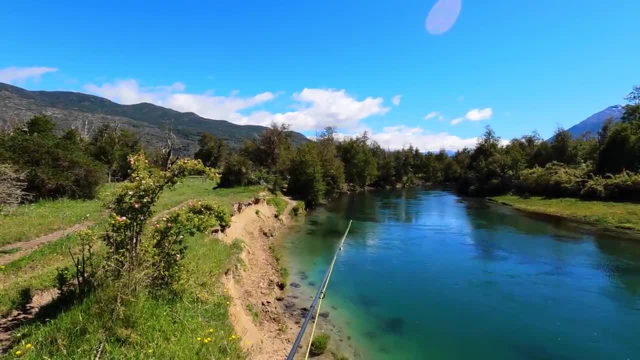 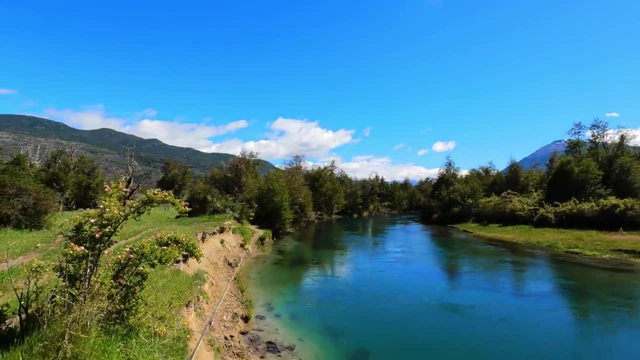 it's right by that rose petal there. so it's. it looks like it's about three feet down. it might spook too, though with the, with the angle of the sun, I might end up flashing it, but might pooch both of them by getting spooking this guy into that one again, which is never good. 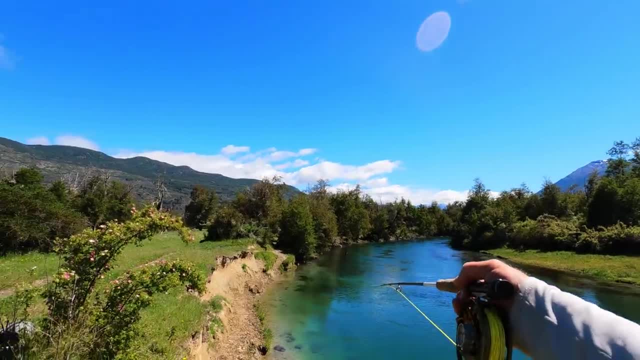 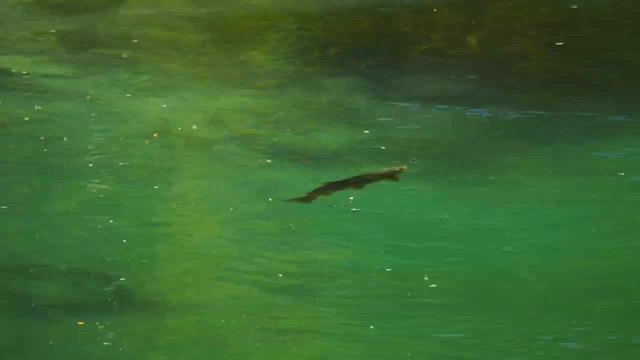 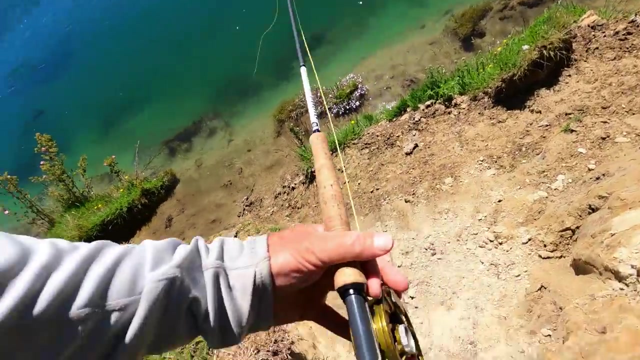 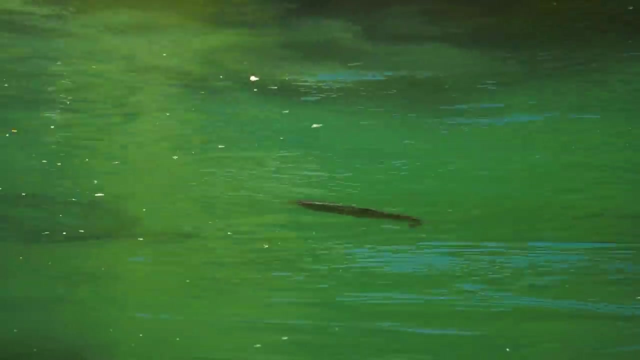 but that's a high probability. see that this one dropped quite a ways. oh, he's right here behind this weed bed up to the right. see, he's dropping those. so he's, he's right here now. anyway, get me into position here. the one that was up is really surfing. yeah, I see that I'm. I'm not going. 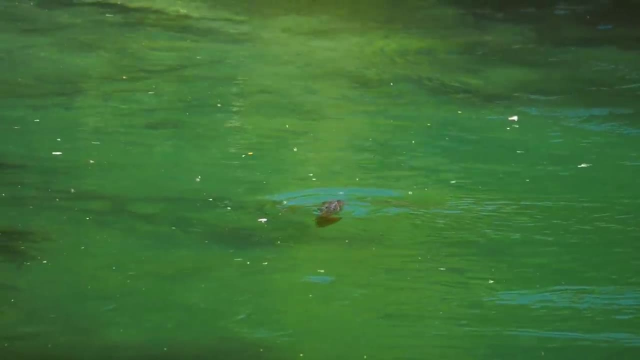 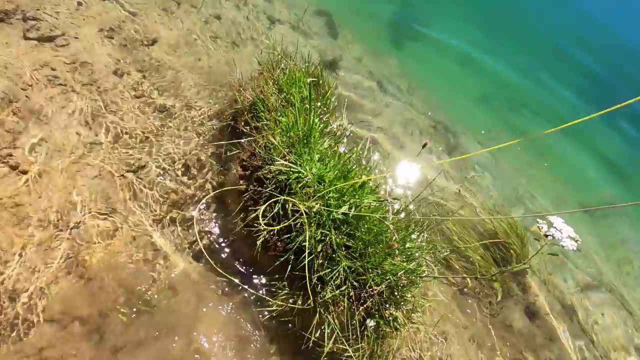 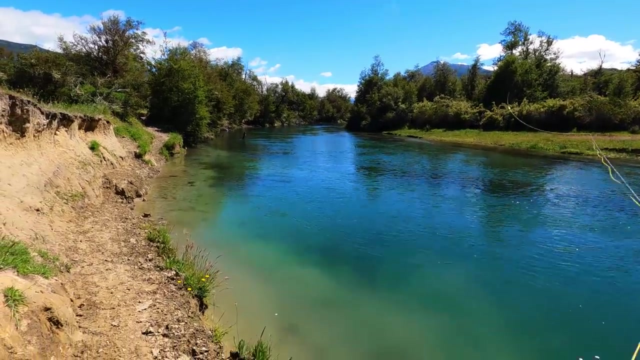 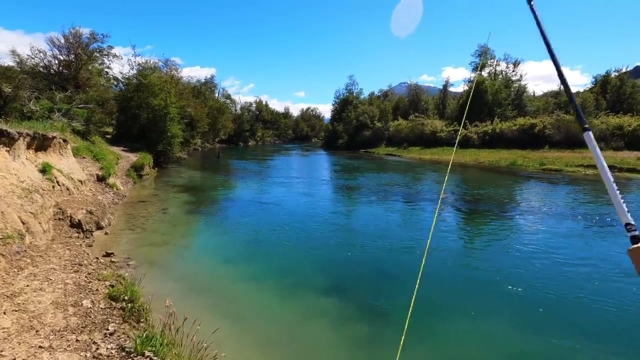 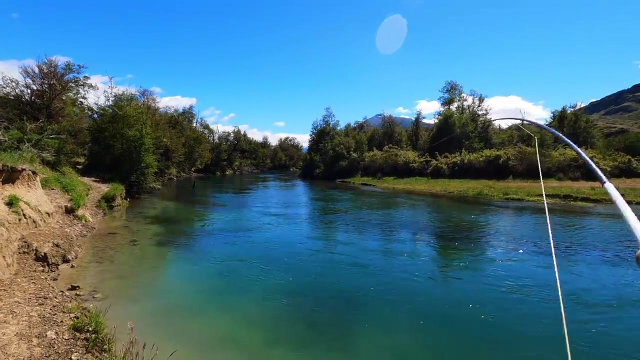 while the wind's up either. I see it way up top. it's cycled down already once, so I'm just gonna actually gonna wait back here. okay, now we wait. this is the game. okay, I'm gonna go slightly to the left, hopefully, and that was slightly to the left. 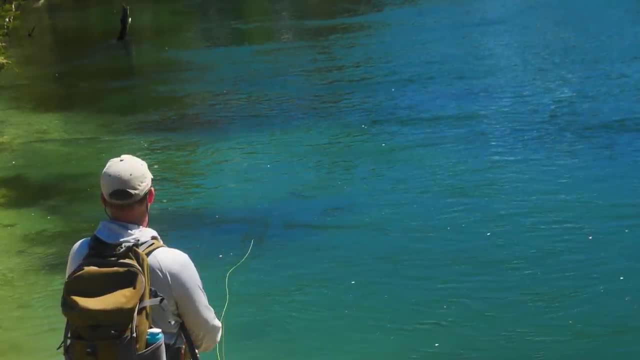 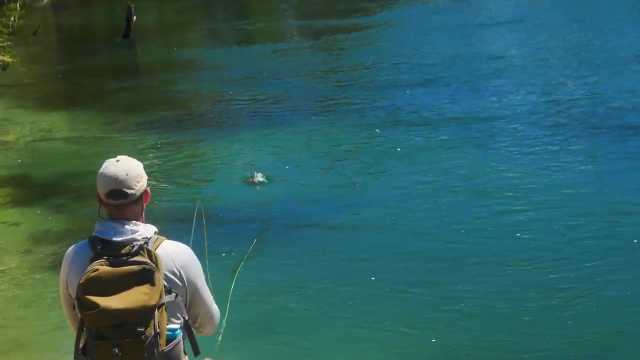 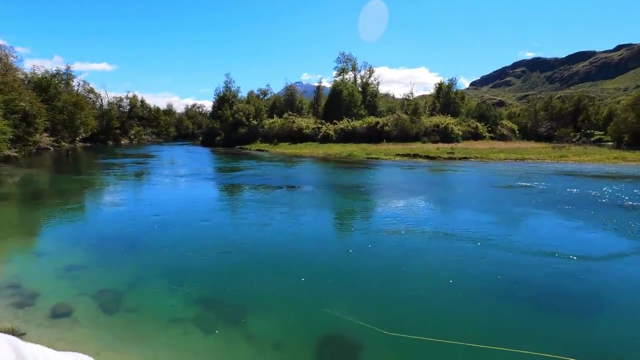 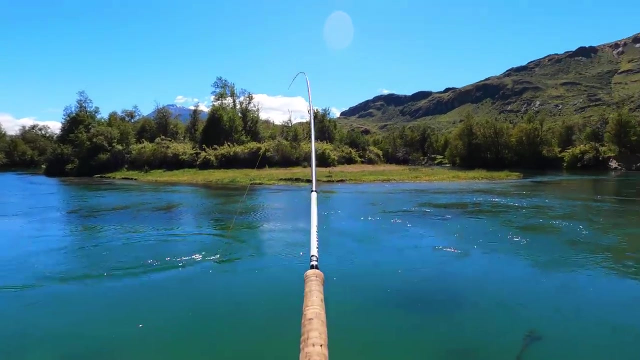 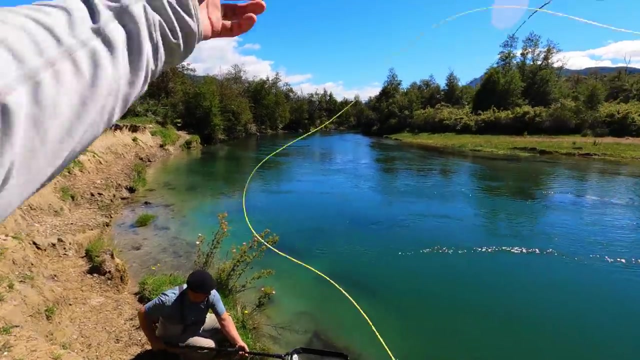 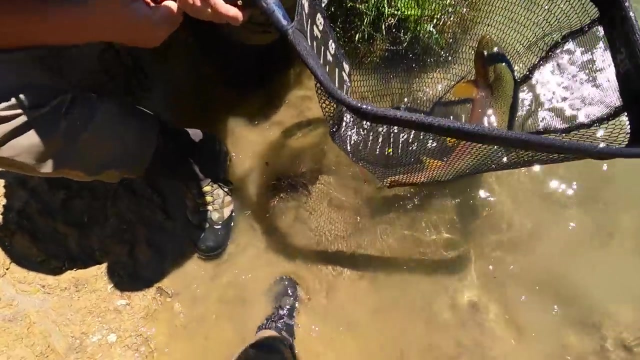 yeah, yeah, waiting for the fold right? no, no, you don't. you may as well do that. that was amazing. come on, here's the pull right into the net, right into the net, right into the net, just like that. good job, hey, awesome, what a fish. eh, gorgeous fish, nice and heavy fat ready. okay, here we go. 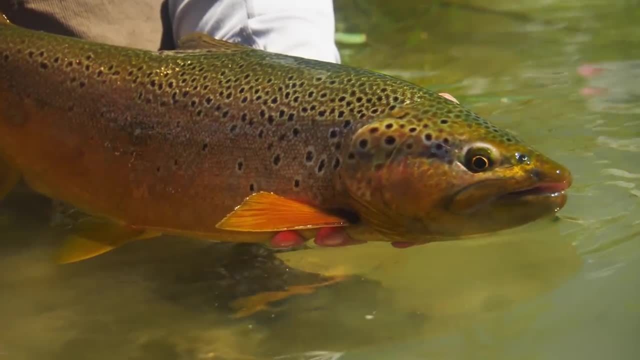 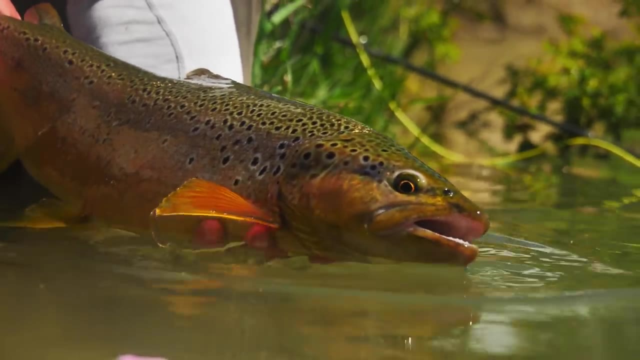 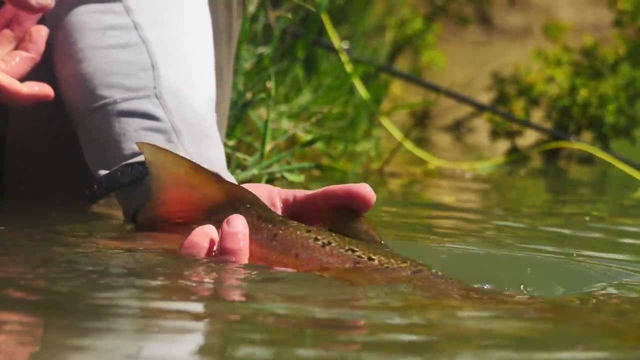 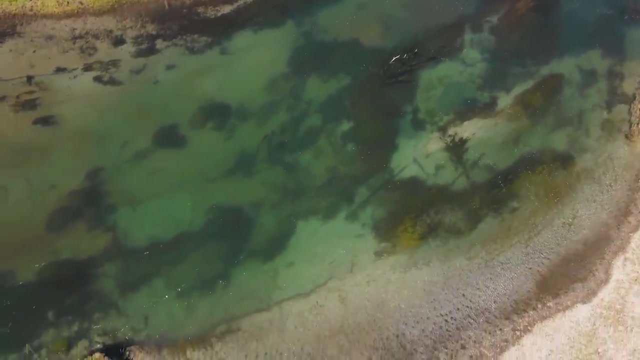 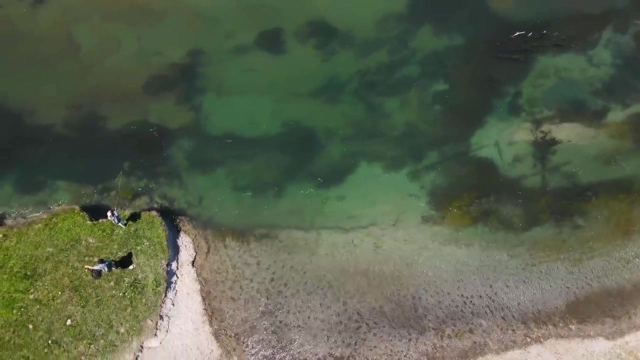 wicked gorgeous fish say, when you're blue, five, four, three, two, get ready. okay, I'll go down and up again and here we go: love awesome, gorgeous fish, wow. so. so we were just standing here, guys, and I was about to prospect and I looked out and there 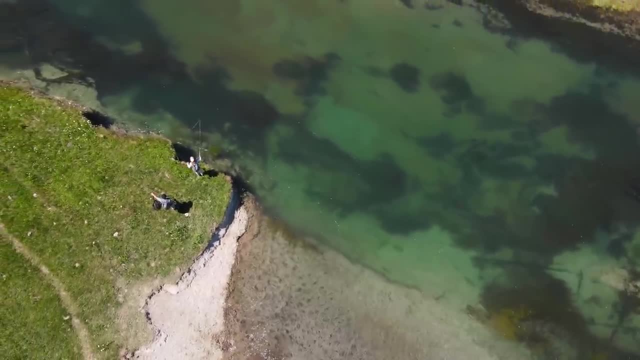 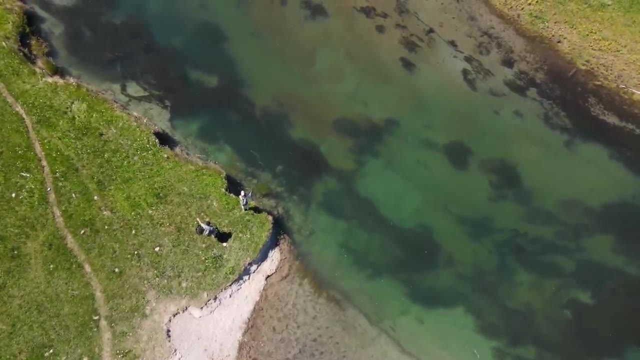 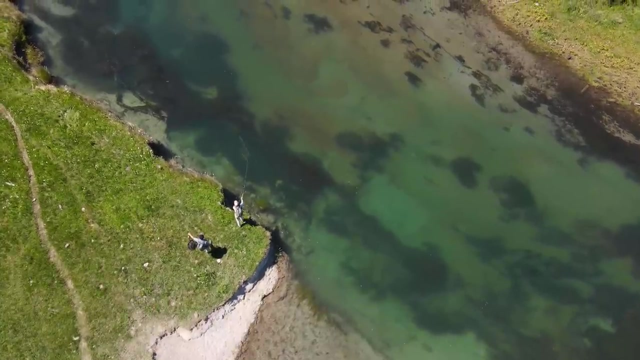 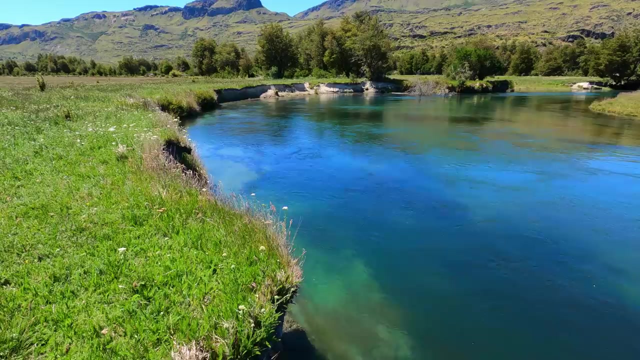 is a fish it's holding just in an exposed pocket between the weeds. so I am gonna give it a go here with my smaller beetle pattern and see if I can get him to come take. so here we go. oh, they didn't want to budge. maybe it's not sure looks so good. oh okay, so he wanted. 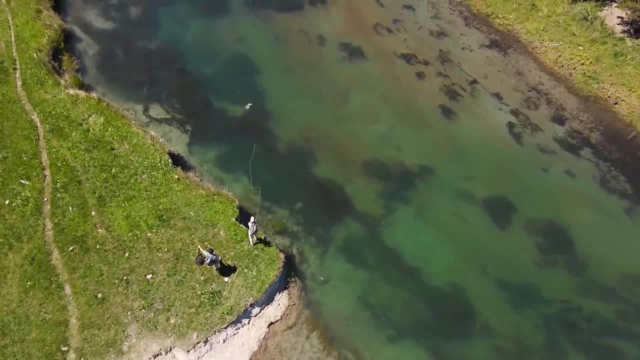 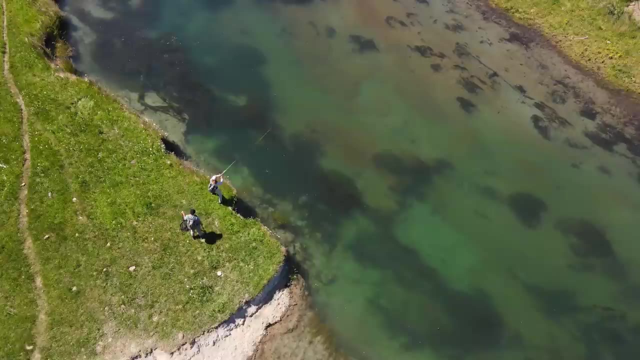 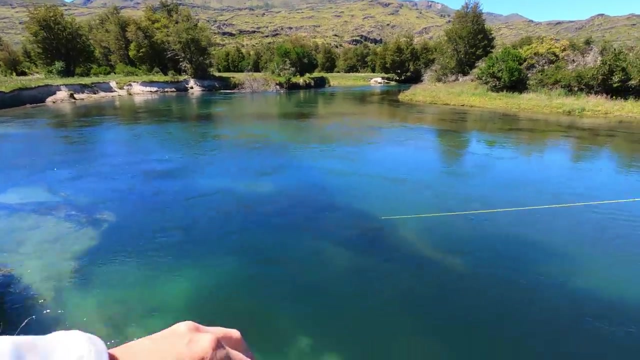 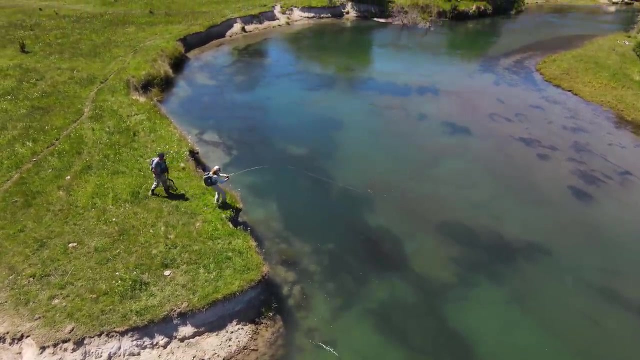 to budge to his right. he exploded on that guys, absolutely exploded on that fly. wow, wow, wow, okay, come on, fish, will I get him out of these weeds? we're gonna find out. come on, come on out. you come out, you come out, you come. oh, there we go free, free, free, free, free, free. yeah, man, right on nice. 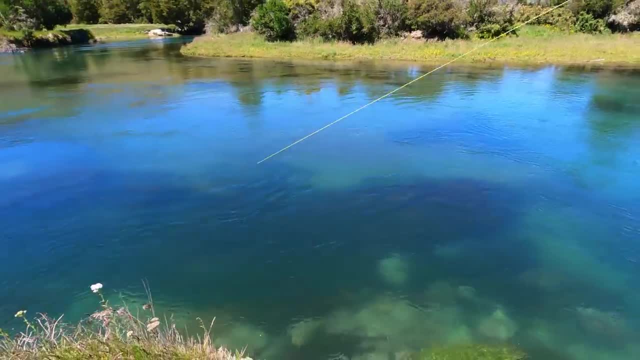 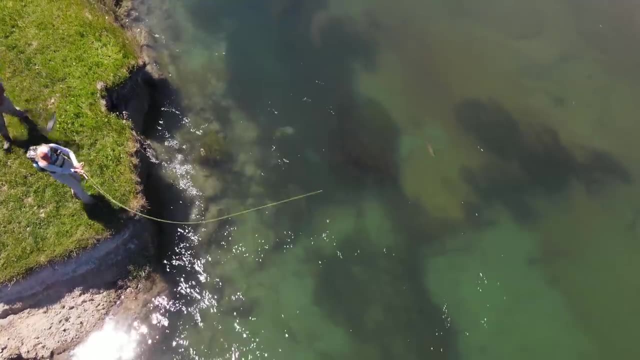 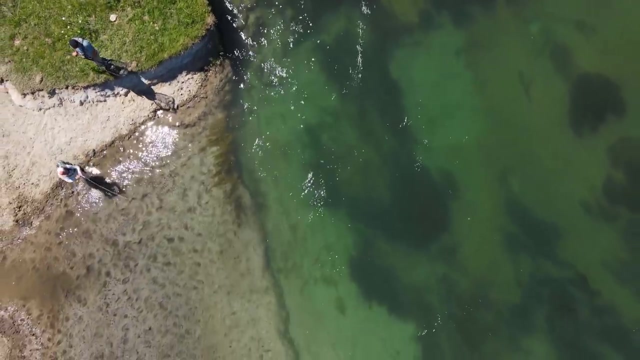 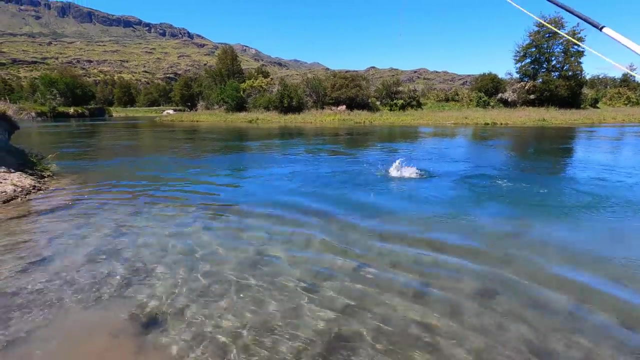 brownie, whoo-hoo, haha, come on, back it up, back it up, like they do in New Zealand. back it up, come on. yeah, we'll swing them around here. yeah, yeah, that should work, perfect. yeah, oh, I need the net. just he's not huge, but that's yeah. oh yeah, right on, haha. oh yeah, he's a. 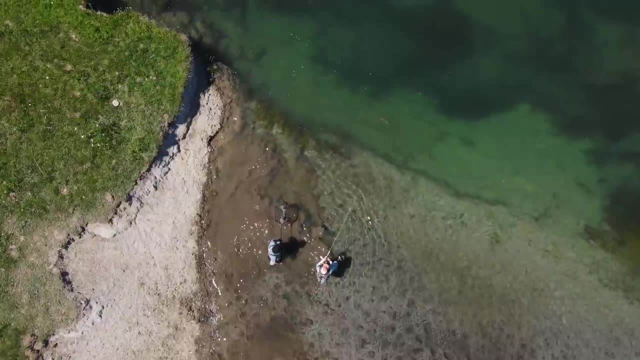 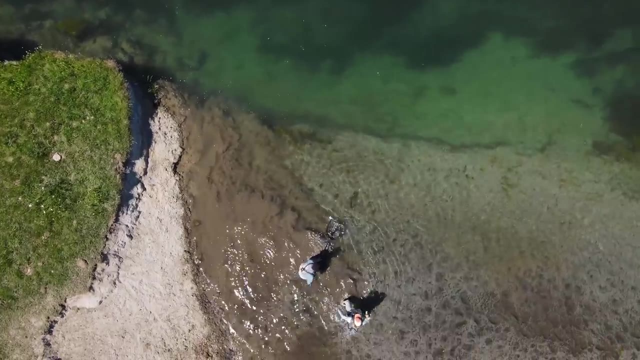 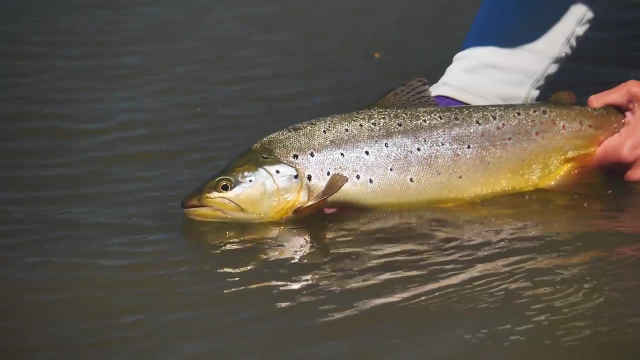 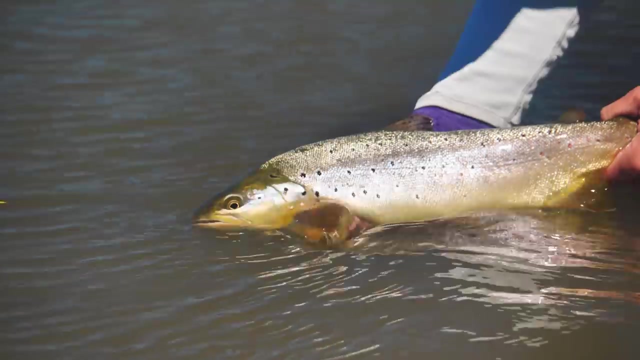 jumper. all right, isn't that cool. all about where he wanted the fly to be. that's neat. and in the net. yeah man, sweet man, awesome, love it. so that was neat. both Marcella and I here were looking for that fish because there had to be one kind of in the zone and it was just a small pocket like maybe I don't know. 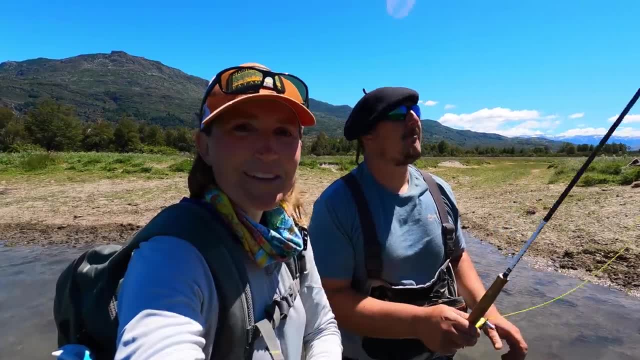 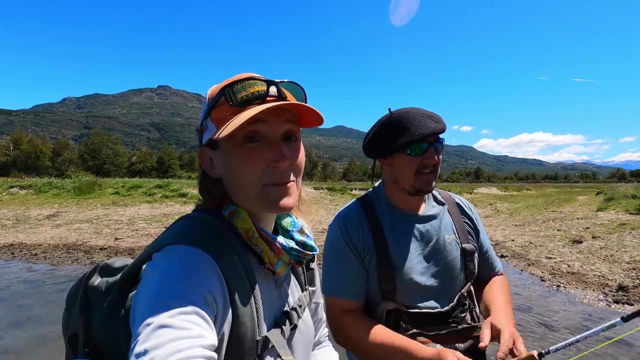 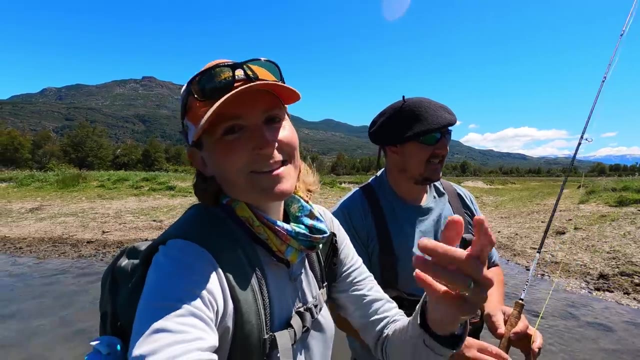 a couple feet by a couple feet wide, uh, in between the weeds, and I looked out there and at first I thought, okay, is that just a weed? right, it kind of looked almost like just a weed itself. but oh, no, no. then it moved, just enough to say, no, that's a fish. and we confirmed: yeah, it's a fish. and 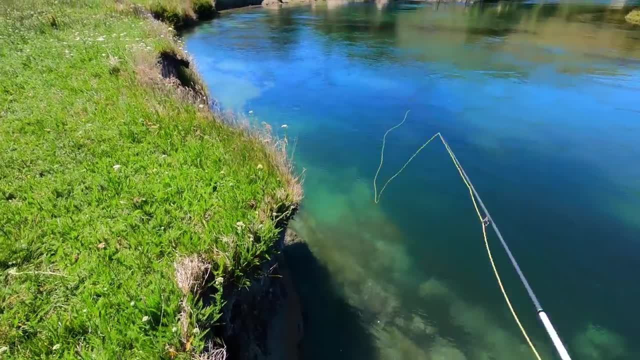 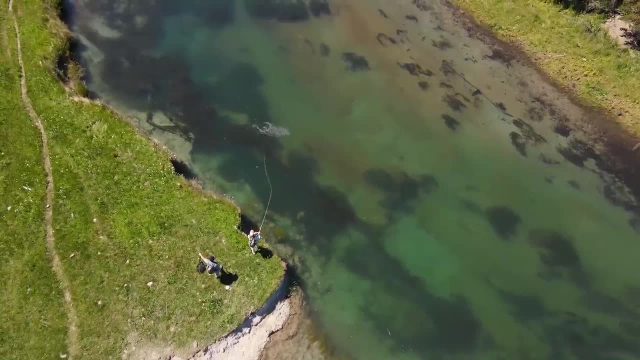 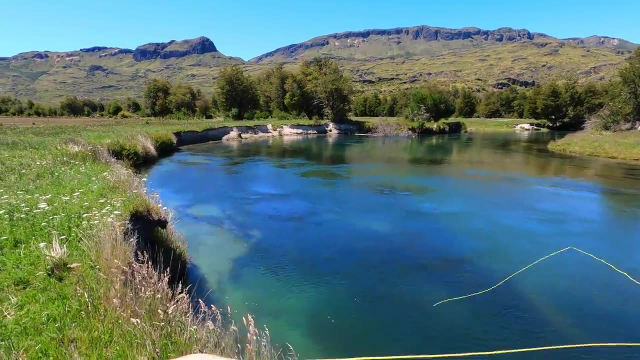 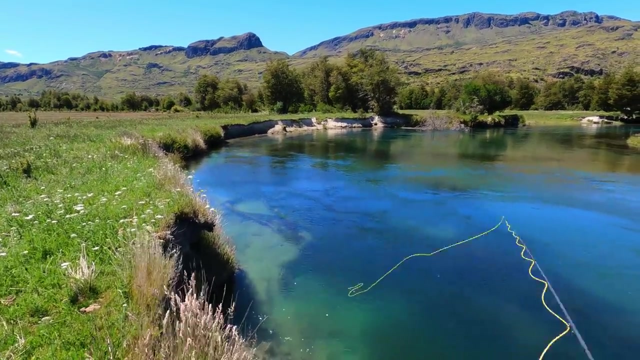 hey, put the beetle out there and wow that that take was awesome. hey, oh yeah, exploded, it exploded. yeah, yeah, lots of fun, all right, guys. well, now I am gonna cross back the water with a slightly bigger beetle, um, and just see what comes. what else might be hanging out in these weeds? I want to get a cast. 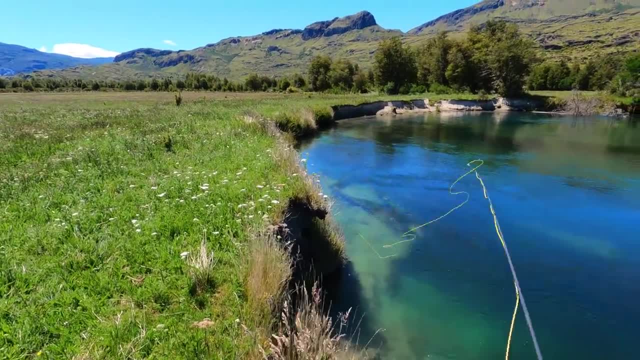 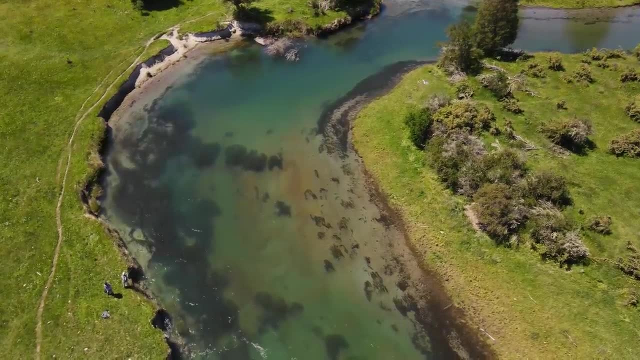 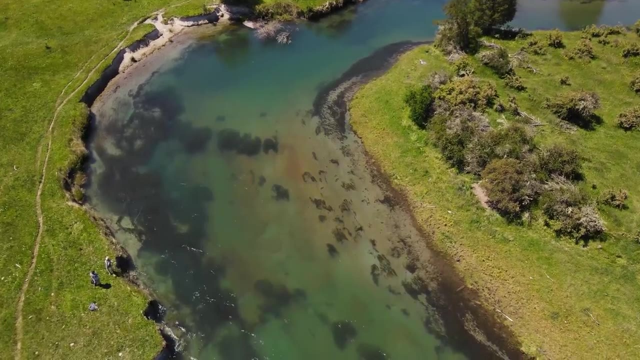 that's right up a little tighter to this whole bank. see if anyone's holding tight to the bank gonna play these weeds right off the end of it. no, okay, then I'm going to do a cast further out right off of those weeds. no, okay, a couple steps forward. 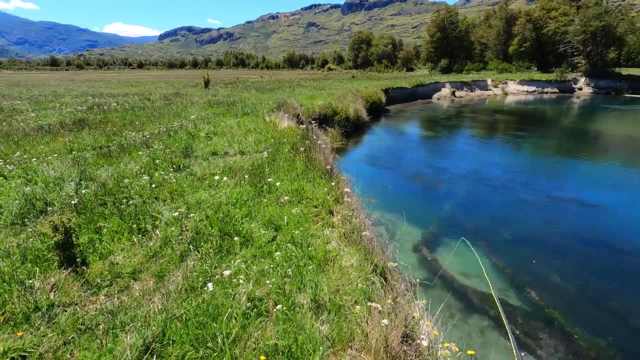 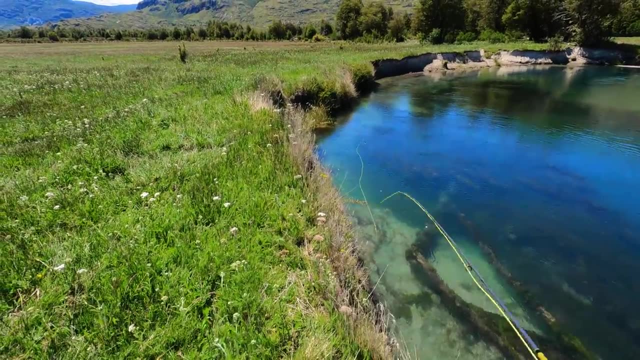 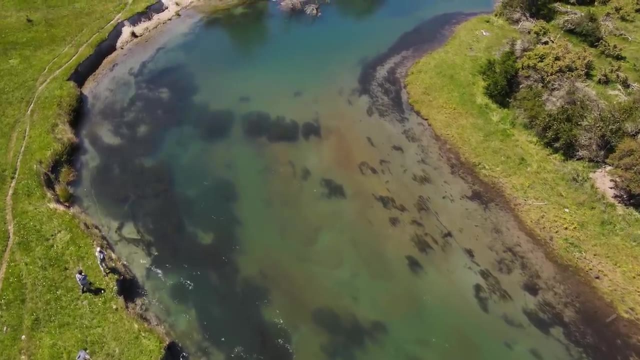 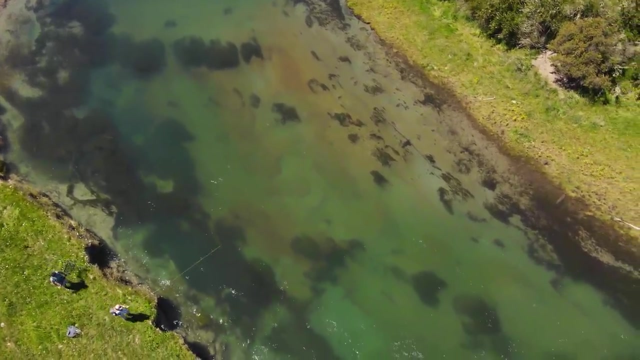 and right in here. great spot if anyone is tucked in and wants to come flying out from that bank. oh yeah, oh yes, oh, what a take, what a gorgeous take again, man, that's fun, that's fun. come on, let's bring you down, not a big fish, but a fun take, really fun take. 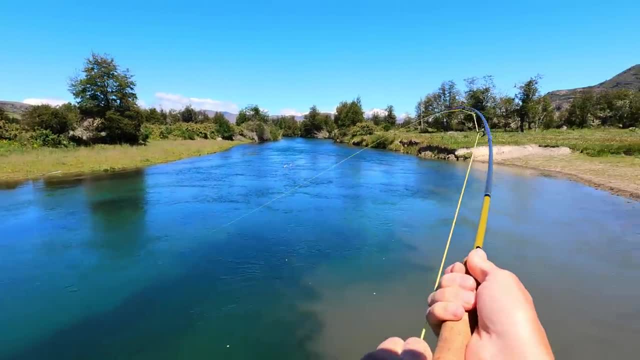 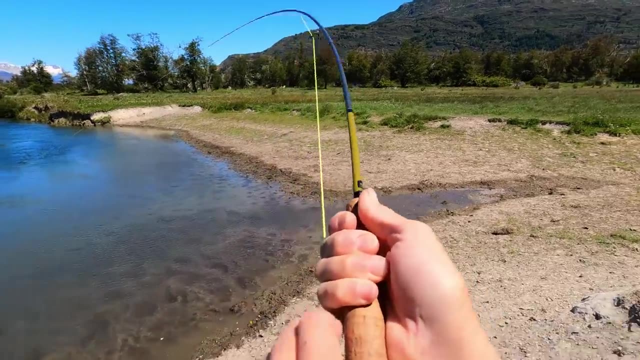 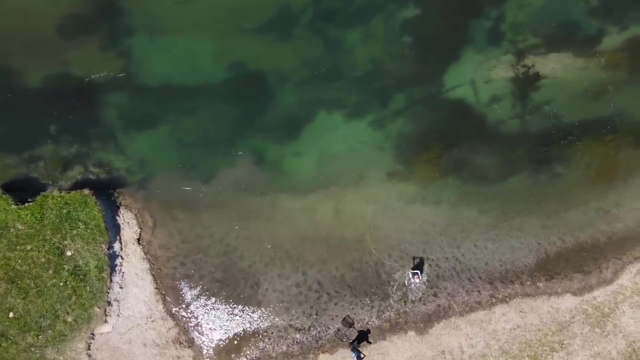 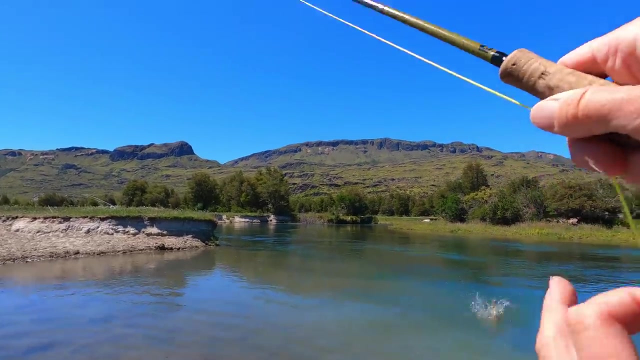 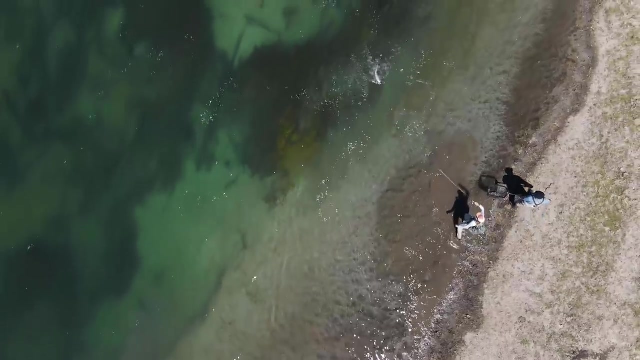 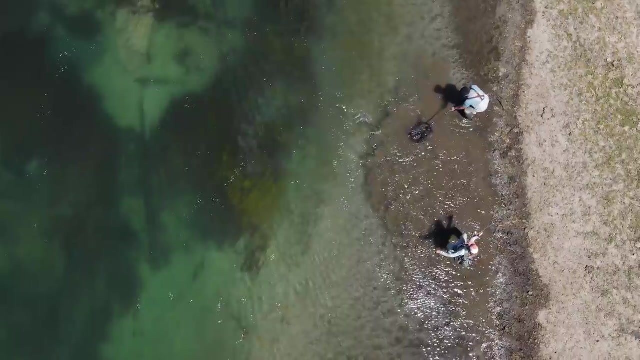 still a good fish, just not a. it's not a massive one until he starts fighting me way downstream. come on, try to surf him in. come on. these jumps right in front of us are just perfect. here we go. it is beautiful, go for it. no, try to pop it in you. there you go, nice. 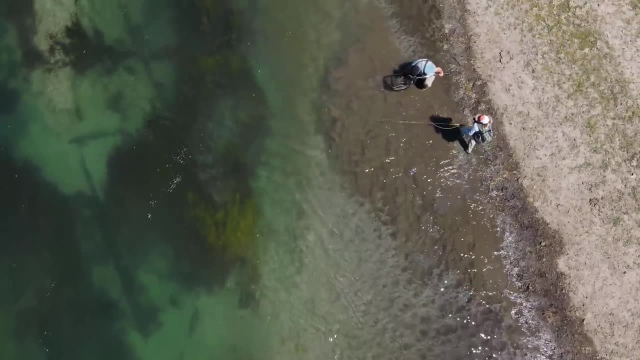 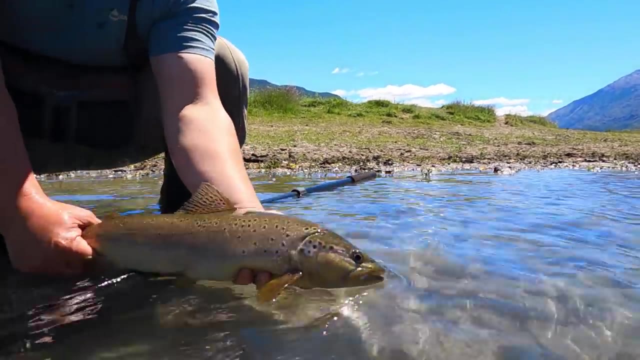 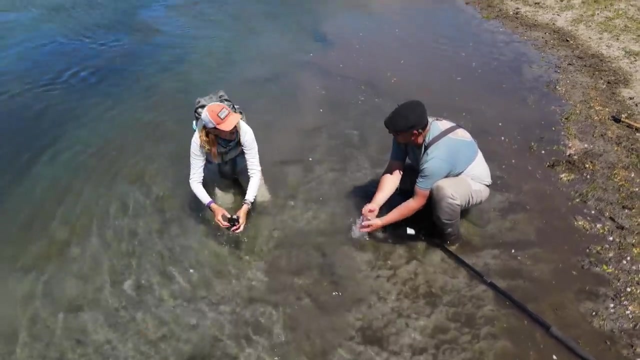 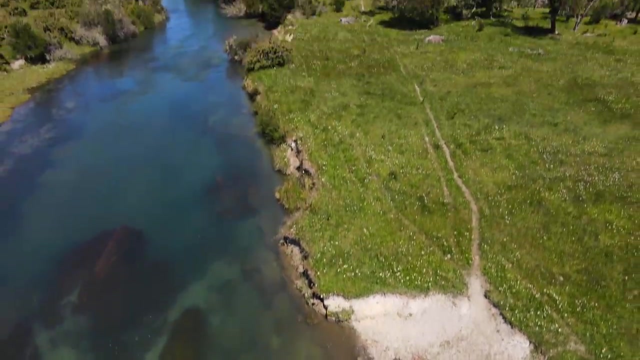 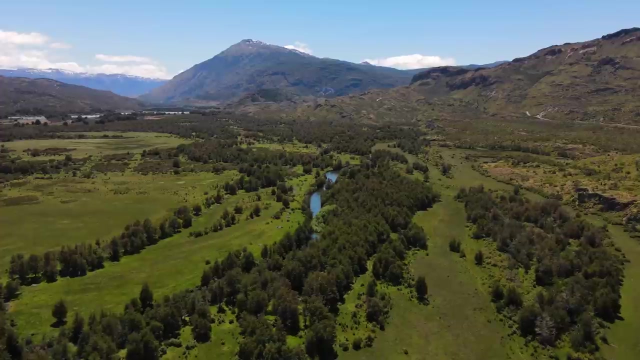 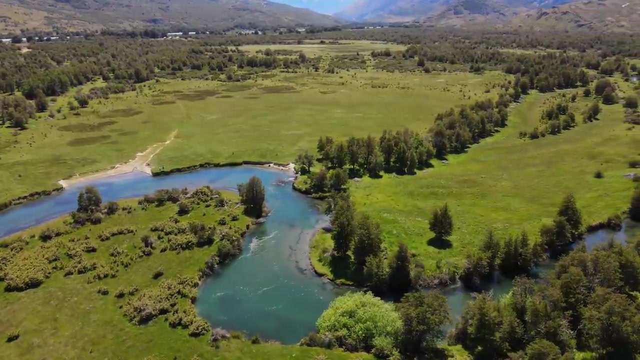 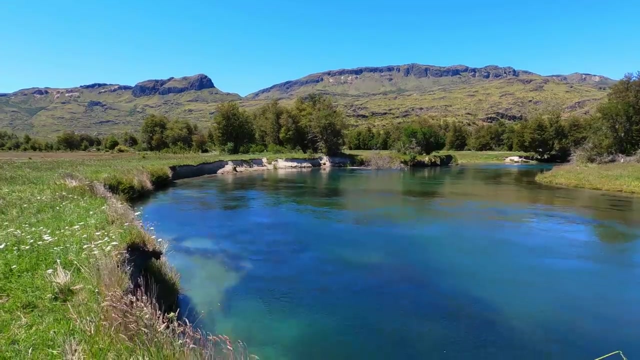 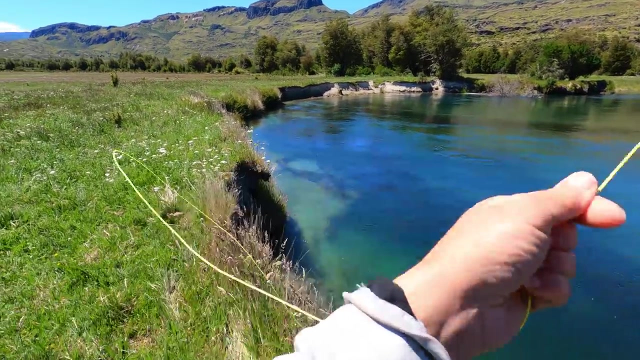 sweet man, really beautiful fish. hey, oh yeah, no, it's longer, it's longer than the last one. hey, we good, perfect. yeah, above the water, nice and slowly down. yeah, man, it's perfect, yep, anytime. so that was really enjoyable, guys, that fish came, that last fish came right off the bank. 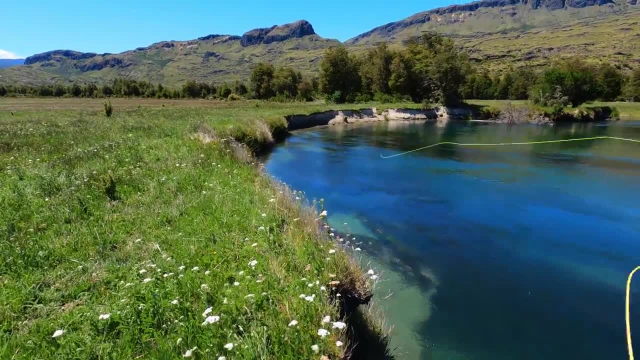 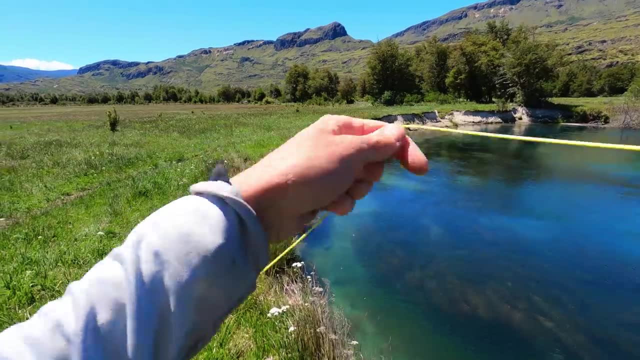 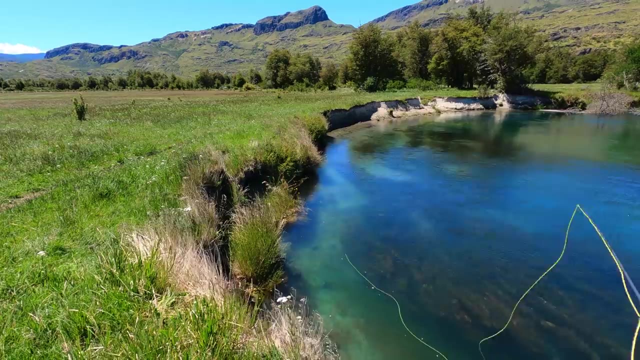 right up ahead here in tight and just look like the perfect spot to get a cast, so I won't refish that water. okay, now I got to get one again tight into this shoreline. no, not into the grasses. Oh, let it drop off. twitch, twitch. I think that. 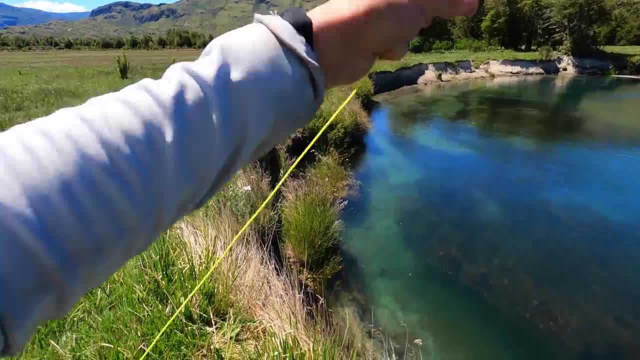 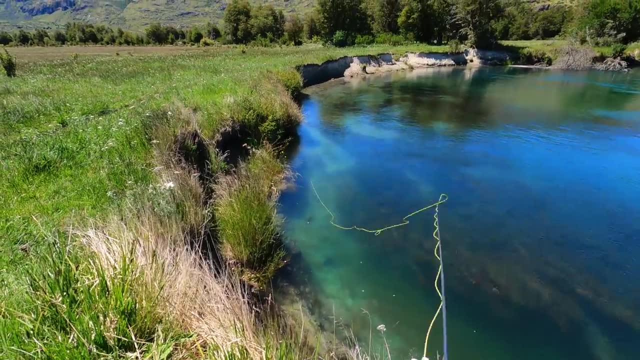 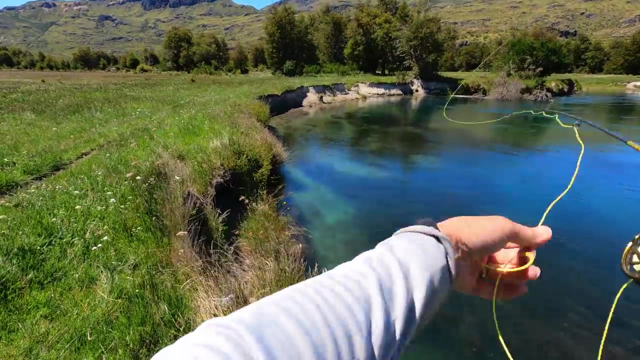 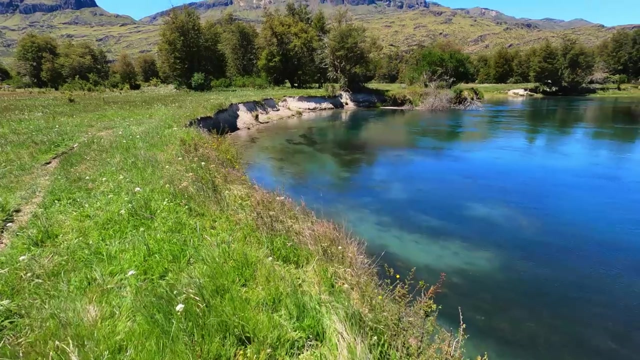 guy came from underneath those grasses right below me. but how about right in there? yes, come on fish. oh, if there is to be another fish, I think that would have been the cast. but he's not. that's cool. no, okay, in tighter now. yeah, I don't forget there was, I didn't get a shot. 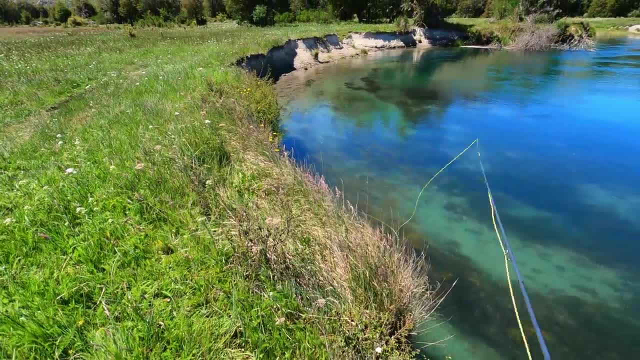 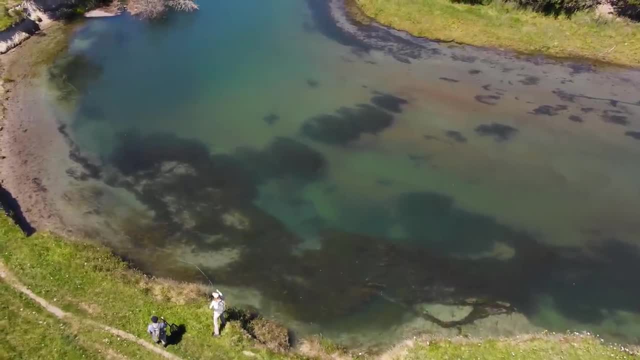 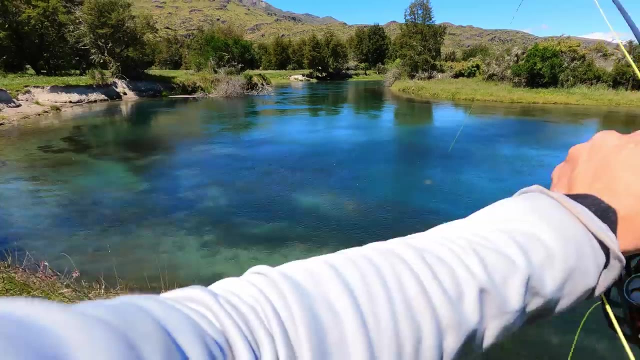 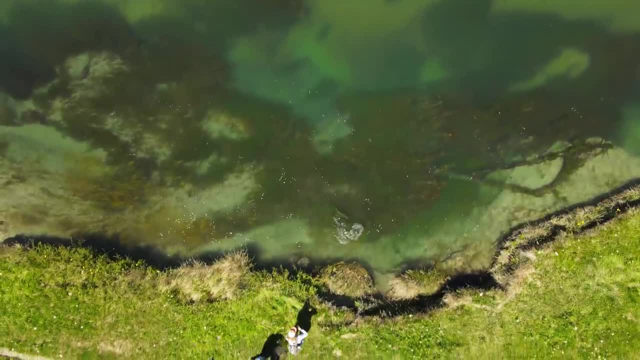 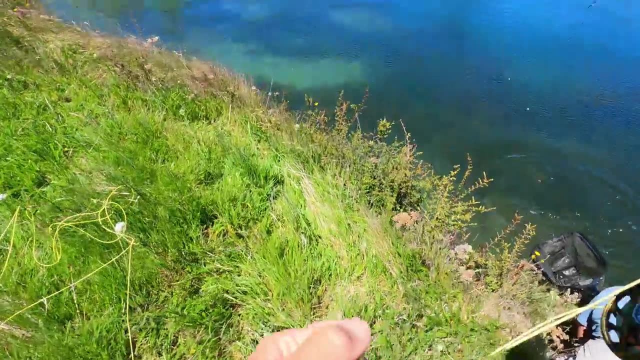 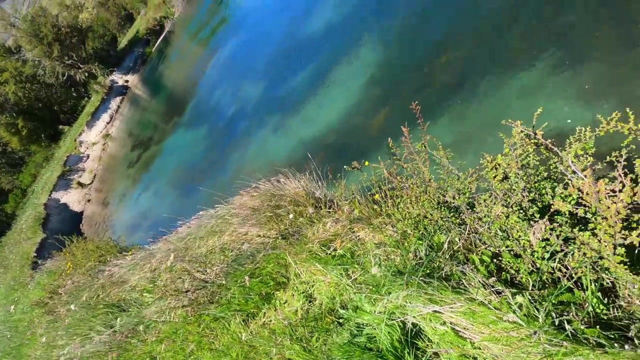 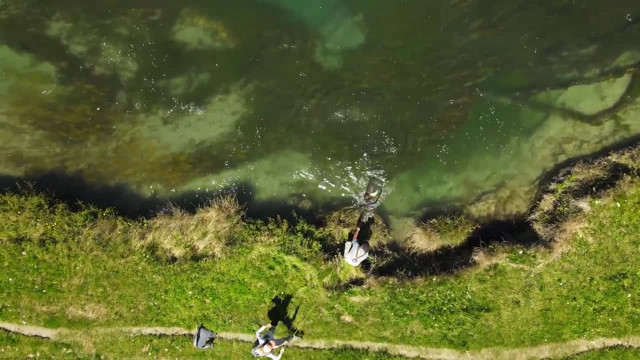 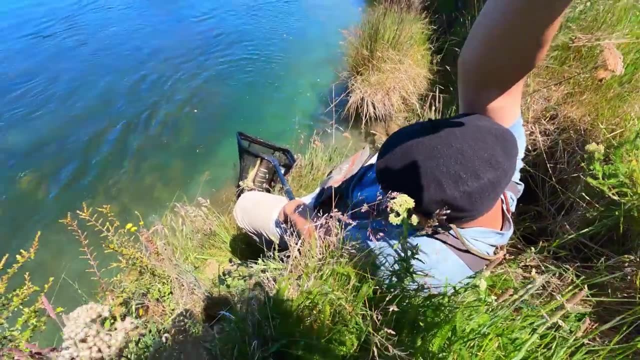 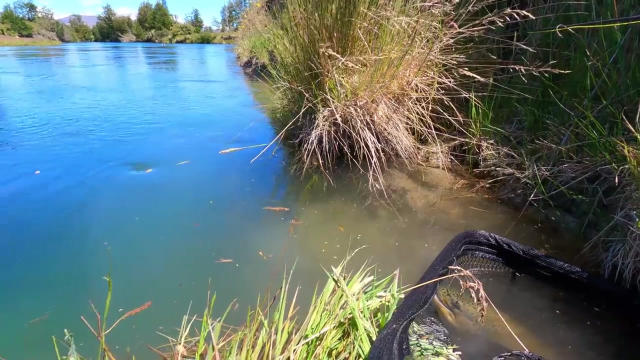 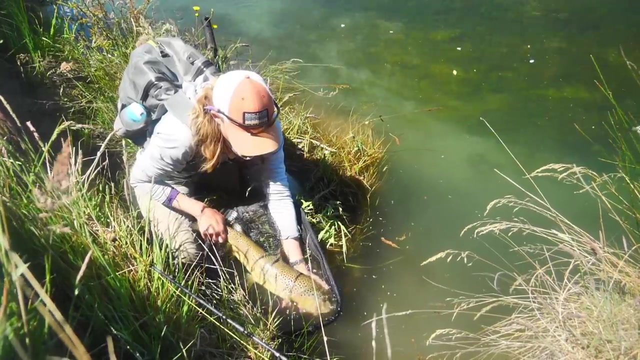 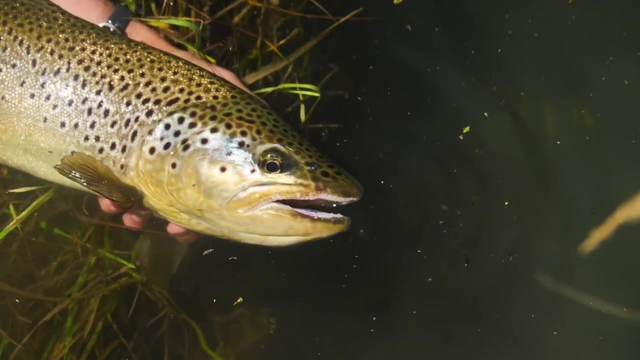 okay, I'm surfing, surfing, surfing. yeah, thank you, it's really nice. hell, yes, oh, what a fish, awesome. all right, so we get ready to let this guy go. oh, it's a really nice fish, hey, just yeah, where he came out of was so incredible. yeah, right tight to the bank had to get that beetle right along it. 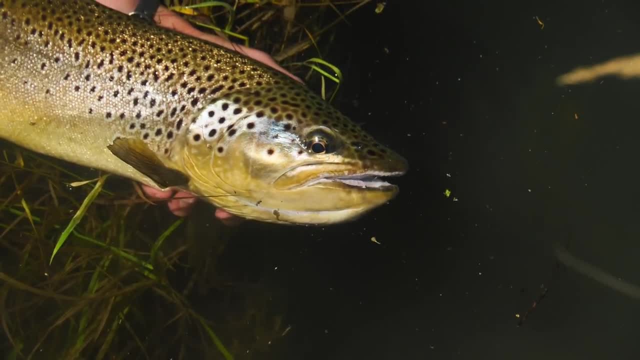 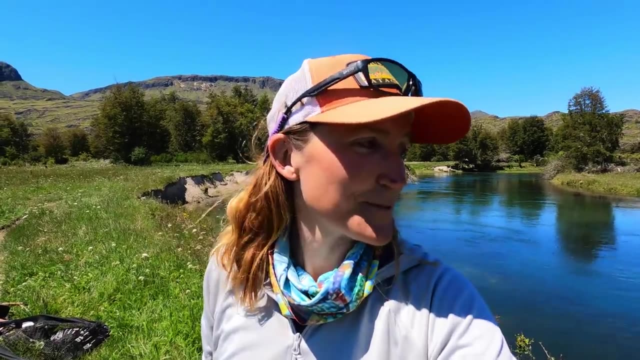 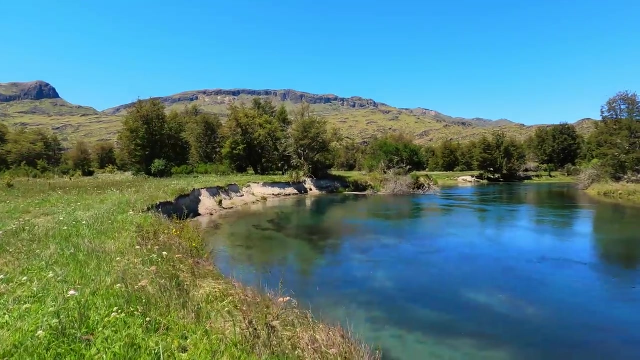 and man. haha, that's what I love. what a fish guys. yeah, absolutely loved those moments and all I was doing was prospecting. this river is full of structure, amazing terrain, so it was just really nice. now, I have to say I really trout structure and I was standing right where I am, right here and up above me. 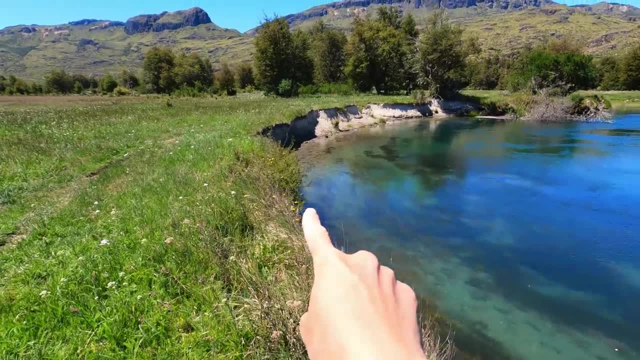 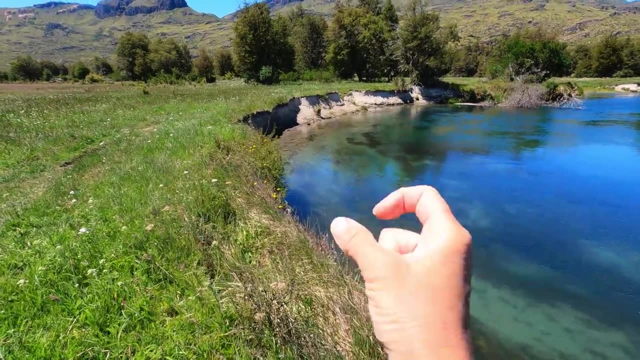 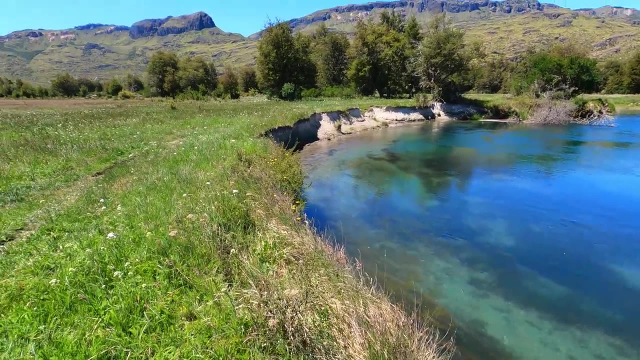 I'd say not even maybe ten yards. you can see there's a line of what they call Calafate hanging over the river and there's kind of a shadow, true shadow, right along that, and I just popped that, cast right in there as tight as I could. 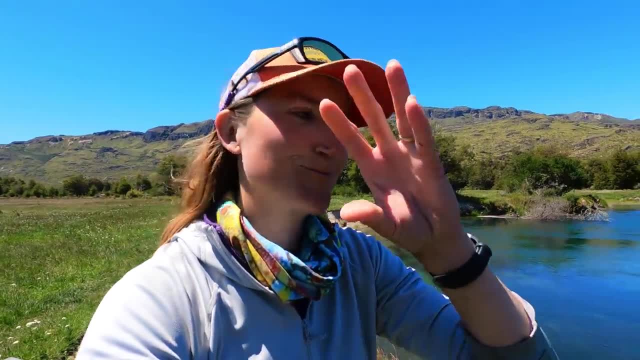 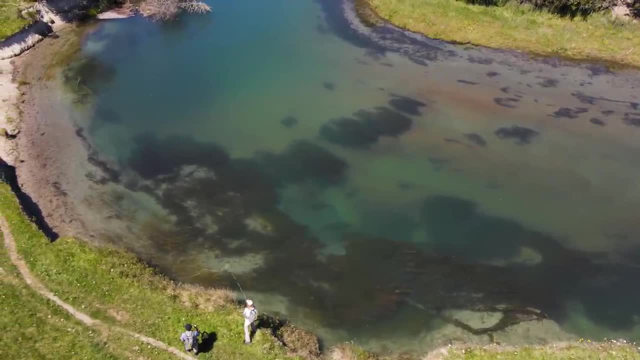 and, yeah, you just see that set of lips come out, suck it in. yeah, I knew, knew it had to be probably a big-headed male. I've seen that enough in our fly fishing career that you go: yeah man, good fish. so, yeah, lots of fun and the nice thing this: 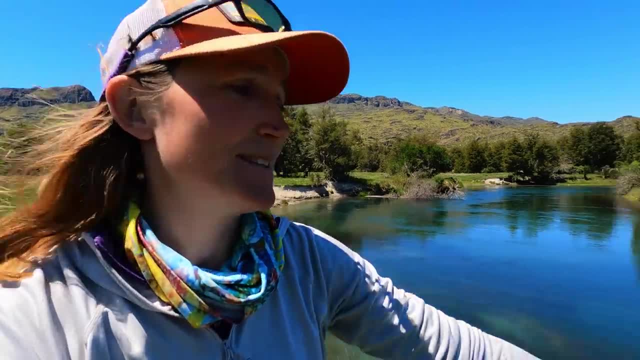 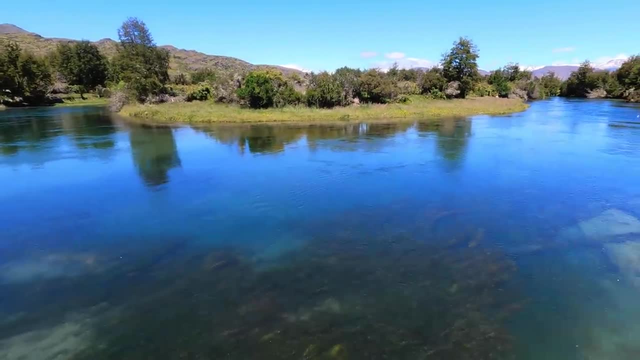 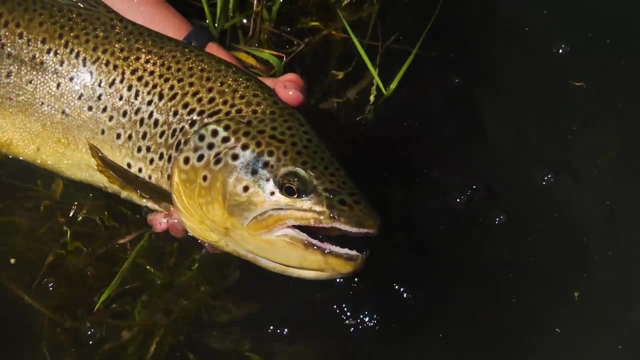 time is that he didn't want to fight me all the way down because out here lots of deeper weeds he could have gotten hung up in. but I cranked on that fish, had 3x on and then we brought him right into this little bay and Marcello did an awesome job of netting him. and hey, that's what we live. 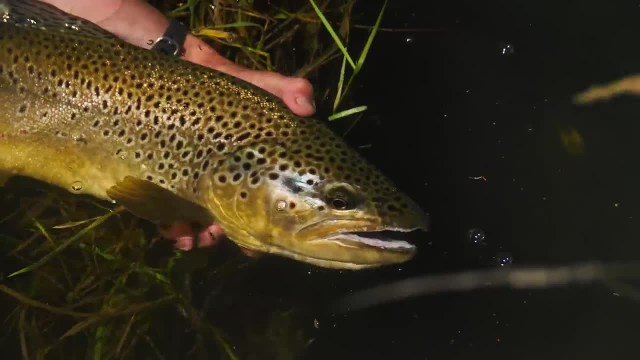 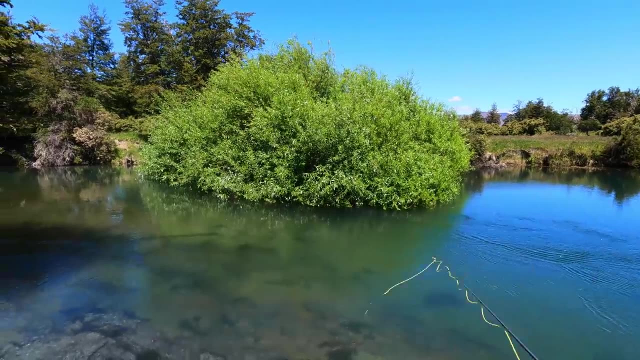 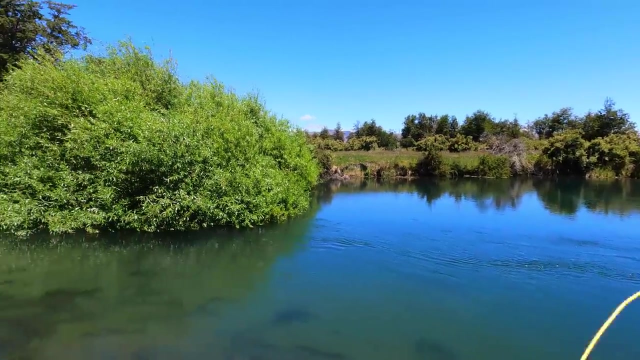 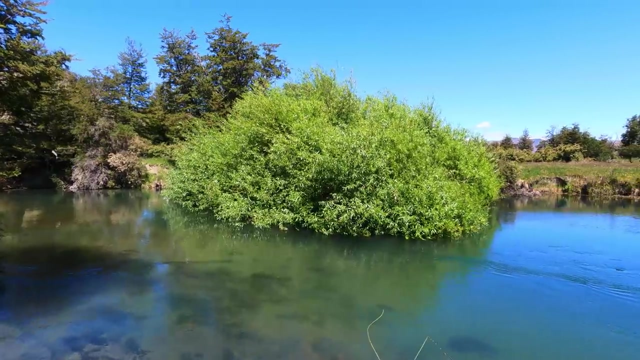 for great, great moment here in Patagonia, okie-dokie. so these guys tell me that there's a fish right on the bottom, right here, and I have to double nip it. so there he is. that's deep, fast, fast, fast, heavy enough. will he move? did not move, gotta go higher. 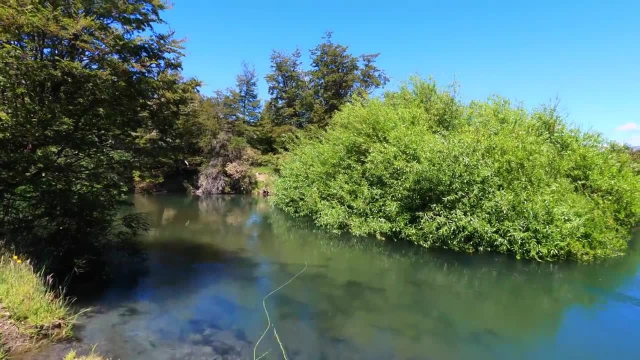 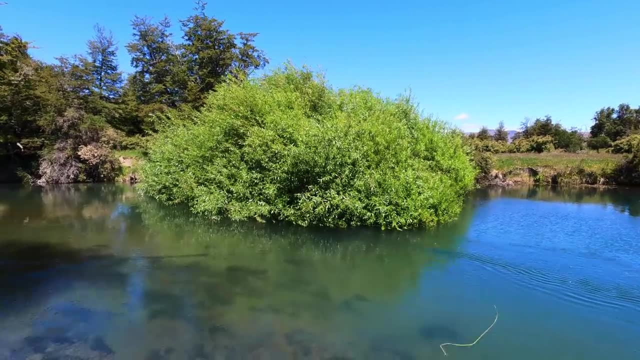 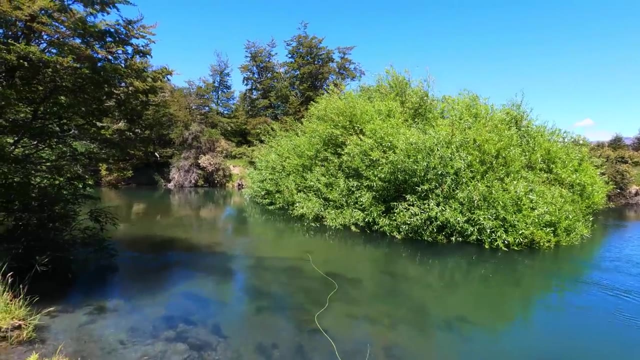 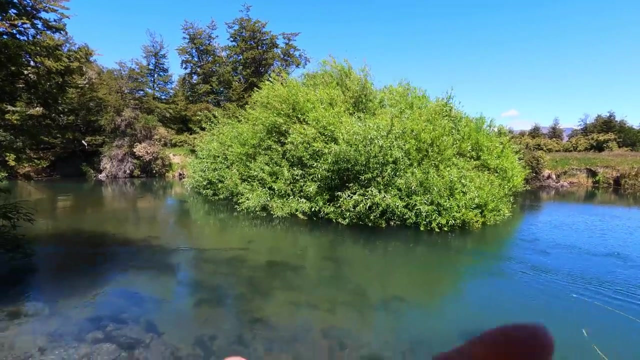 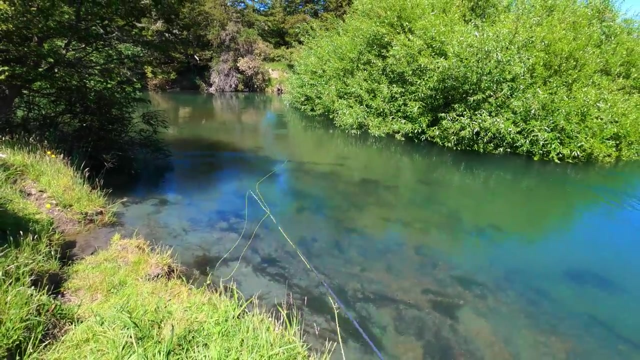 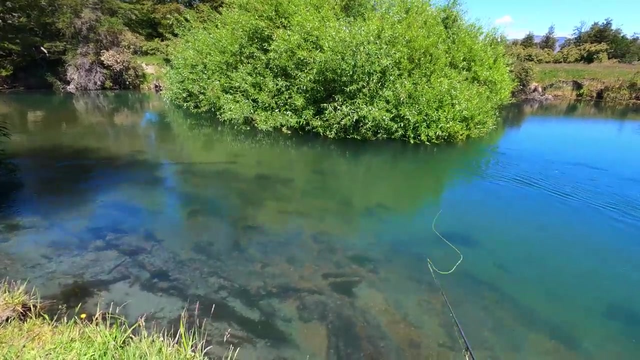 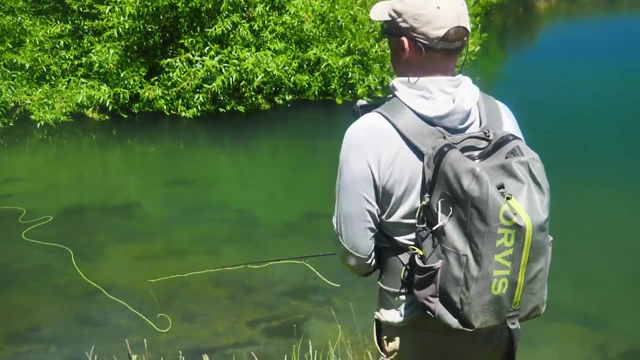 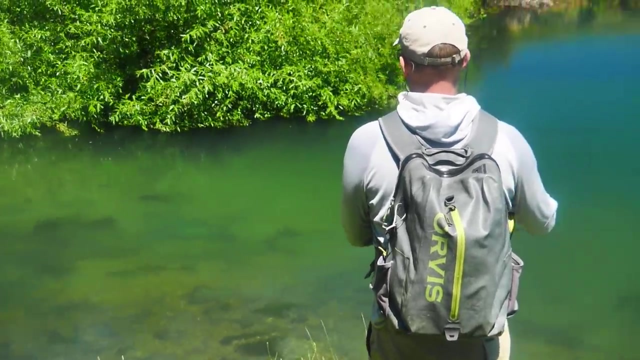 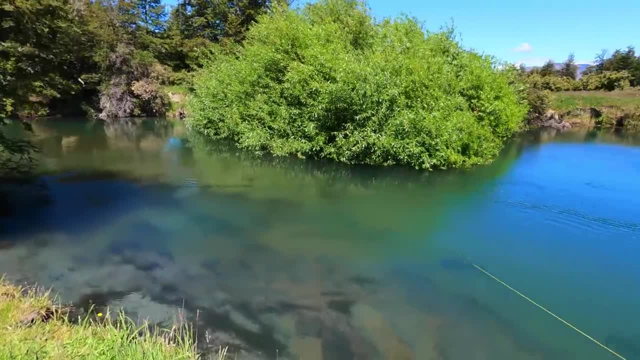 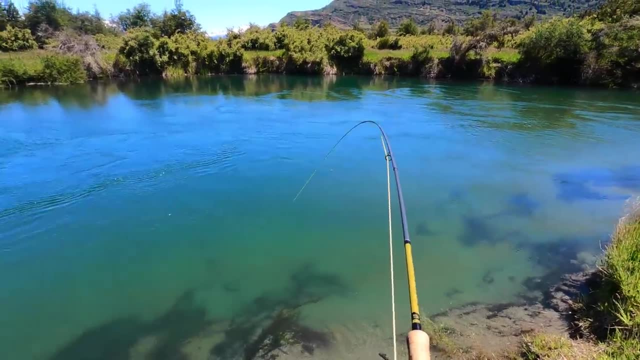 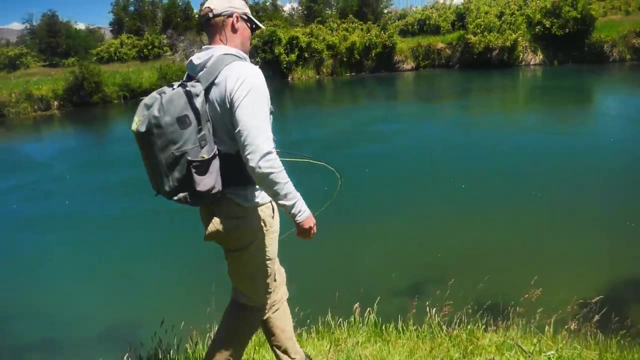 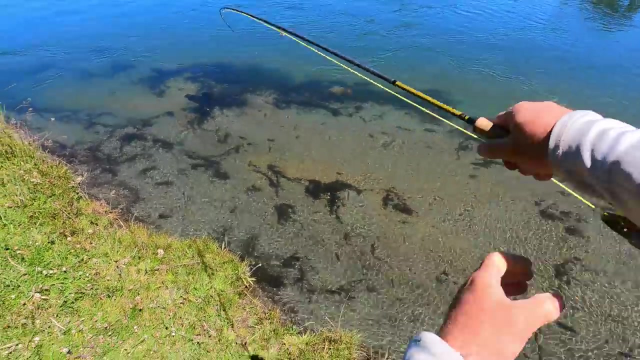 got him. he dropped hey off that shelf. whoo, I saw that head turned down and white mouth open. and here he is: big, fat, heavy thing. hey, he's gonna have. I think we're gonna have to land it down here, aren't we walk the dog a bit? yeah, really heavy fish, yeah. so I'm gonna go like this if I. 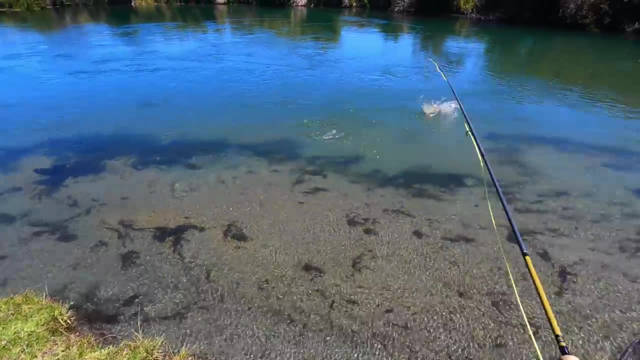 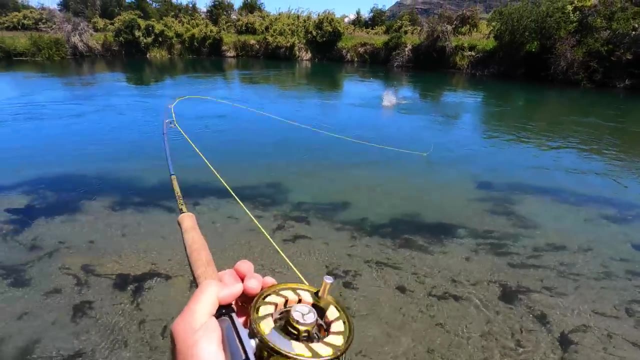 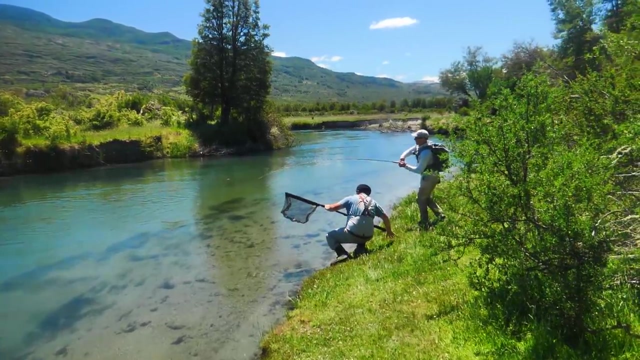 can fold her head if she'll let me there. nope, no, she doesn't want that. I'm in there. washes on now up, it's a heavy fish where we going. you're right in here. you think, okay, what I was looking at, I had. I basically had this to land the fish, if not in there, but I mean if it comes along here and 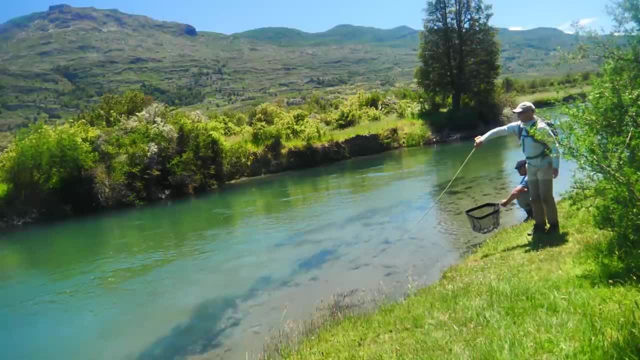 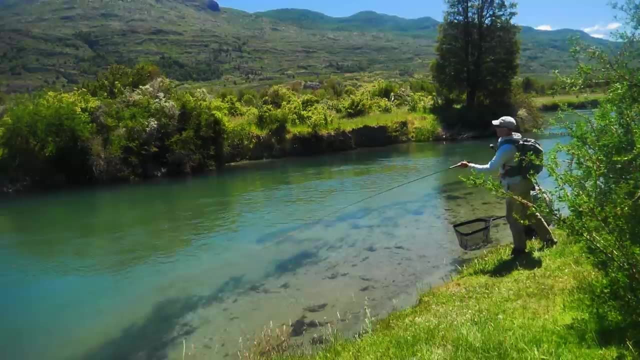 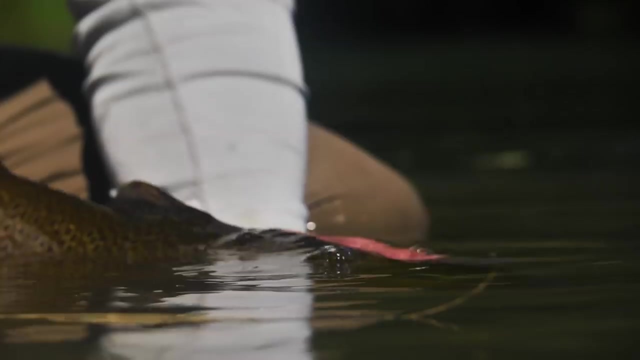 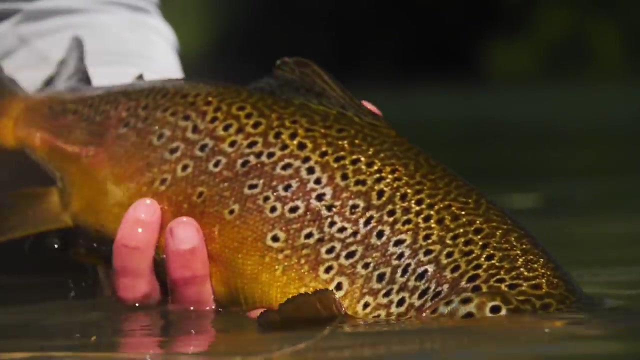 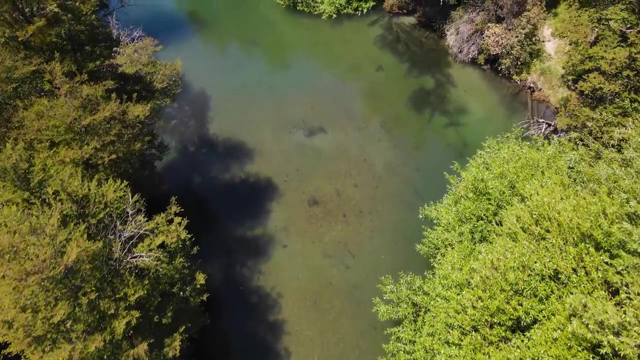 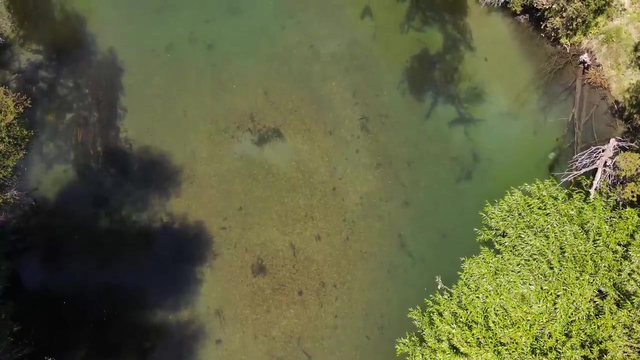 decides it doesn't want to go out there, and it wants to go out there now. I'm in that sticks over there, so I absolutely had to crank on that fish. yeah, okay, guys, my, my lovely wife has found me a gift fish and two days ago we fished this river and i got my ass. 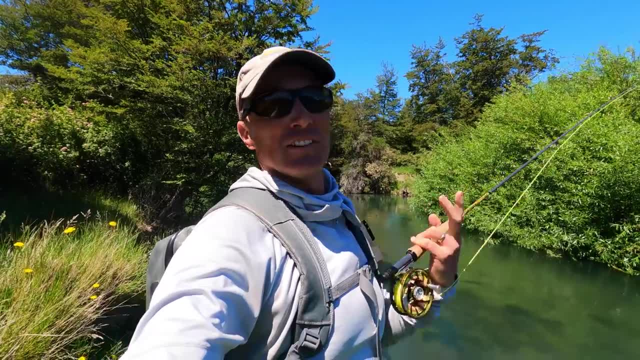 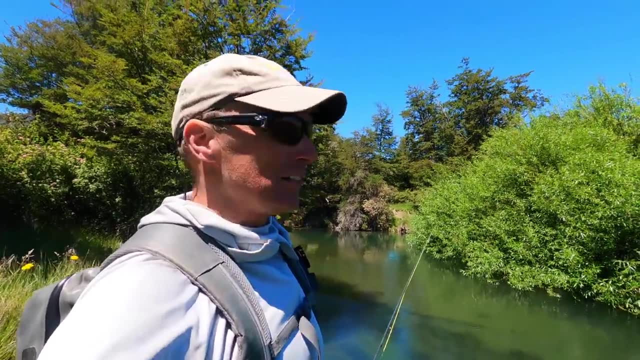 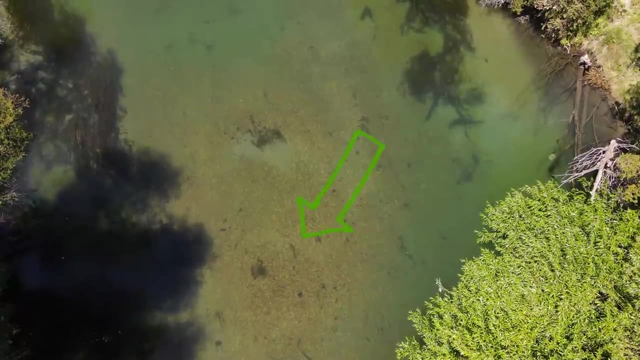 handed to me twice two casts in a row in the same exact log on fish, i don't know- 26, 28, 24, 26, whatever inches long. and now my wife has found me an exciting fish, and what i mean by that is right there in the middle in the river. there's probably 25 to 26, 27 inches sitting right there. 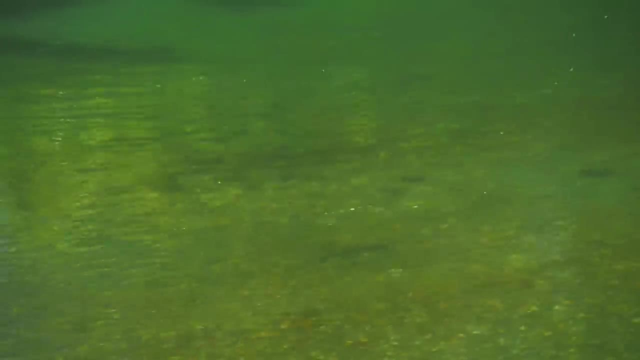 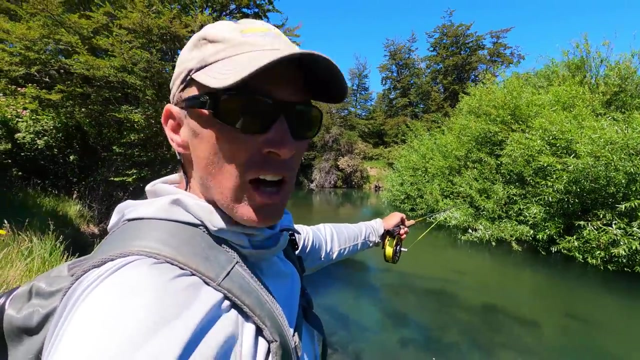 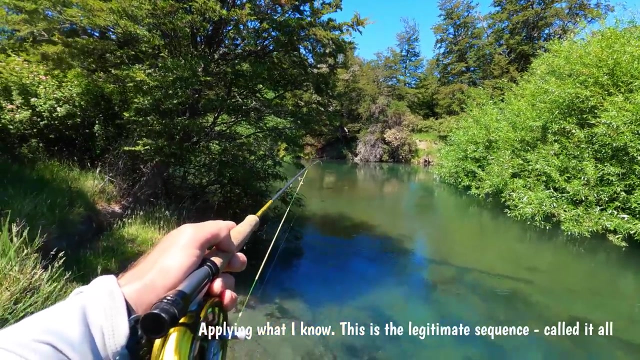 in the glowing sun, but you know what's going to happen. so we know if i, if i hook up, if, if, if, um, it's going there, there's no way in hell it's not going under the willow, um. so the only chance i have is to draw it as far left as i can with the big beetle. so i'm going to stick with this big. 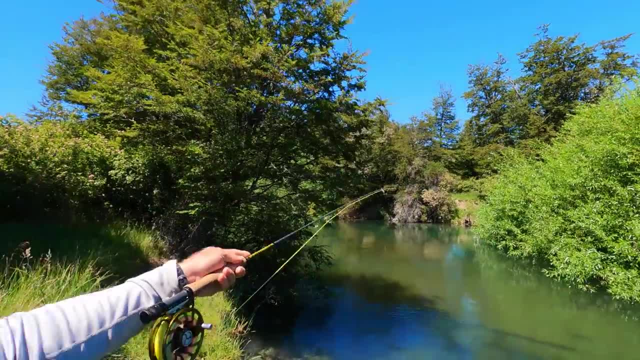 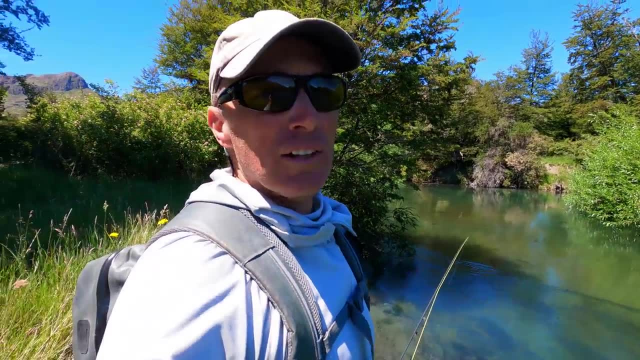 beetle thing and try to draw it laterally over to the left and actually, before i even fish, i'm going to tie on 2x. and i'm going to do 2x because i want to gun the crap out of this thing if i hook up and 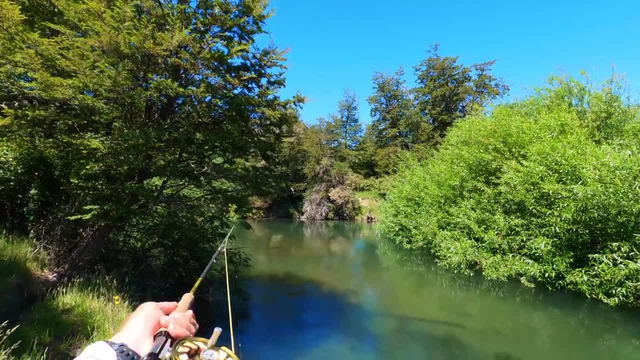 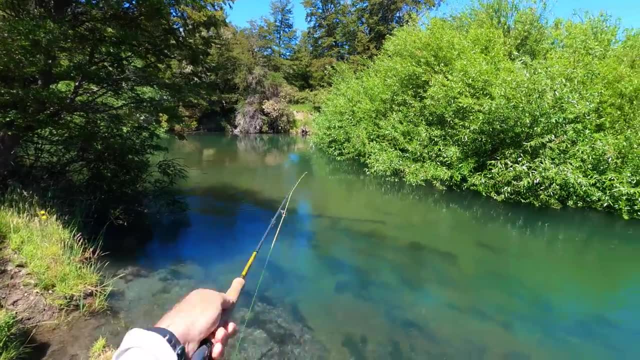 if i can gun it, gun it, gun it, and then, as i play it, he's going to go that way and i'm going to try to wrench it this way and we're going to come. if i hook up, the plan will be this way. it'll. 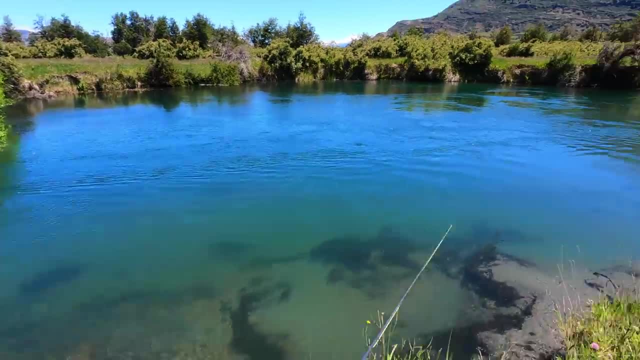 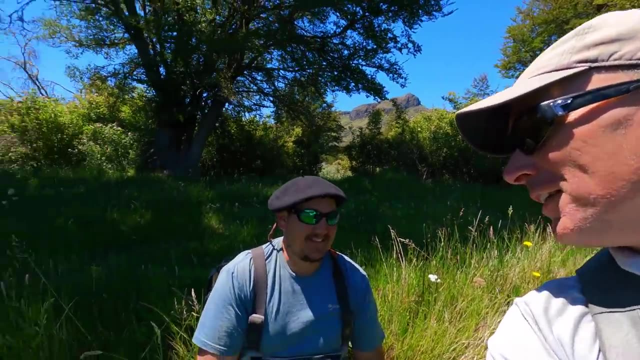 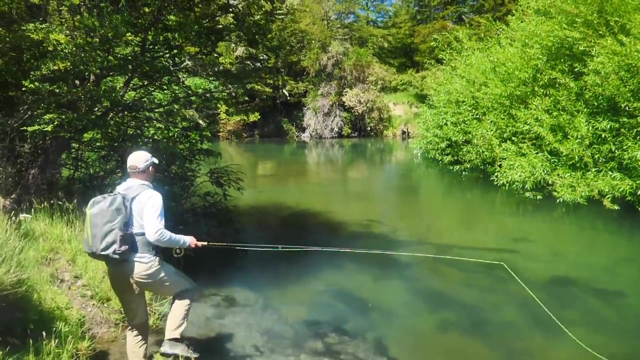 arc underneath this willow and, as it does, i'll fold it this way and try to bring it into the pool. 10 bucks says i don't win, but you gotta try. why, why? why do i have to try y'all? because you always go, gotta try, always try, okay. well, i'll be back in a minute. i'm doing my thing, you do yours, okay. 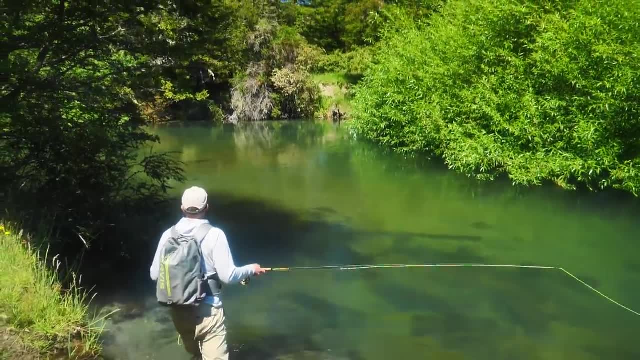 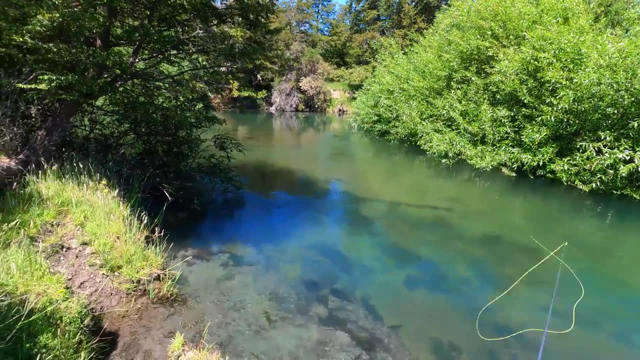 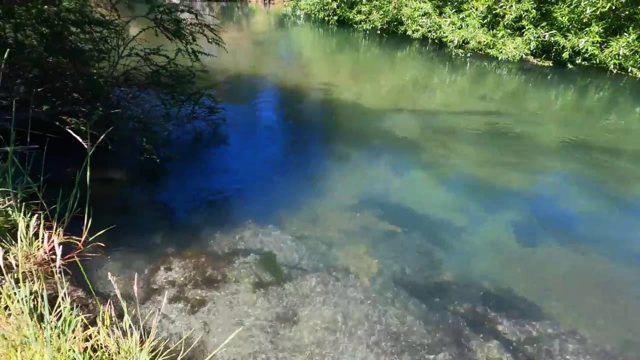 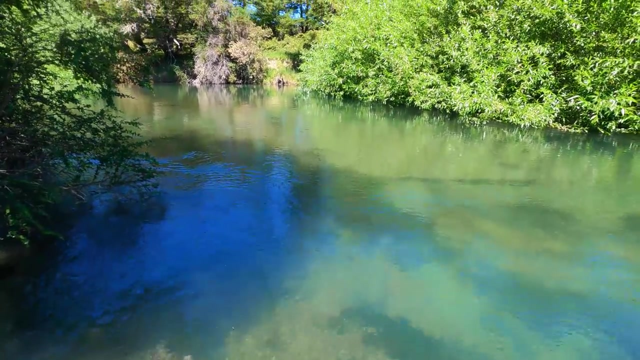 so you see it. yeah, oh, yeah, right, by those two rose petals. yeah, okay, so i got the 2x, i got 2x and with 2x this is a long mother of a cast, so that's deep and it's bushy. will he come to the dry fly? will he come? okay, let's just size up the cast. 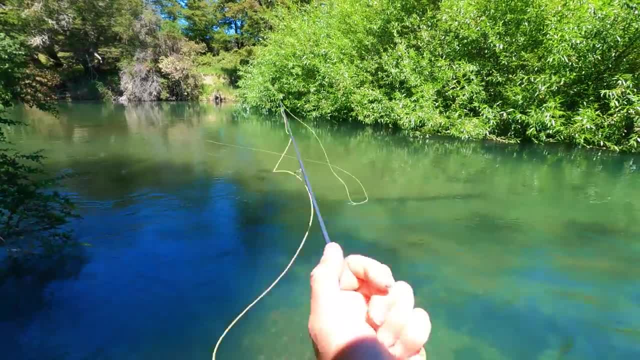 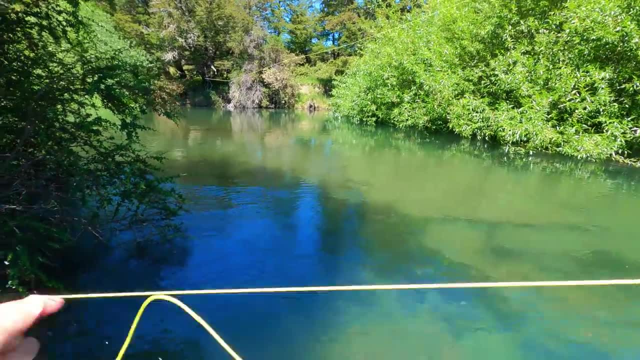 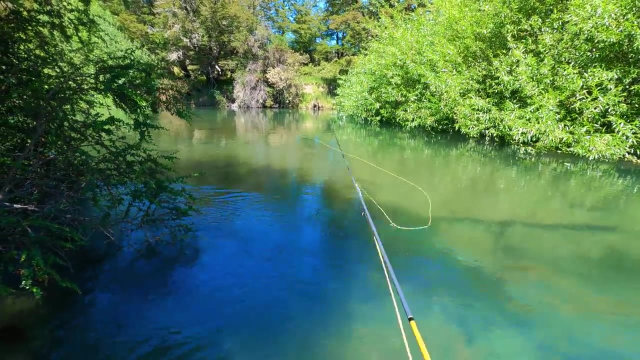 okay, that's not that bad. could be worse, right. okay, now, how about we roll it? gotta come to the left. he has to come. no, that did not go my way, okay, so the wind kicked it back. okay, where's my fly? it was not a good cast. 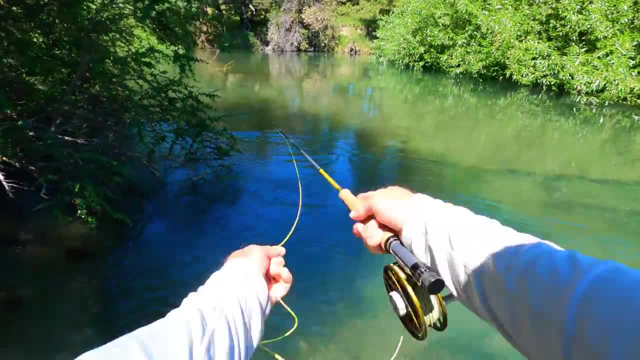 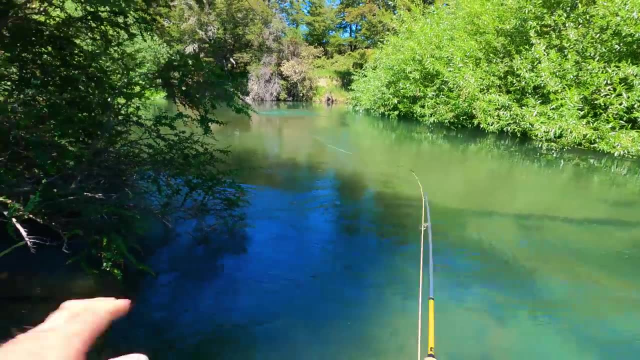 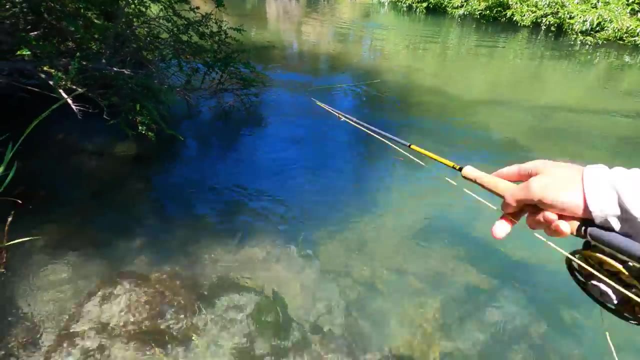 i'm trying to feather it. i don't want to. here he comes. okay, this is my what i talked about under that. oh wait, eight, eight, eight, eight, eight, strip, strip down. see, this is what i'm talking about. will he come? will he come under, under, under? 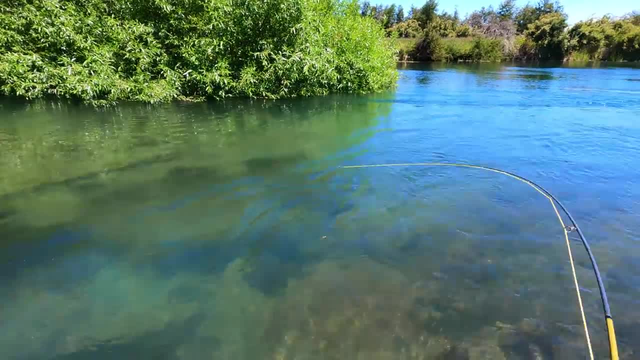 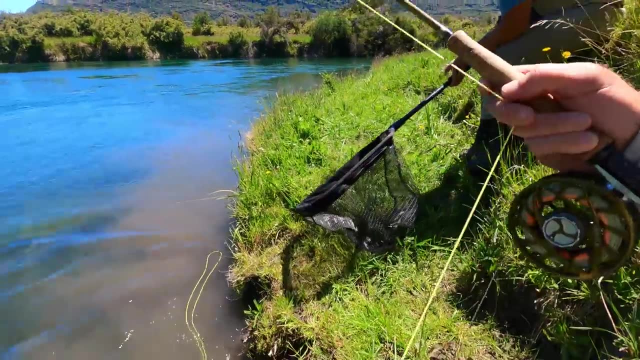 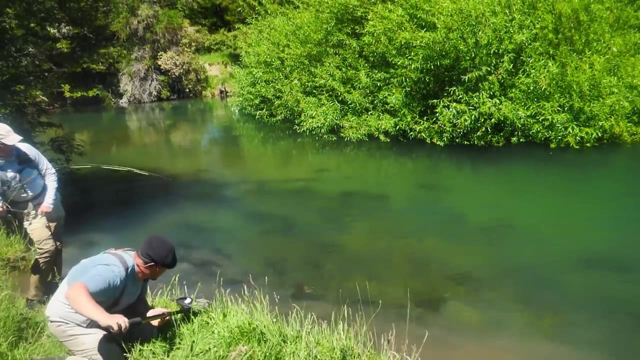 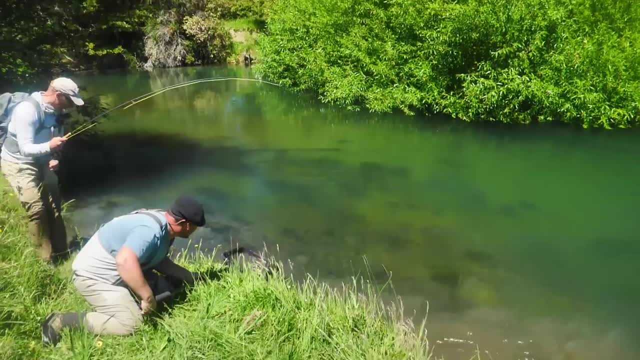 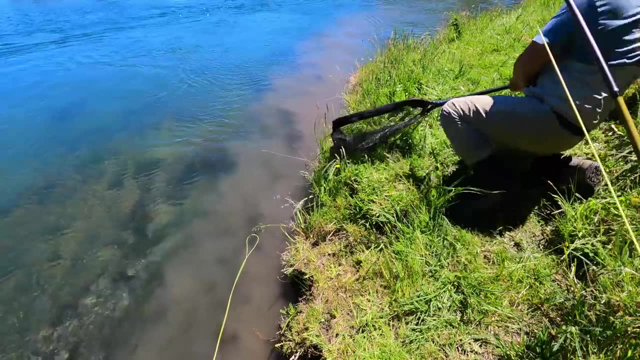 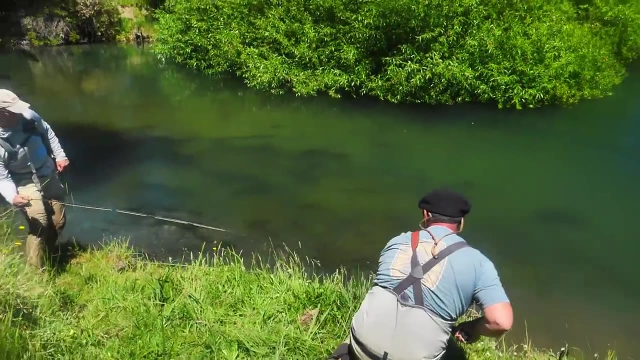 on fish, come on. okay, right, shit, no, no, okay, go down. just a touch foot, two feet, two feet, go go, go, go right there, right there, okay, hang tight, hang tight, come on, come on. no, what should i do here? i know i want to fold this, but 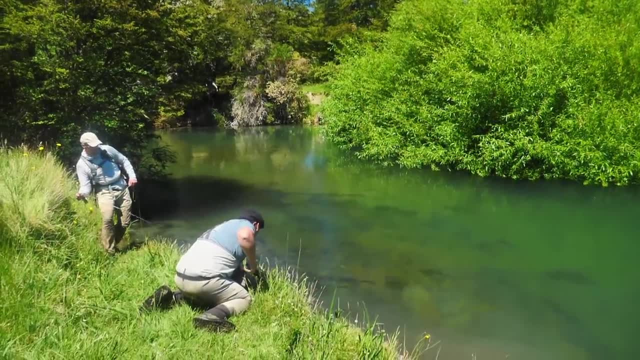 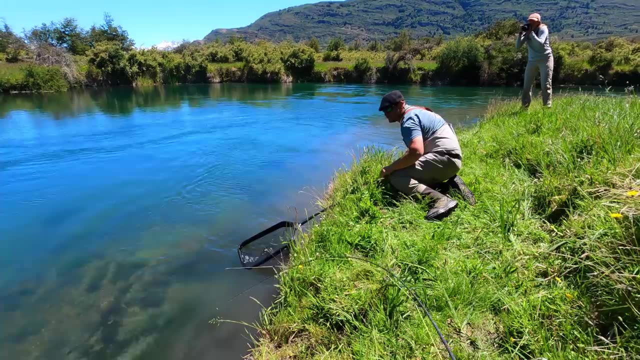 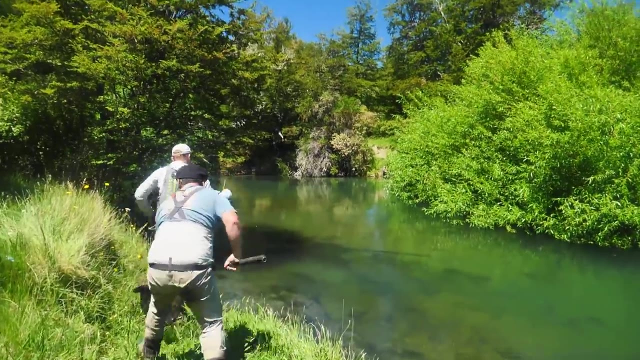 come on, get it up. come on up. come on, fold this way, please, just once. no, i i have such little space to work with here. okay, i'm gonna go this way. okay, i'm gonna try to keep them here. can i try to keep them here? if can you do it, we might be able to fold them. come on, dave. 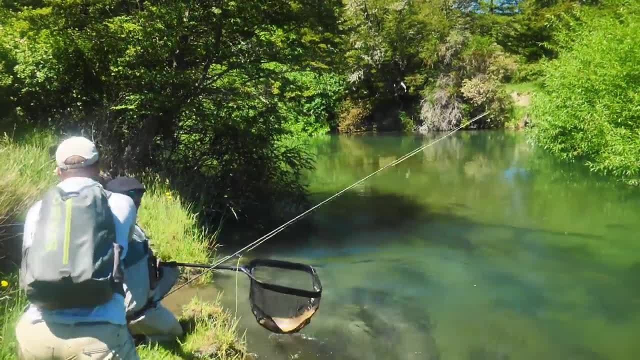 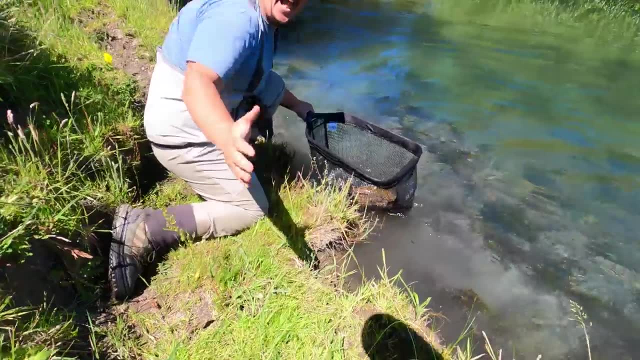 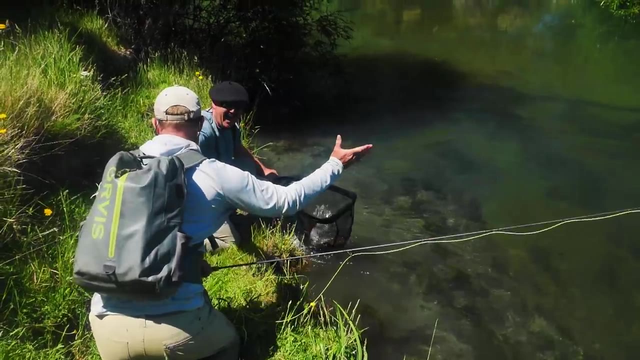 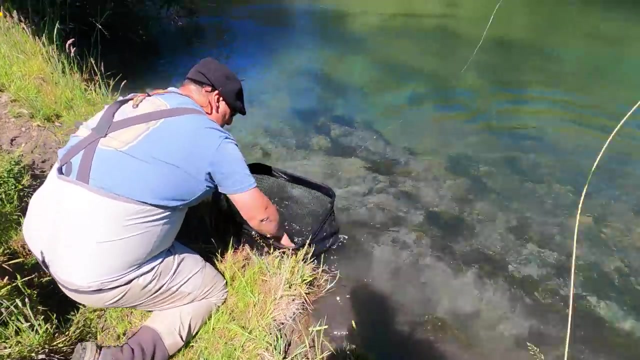 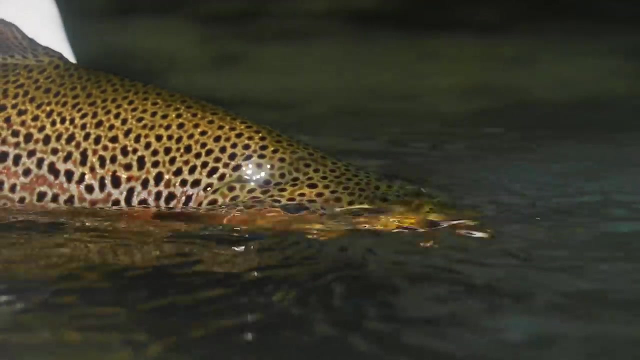 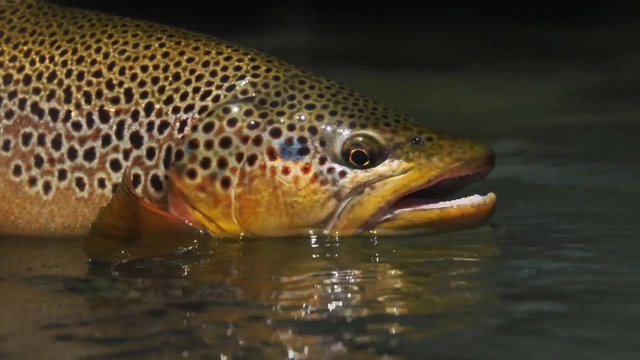 yeah, baby, yeah, yeah, yeah, yeah, yeah, everything went to plan. you don't get that. yeah, yes, oh man, yeah man, no swimming, yeah, no swimming today. you, oh wow, did you see that thing come over? that was the only way was to draw that fish over. hey, awesome man, you didn't have to rescue my ass today. 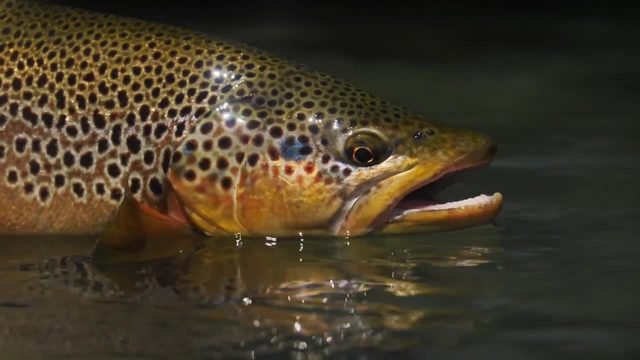 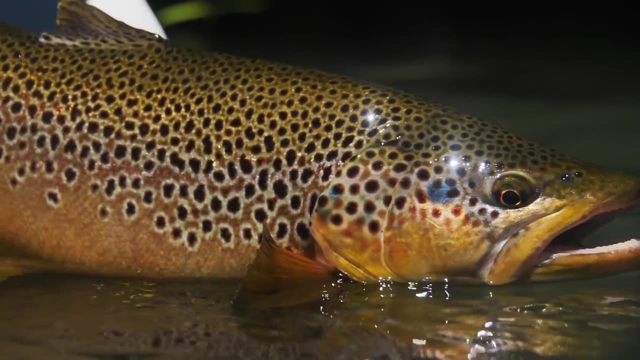 what do you want? love? okay. so it's all, amelia, you tell me what you want. that was fun. i'm so happy for you. had to come. he had to come left. had to come, left. had to come, come. he had to come this way to have a chance. 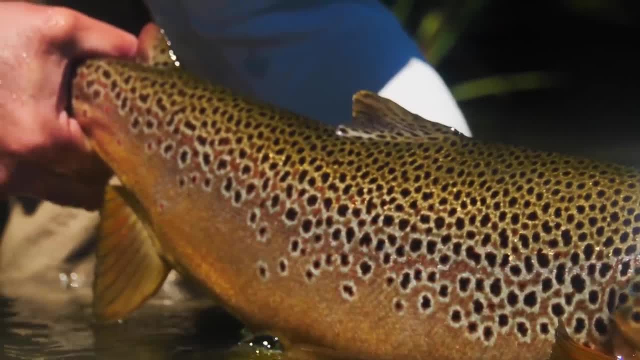 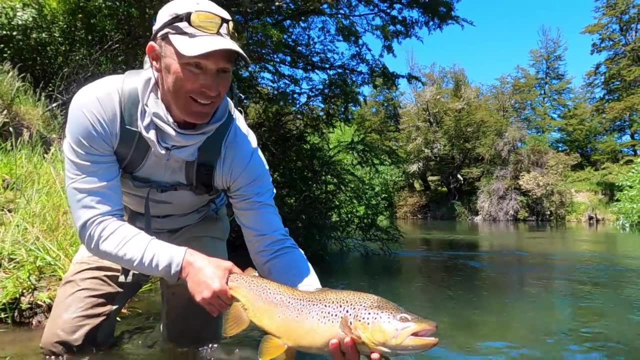 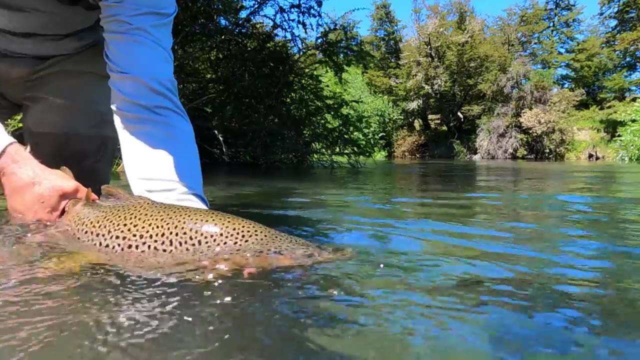 yeah, awesome, here we go. love, what a fish. hey, dave's gonna go down. yeah, we gotta get out of the back here and i'm gonna come back up and up you good. yeah, okay, here you go down, okay guys. so if it sounded a little, a little bit doubtful and kind of 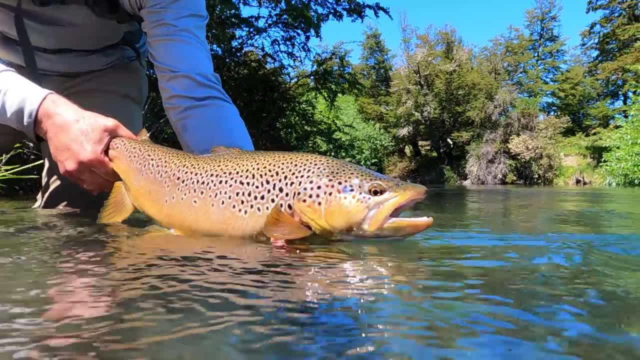 self-deprecating, but at the same time cocky to call that kind of a shot. how would that? at the same time cocky to call that kind of a shot? we did it by shooting six times. we did that thing by shooting seven times, at three times. 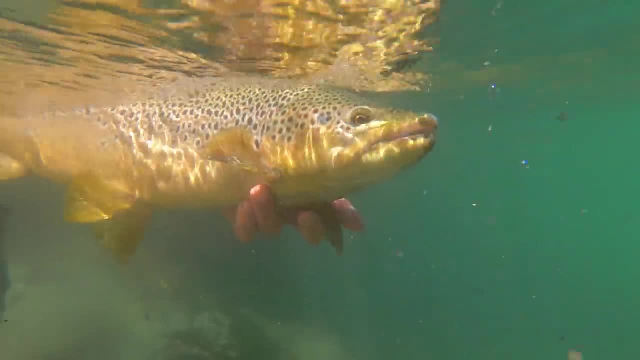 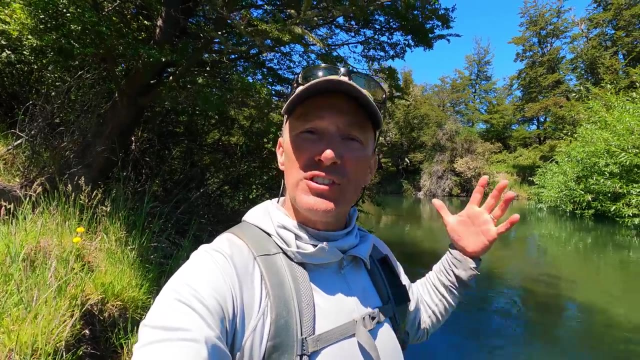 did. I know what I had to do and and I still needed luck full stop. you have to get lucky with those and I got a lot luckier than I thought I would. but we've seen Browns come to flies and you know you feed the fish well during a hatch. 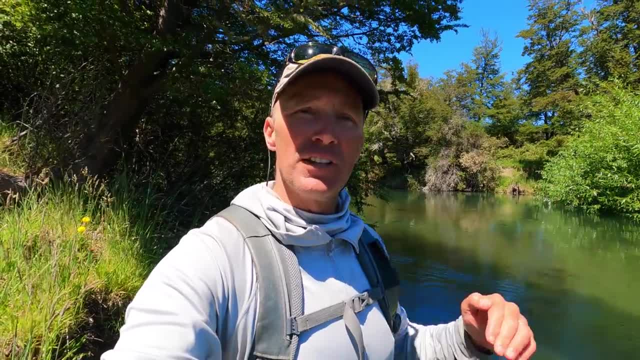 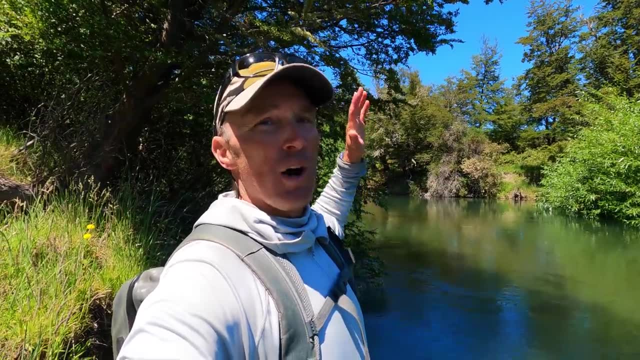 you can feed the fish, cast to its feeding lane and drift into the fish with terrestrials. you don't want to do that, you want to put it to. you know. in that case, I knew where that fish was. I wanted to, I wanted to smack that fly. 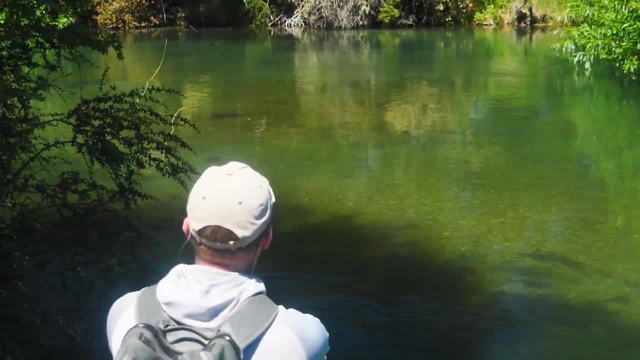 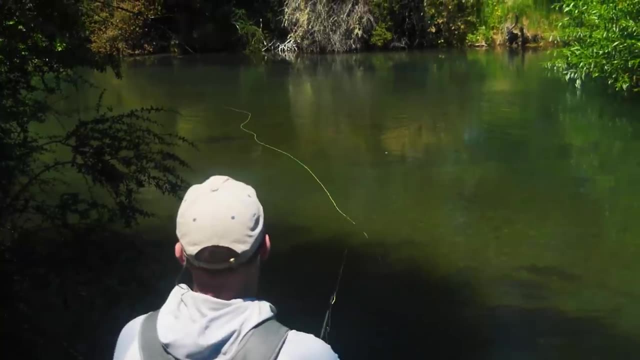 on the surface with a smack and let it come three, four feet over. it's something you see in New Zealand all the time with cicadas. you see it with beetles in New Zealand. you see it at home in Canada with grasshoppers. you see it in Montana. 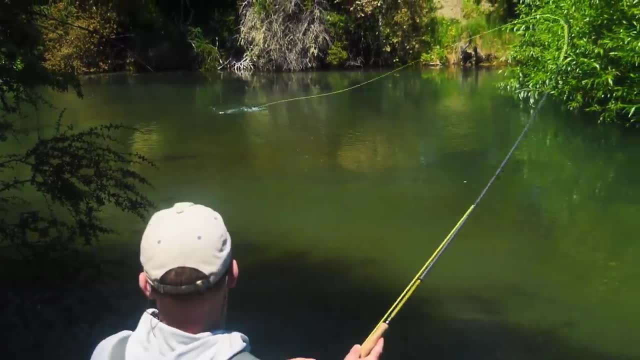 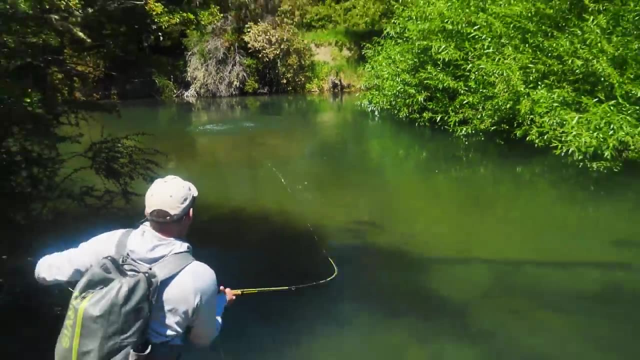 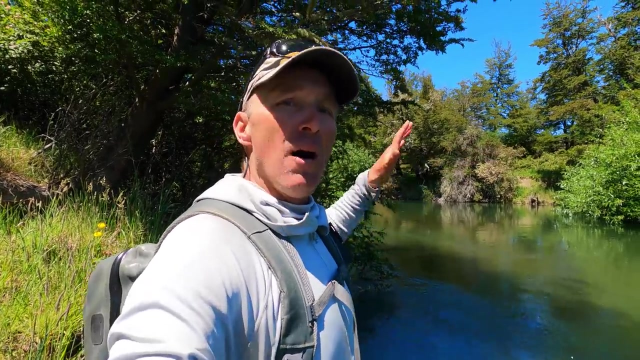 and the States with grasshoppers let the fish come to the fly and I knew before I even fished to this fish that I was gonna get the take. if it wanted a dry fly, it had to come to the left. I was not going to allow myself to cast to the fish and risk it turning to the right. I 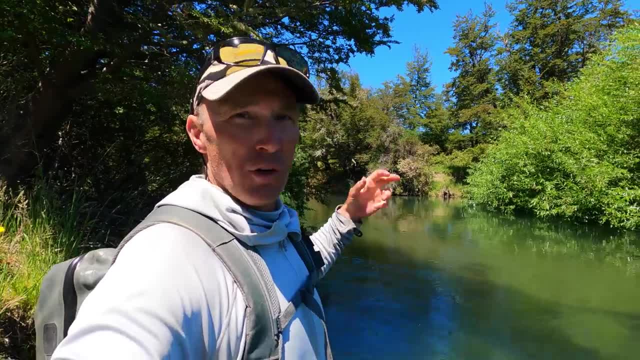 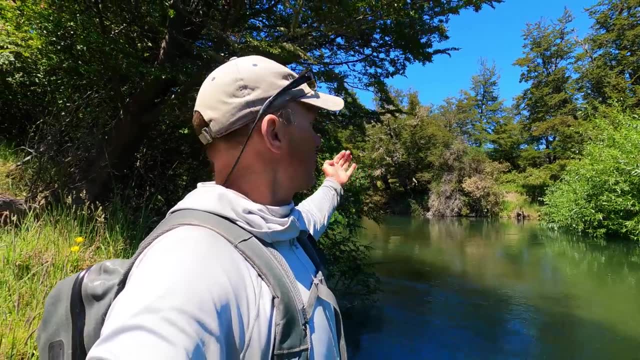 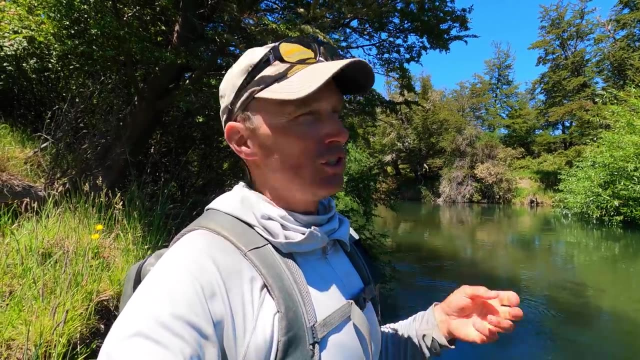 wanted that fish coming left. why proactive? you know the old, proper prior planning prevents piss for performance. get it coming left, then when it eats left, hopefully it turns to you or just or goes back and you can hold it back. those big male Browns usually aren't hot rainbows. they'll fight by rolling and in. 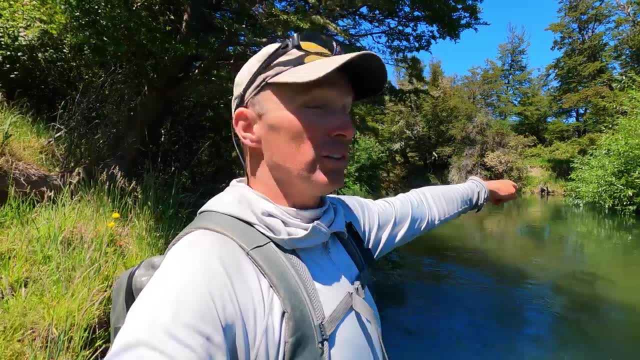 this case, that guy came out here and it was like: okay, I knew, hold it along the willow, hold it along the willow and, like I said before, I even fished to it, there's gonna come a point where you're holding it like this, where 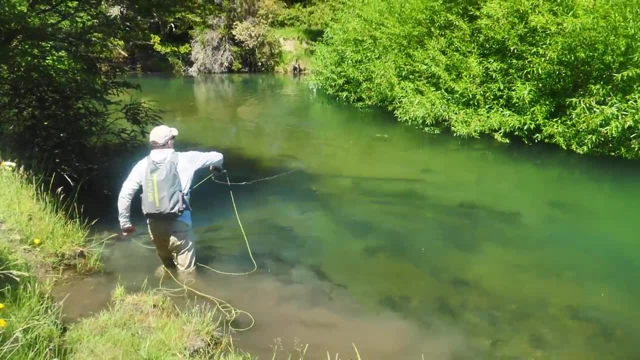 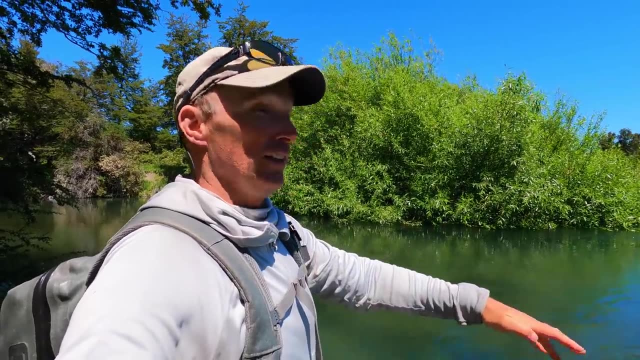 you have to fold it like that right now in order to get that pressure to keep coming and, drawing and pulling it from this side of the willow. you do that, you got a chance and then it kind of came over and it's like, really, this isn't. 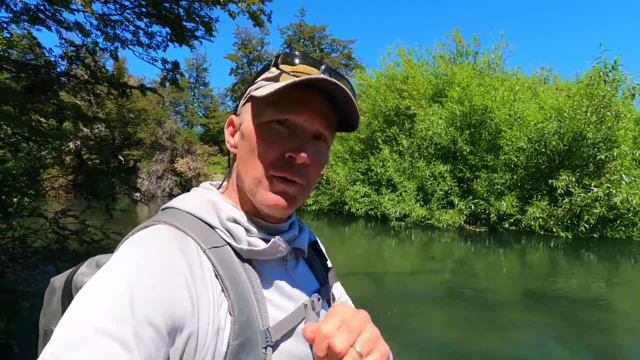 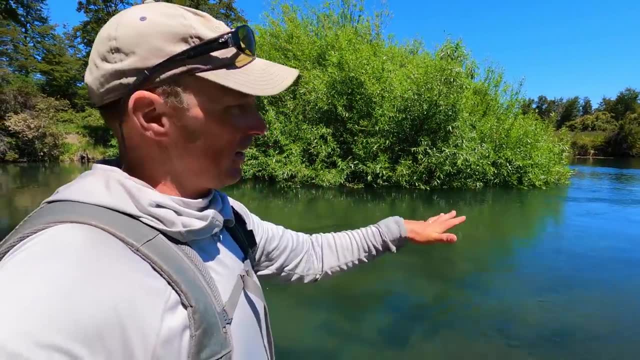 not going to last that long if that tip it holds. that's why I went with 2x in order to crank this fish out. quite often along this edge right here, those pec fins will flare out like that and it'll be a good catch. just glue to the bottom. well, that thing allowed me to pull, pull, pull, pull with. 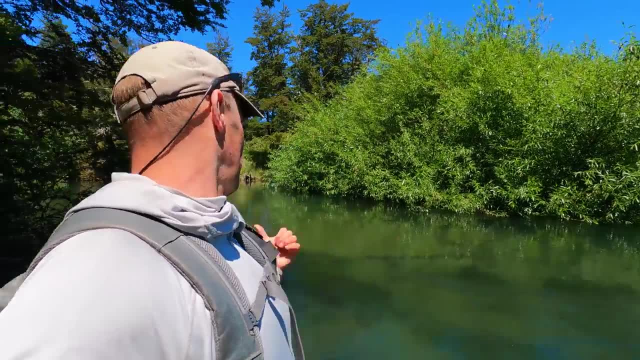 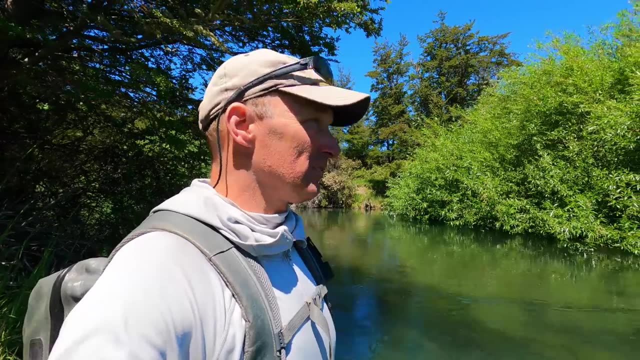 that 2x and bring him up and boom, boom, boom. and then he came up here. it was like, okay, we have a chance to fold them right off the hop. and I still think it was a seven pound Brown, I don't know plus or minus. well, I don't think it was. 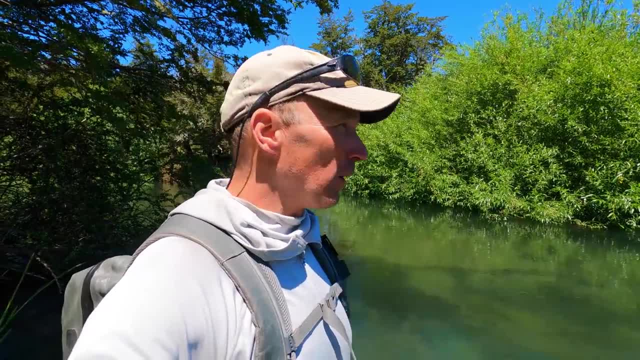 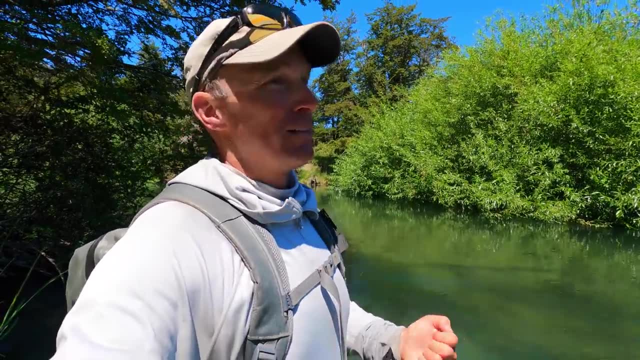 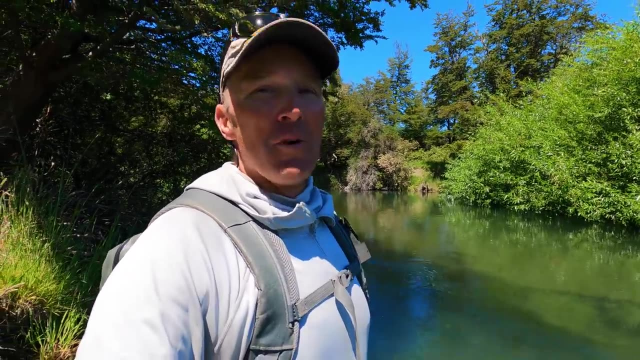 eight, and I don't think it was in the sixes, I think it was in the sevens somewhere. and those are the ones that sometimes you can stop their fat rolling behavior and flip them into the net. and our friend up there, Marcelo, was there with the net- was like yes, and we got him. 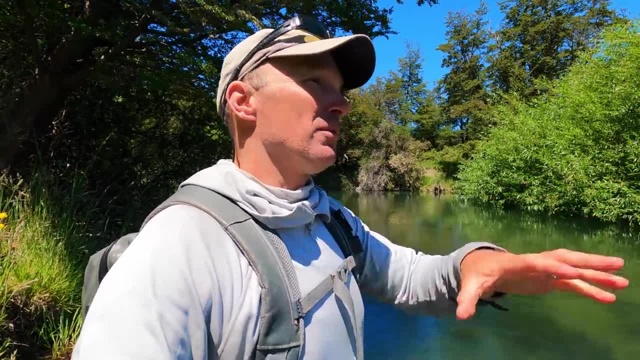 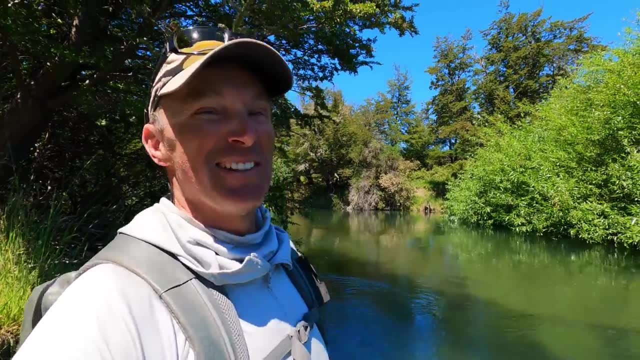 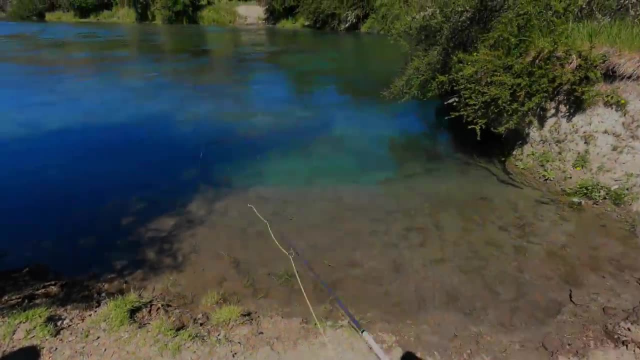 proper prior planning for his poor performance. we got everything that we hoped for and we got some lucky breaks and we got one hell of a fish in a stunning location on a great day here in Chile- just amazing, okay, so we cannot see. we've got shadows and we've got a really nice bank right here. 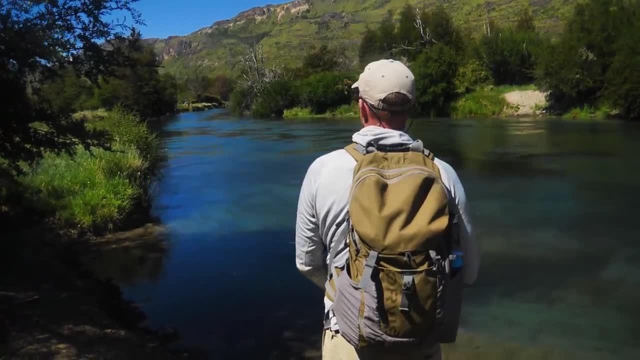 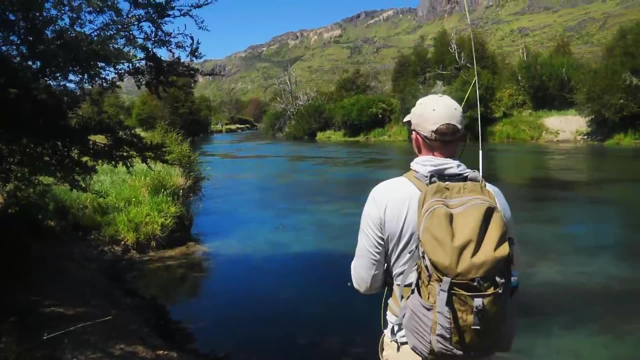 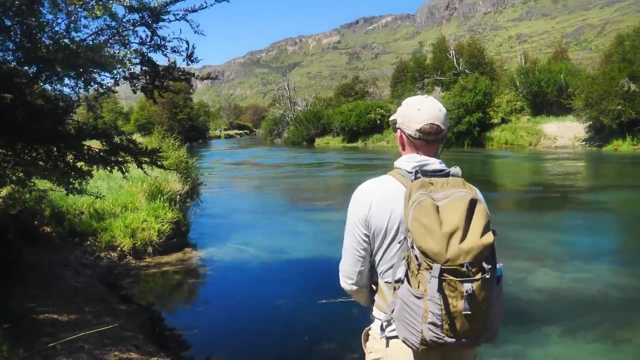 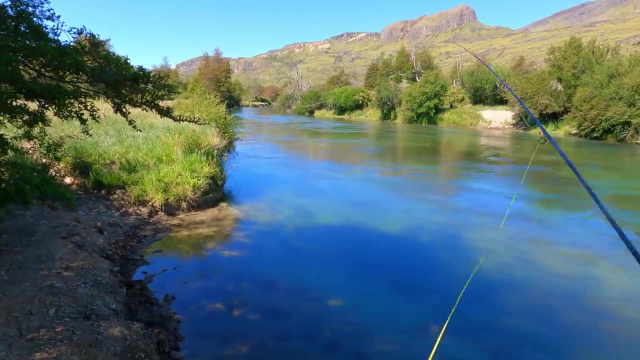 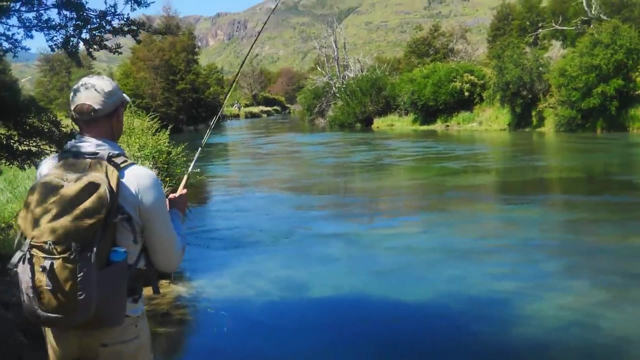 has to be a fish kicking around here, just try to stream it out. anybody come out a little tighter, not that cast a little out draws anybody out. no, smack it. anybody want to come out? yep, there he is. I always have to work those tail out. undercuts, always a little. 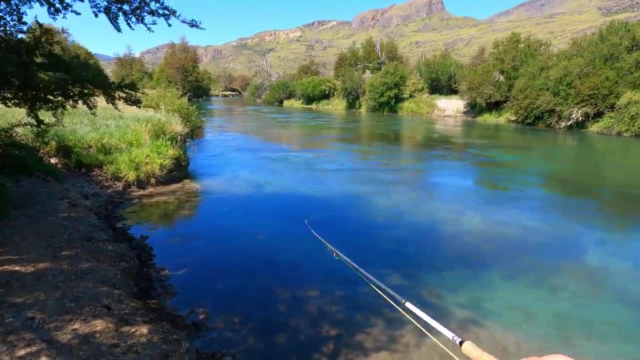 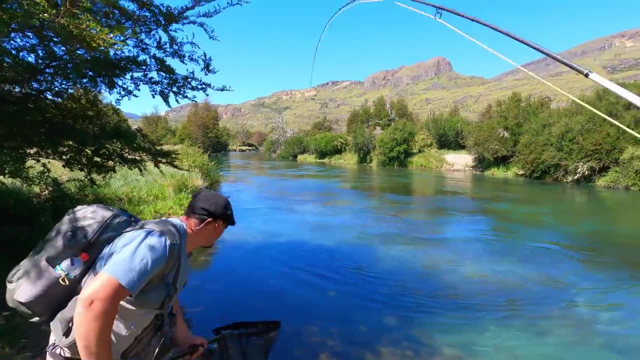 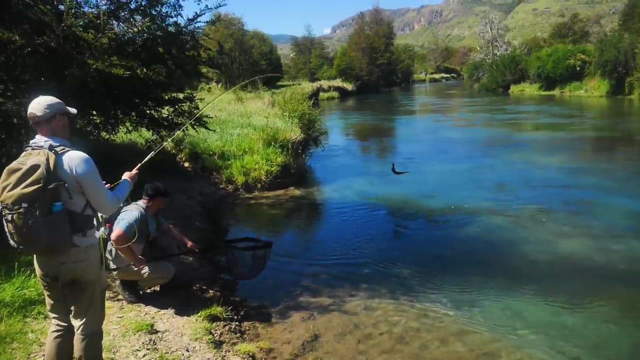 brownie around Amelia with the call on that one, though: take the time. she said: take the time, yeah, yeah. it says: take the time, that's what we do, yeah, hopefully, hopefully this one doesn't get ahead of steam and cut down the shoreline, cuz I'd be pretty much in trouble. 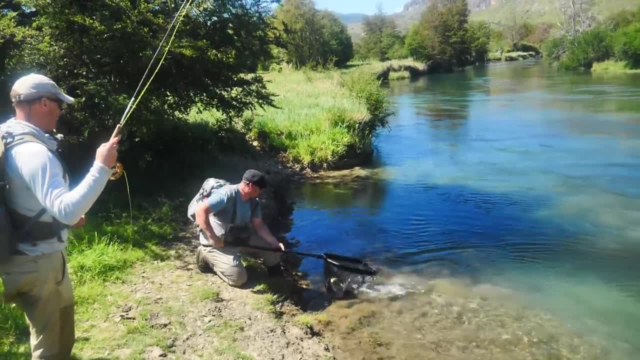 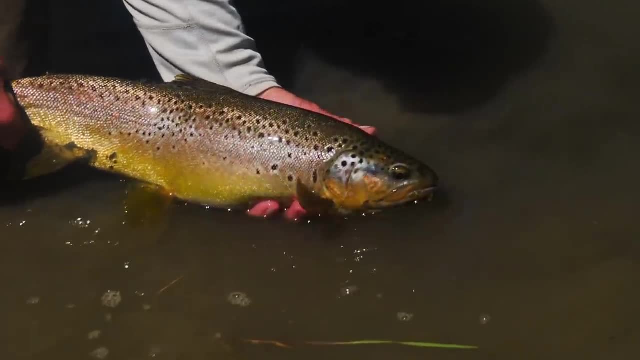 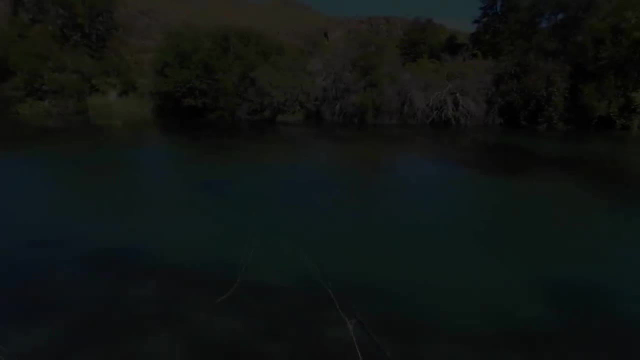 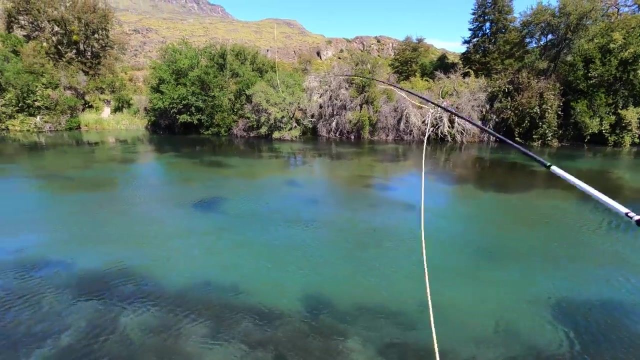 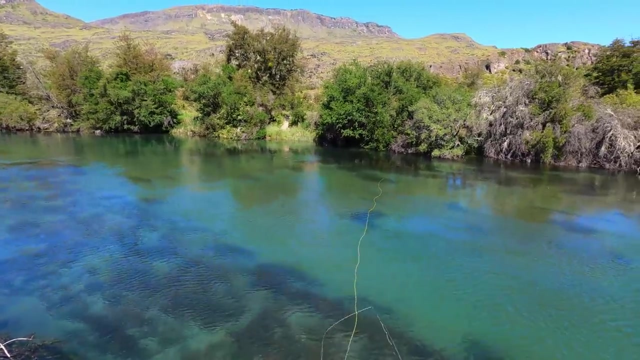 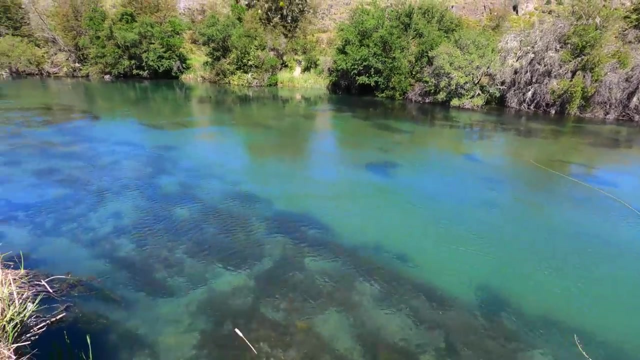 at that point, fold little buddy. thank you, awesome, sweet, they're so heavy. hey, every one of them is a fat little bugger. yeah, yeah, so you want to just video the release kind of thing, or size this up? try this. did he move? that was below him, I think. okay, I have to just come this way, don't go any. 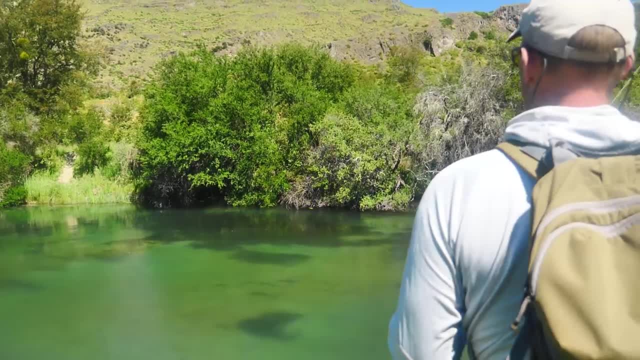 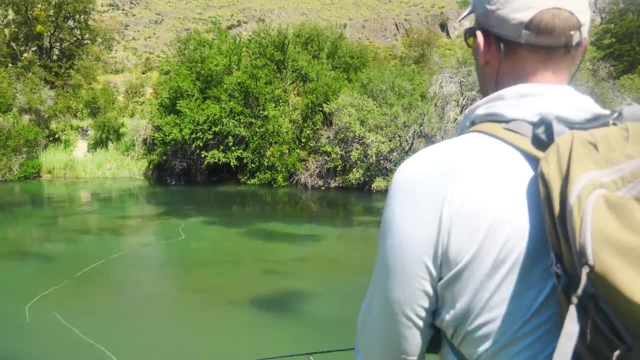 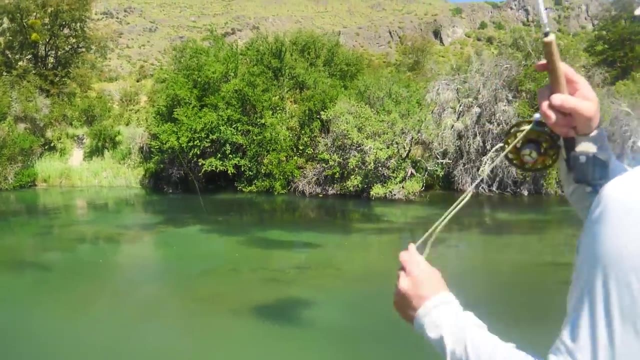 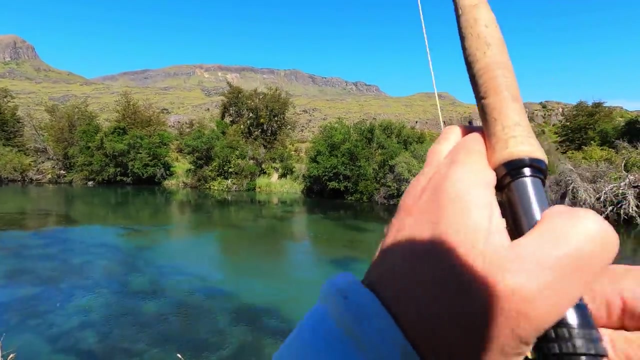 further over. yeah, now I got my ear on that cast. okay, yeah, I'm gonna try that's big fun. yeah, I'm gonna try that's big fun. yeah, I'm gonna try that's big fish, though whoa try to keep them out of your fish in the middle. 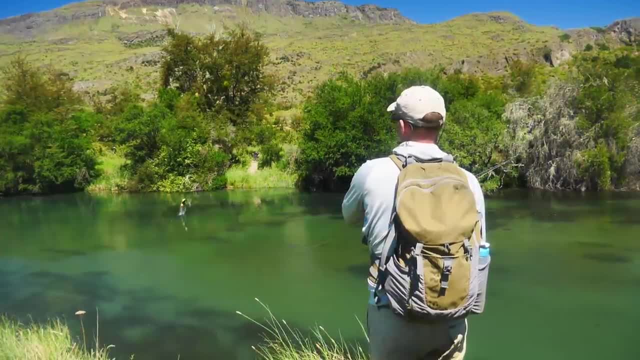 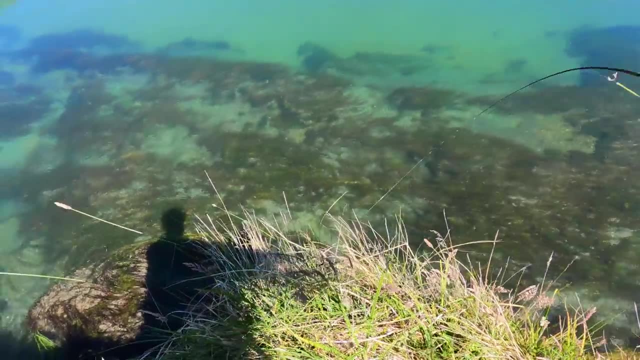 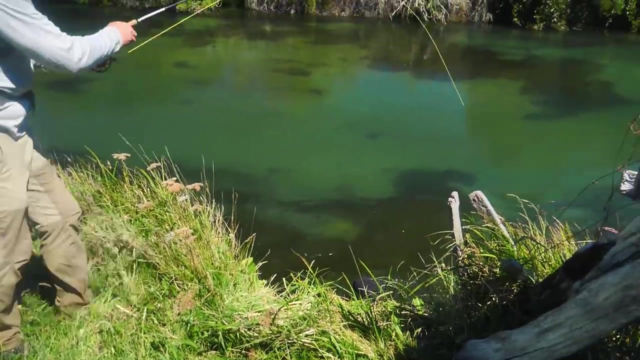 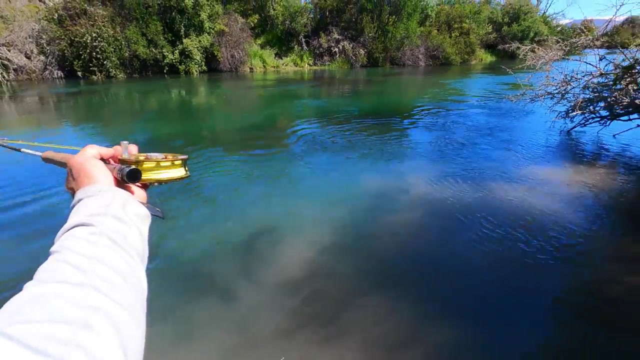 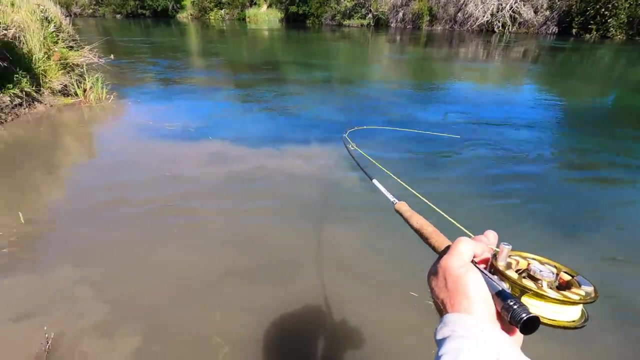 here. try, that's. a big fat brownie is what this is. yeah, watch that other one, though. still it's good. yeah, see, my problem is I can't control that fish from here. I can't control this fish. see, turn, turn, turn, turn, turn, turn. just try to walk the angle back. kite this fish and 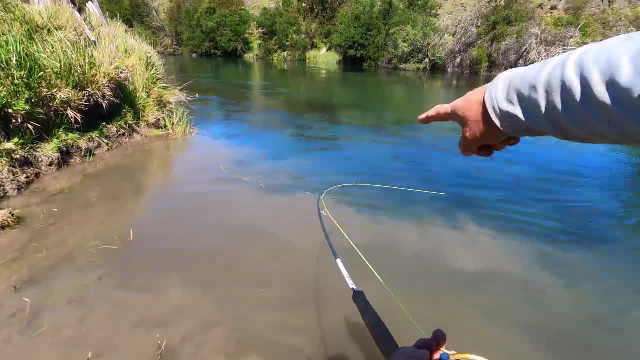 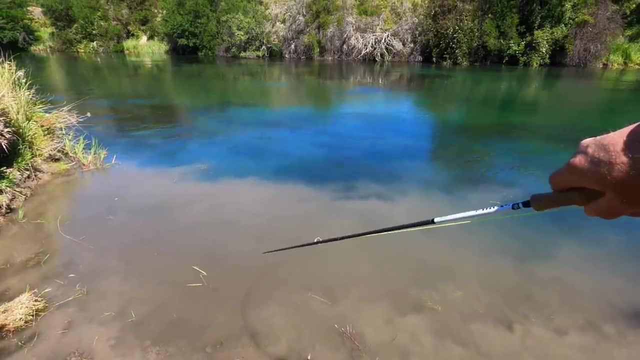 you're gonna be right here. yep, I'm gonna try to get them upstream of you. then I'm gonna try to fold my rod this way. it's the only chance I got to try to keep them low. I'm gonna if, if I can get the angle on him here, if I can fold them. 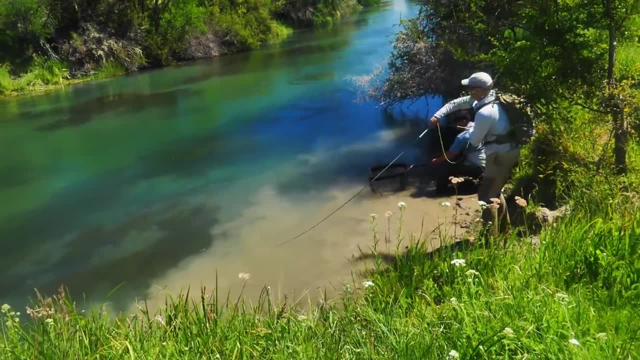 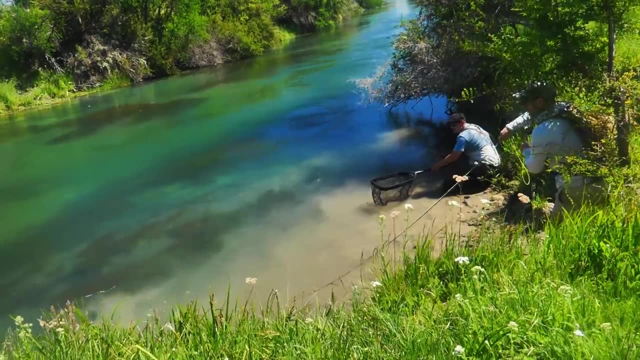 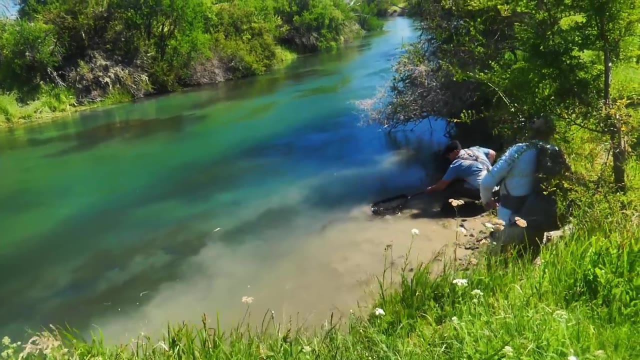 this way. it's a big fish if, at this point, as soon as i fold, i'm going to fold right at you. okay, three, two, one. no, i don't like that angle. no, i'm gonna fold them this way into the net. in into the net. yeah, i thought he. 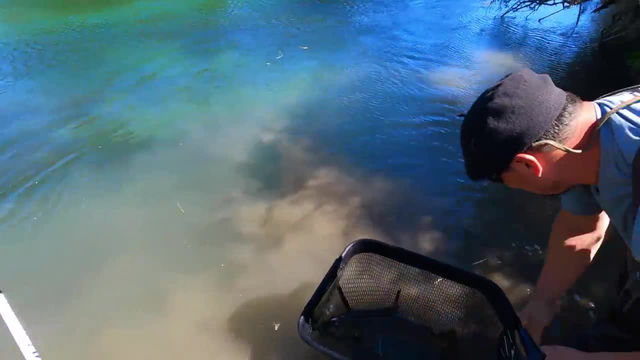 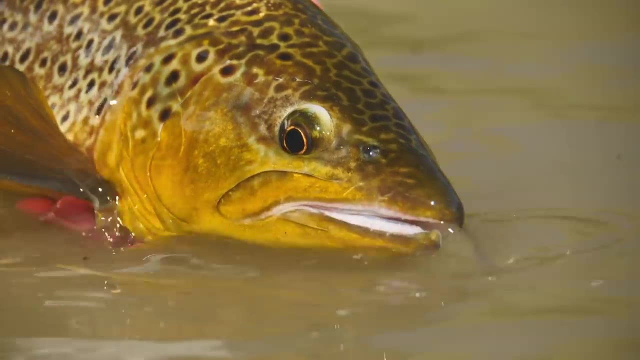 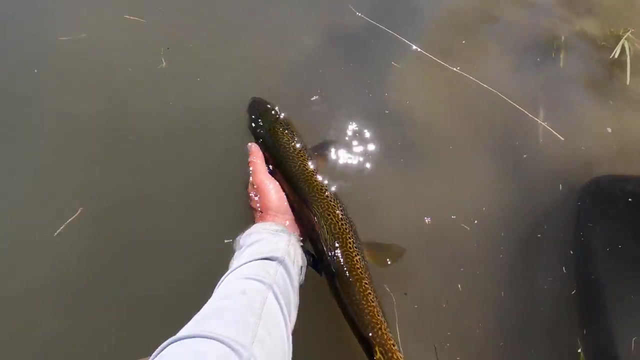 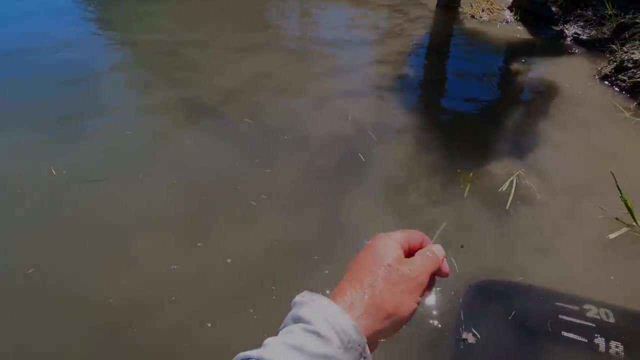 was a goddard, haha, yes, awesome, oh, that's lucky, that's lucky, gorgeous fish. yeah, you ready, it's beautiful. okay, it's a stunning fish. here we go. look at that was a gorgeous fish, lucky, yep, we've. we've got a gorgeous, uh, brown here, guys, it's. 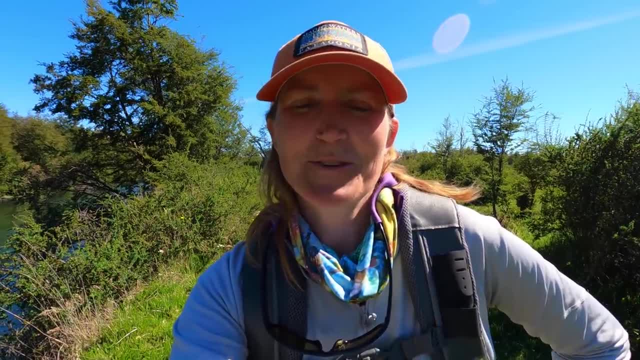 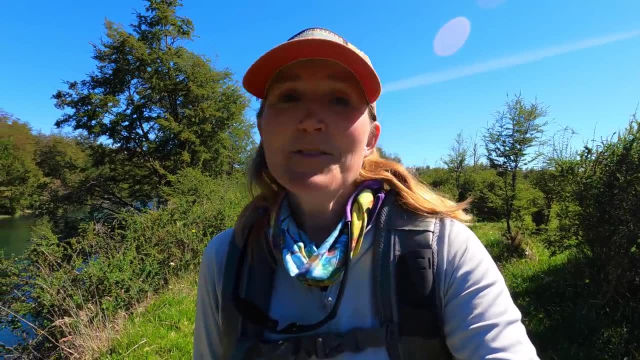 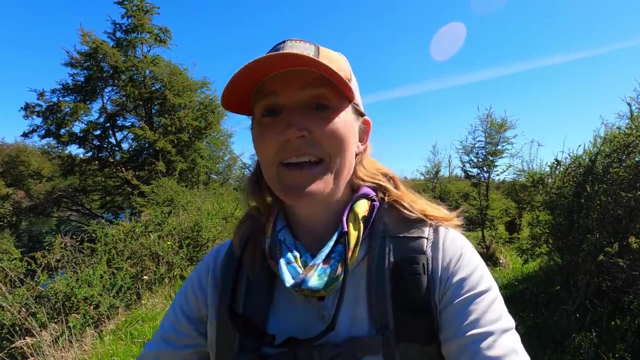 surfing the back end of a whale weed bed and, yeah, it's just beautiful. you can just see his gold shape just kind of swaying left right in this spot and uh, i'm not sure about landing this fish because the river right here is actually one big sort of giant causeway and we've got a lot of califate on. 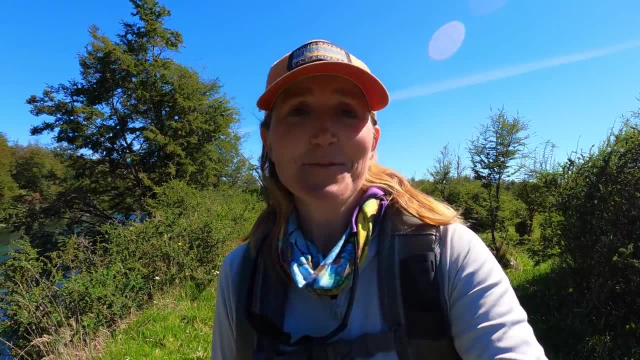 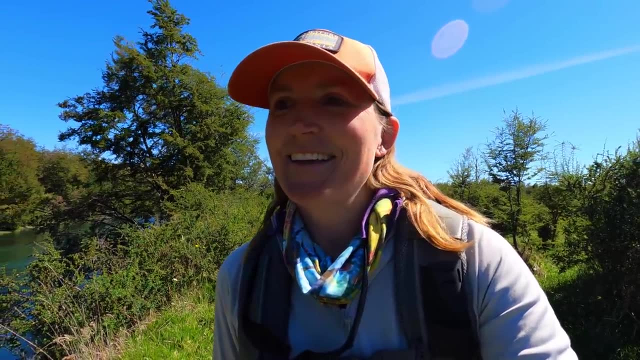 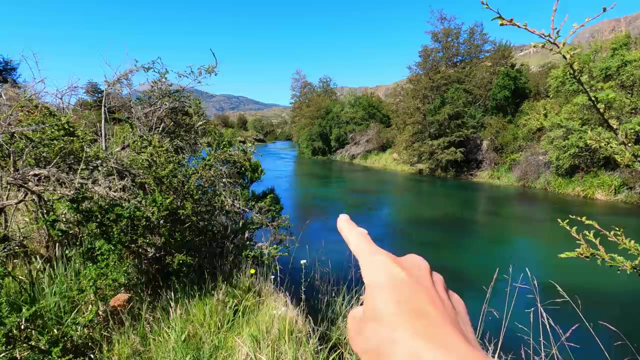 the banks, and not not many too. not too many places to go down where it's actually shallow enough. but hey, um, hook up should be pretty sweet if i get a chance for it. and uh, yeah, so he's just literally out. oh, there's califate bush off left here and he's just out from it and swaying back and forth in. 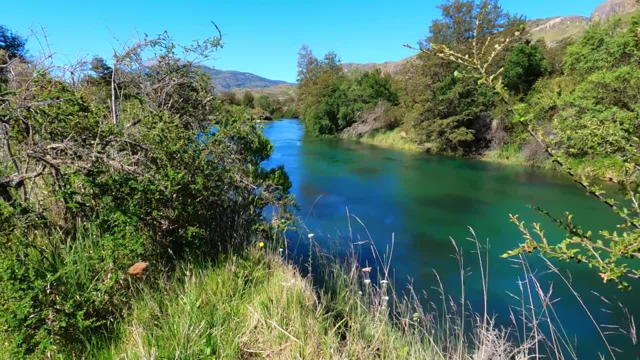 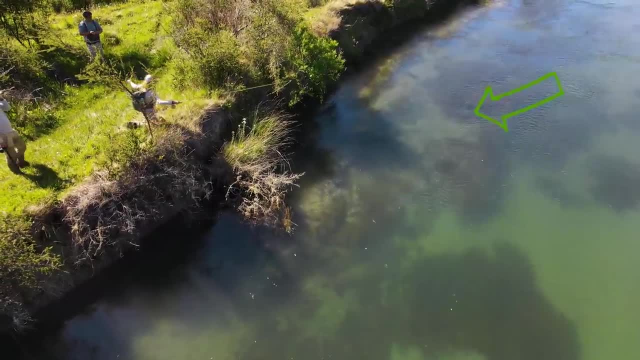 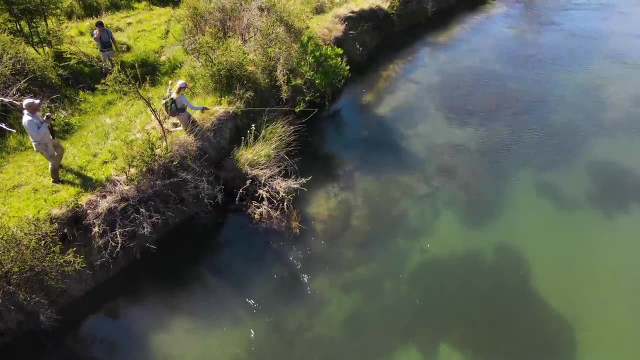 there. so it looks like the spot that i'm standing in right now is probably my best cast to him. i mean, i'm hopeful that getting forward like this and waving my stick isn't gonna kill my opportunity with him, but i think i have to go right from here. 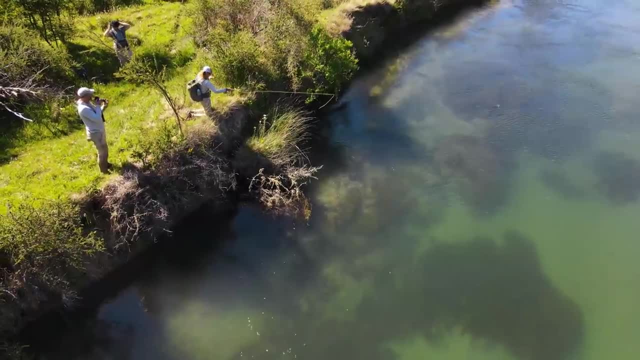 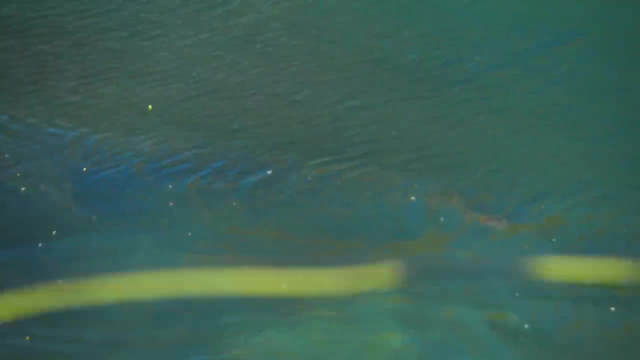 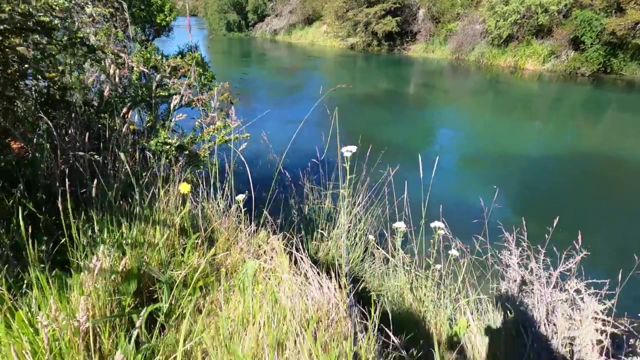 okay, yeah, i think. so he just rode. oh, perfect, okay, that wind's gonna be a bit fun, it's gonna be a bit wiley wiley here for me, so i'm gonna wait, pause for a break in it and then go. okay, guys, so i've now actually changed up to a grey stone pattern because he didn't. 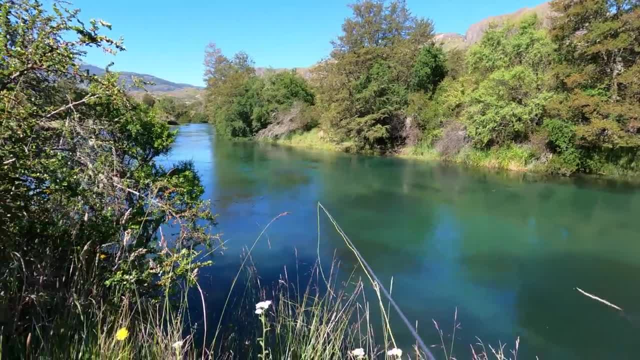 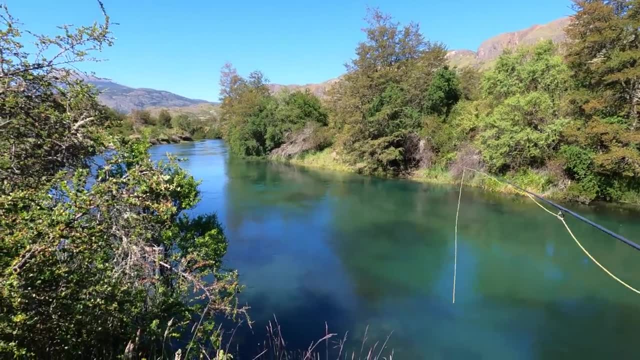 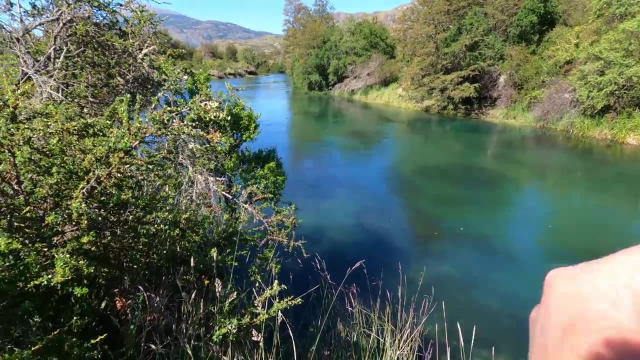 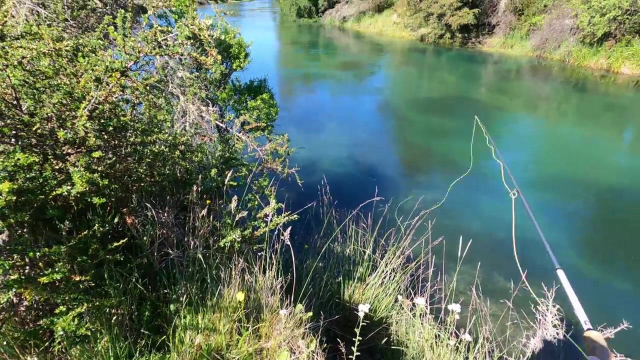 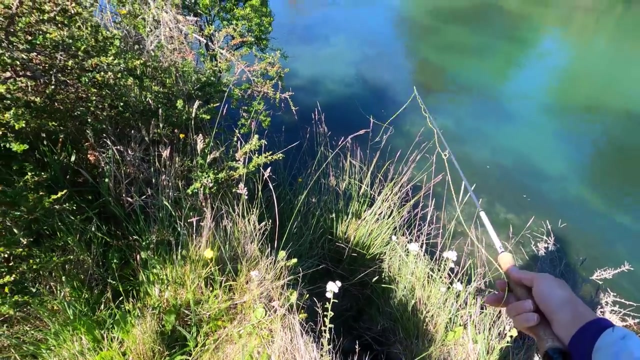 want to eat the small beetle or the sedge. so, yeah, i'm gonna go with that. now, here we go, let's see what happens here. okay, okay, let's give this a go. okay, oh, he looked hard. you saw that. yeah, he looked hard. no, okay, I'm gonna go to actually go a little bit to his right, but don't lead. 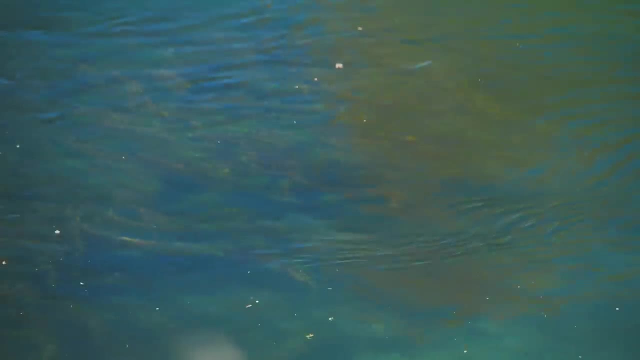 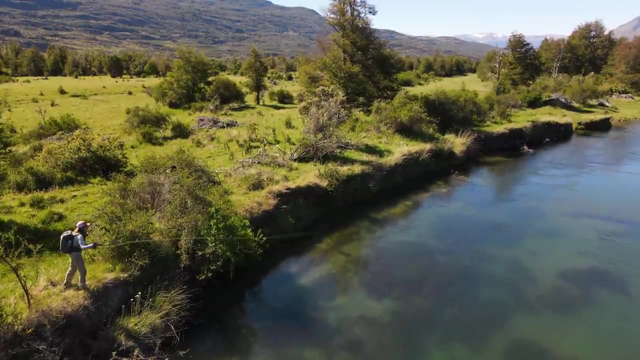 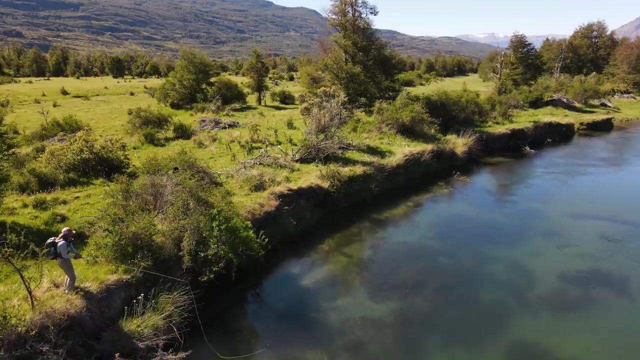 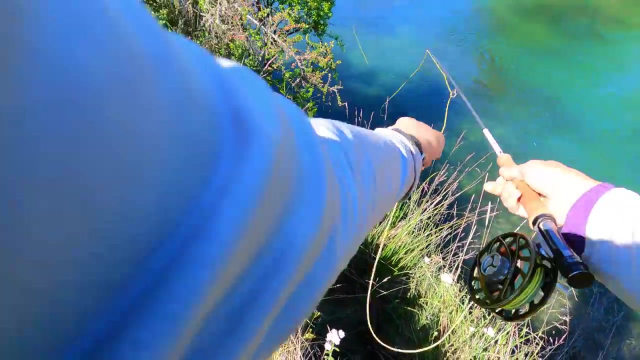 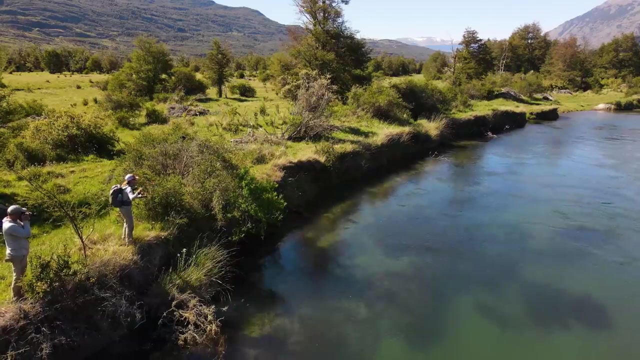 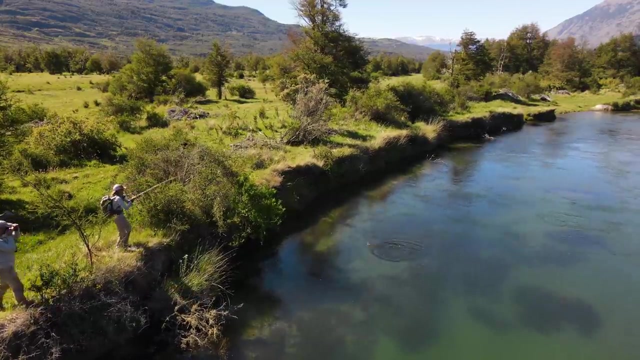 him so much he didn't know. refusal, huge refusal guys last minute. Kate, dropper, nymph, it is Wow, Wow, Wow, yeah, right on, okay, here we go as a chance if he wants to come over. no, I got to get right on him, yes, and eats the dry. oh, I think it dropped to the dropper. good luck, good luck, good luck. 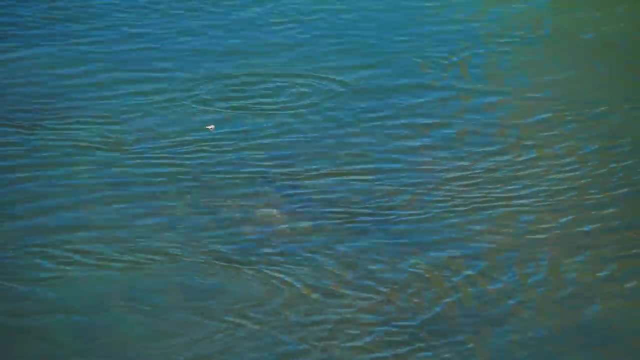 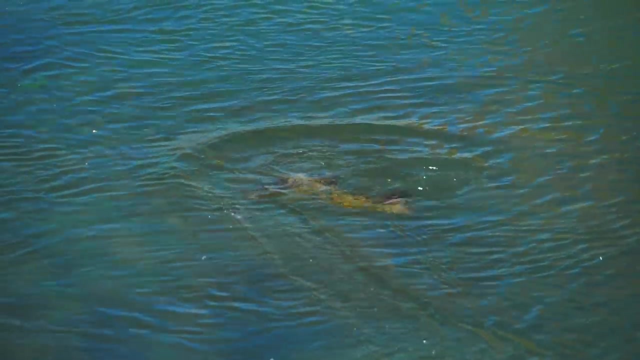 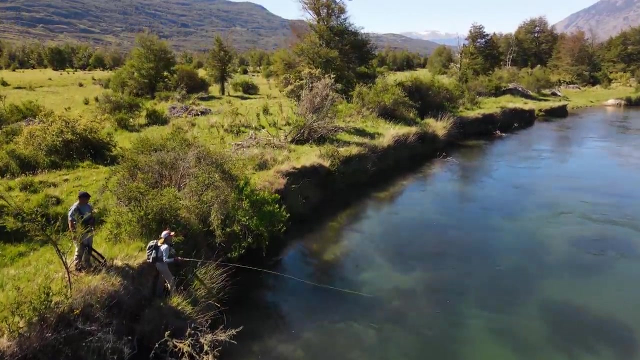 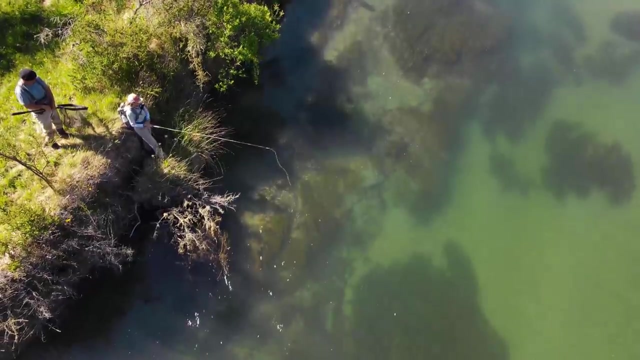 good, heavy fucking fish, heavy, heavy, heavy fish guys. heavy, heavy, heavy, heavy, heavy heavy. I don't know man, I don't know. he's in that weed like nobody's business. oh, no, he's off. pop, he's off. no, he's, yeah, he's off. holy crap, that was pretty amazing. Wow, Wow, Wow. what do you think of? 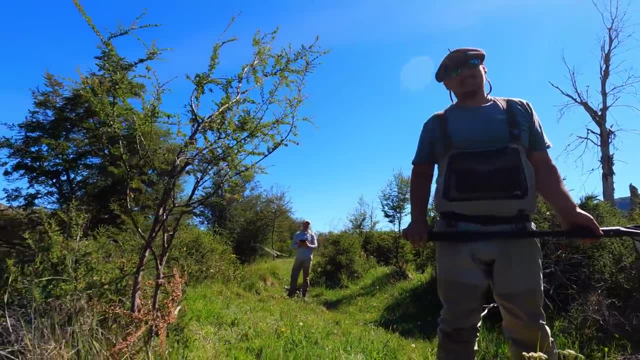 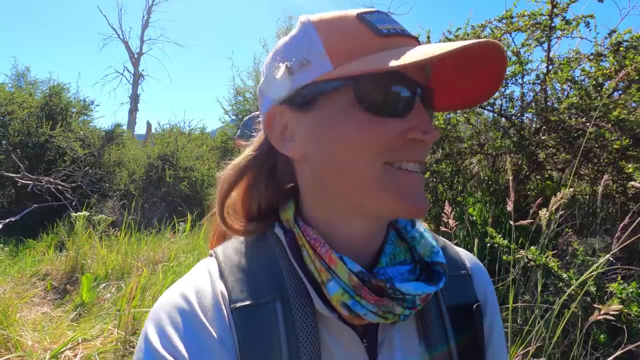 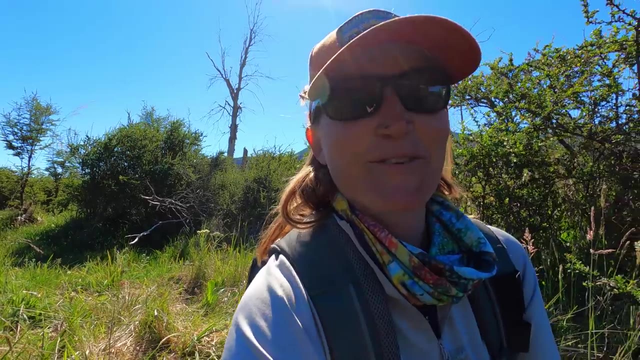 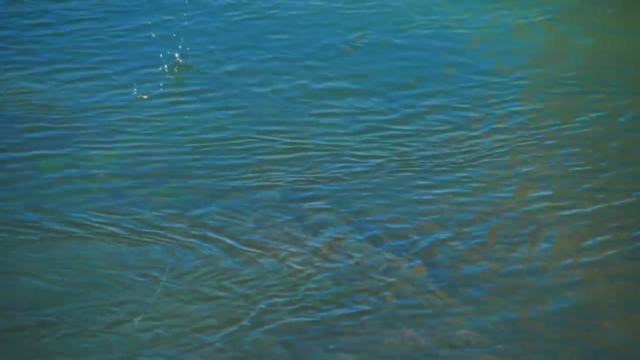 that Marcello. hey, thanks, man. well, guys, like I said, you know, fighting this fish, getting it to land, non-starter, but yeah, that was fun, what a fish. so, after all that guys, timings, everything you know, I put on the caddis pupa, but that fish came and took the. 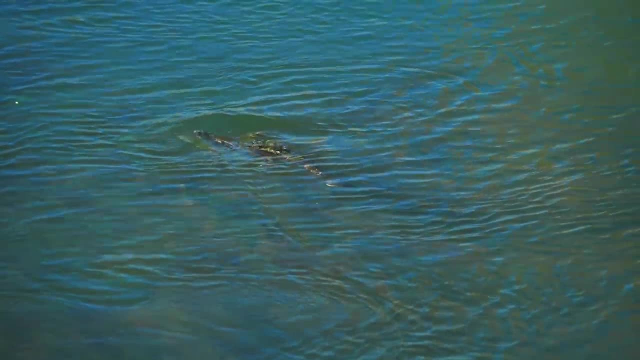 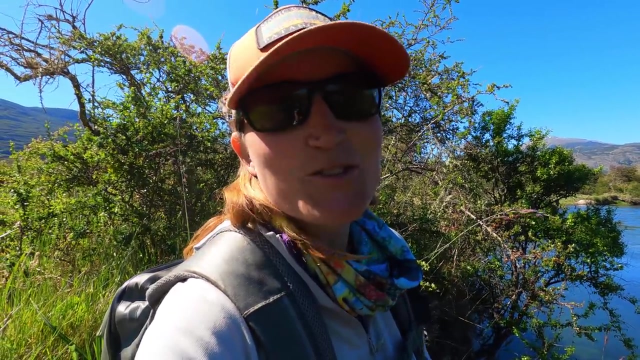 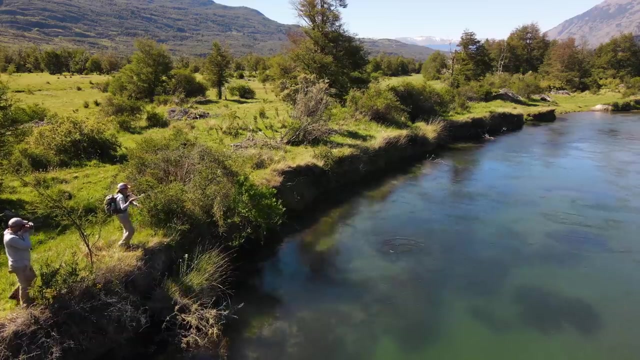 dry fly just smoked the the old gray stone pattern. so yeah, Wow, what, what a fish. so much fun, heavy weed. I mean that fish jumped tore into that heavy weed. there's actually a lot, quite a lot of current here, current pressure. you can see that in there, not much of a break. 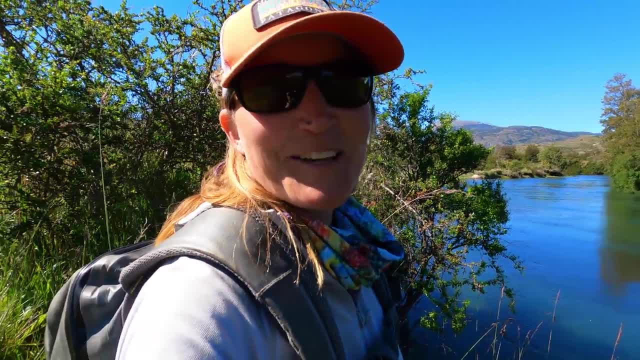 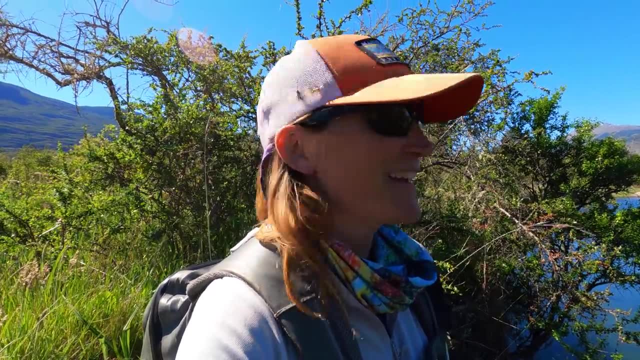 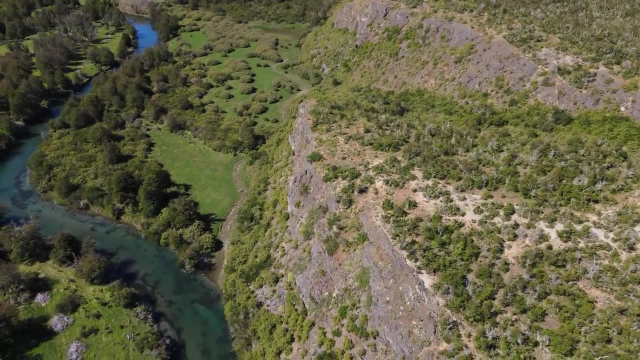 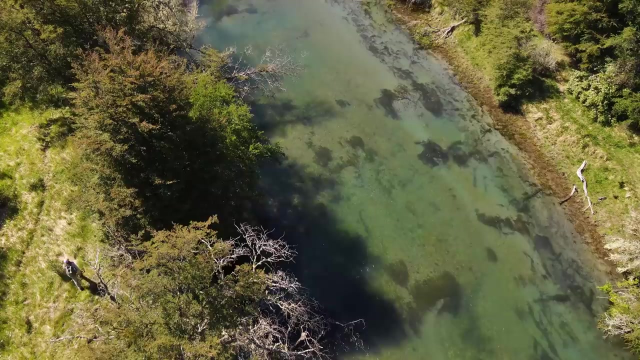 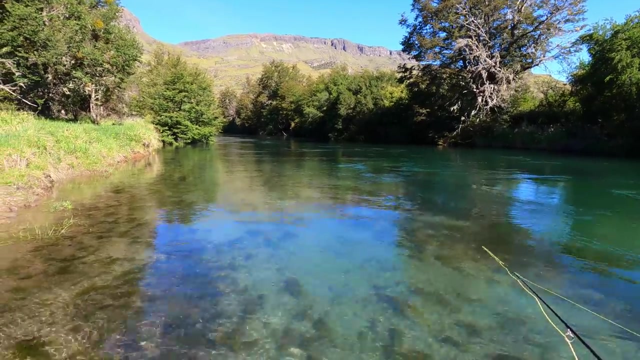 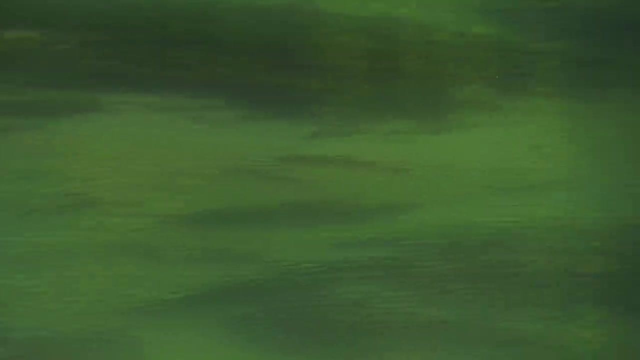 and, uh, deep, deep water too. so no chance. but man, that was super fun, loved it every moment of it. the visuals again were just awesome. let me know, okay. so I've just seen, I'll tell you when I'm gonna go. just seen him and I think my plan is to try to go upstream of him a few feet and maybe a few feet to his right. 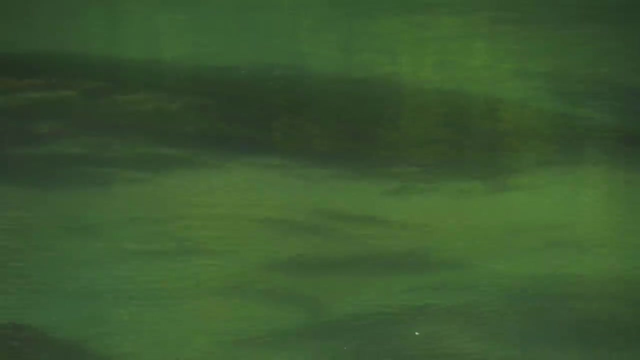 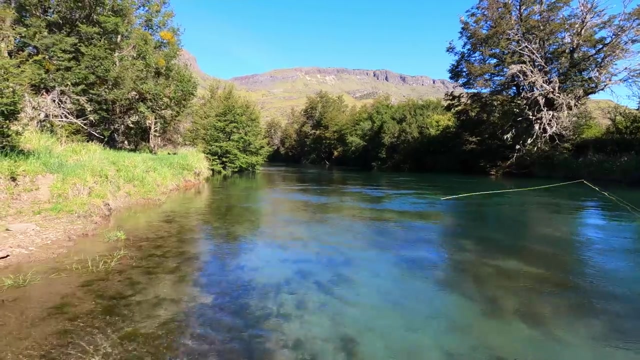 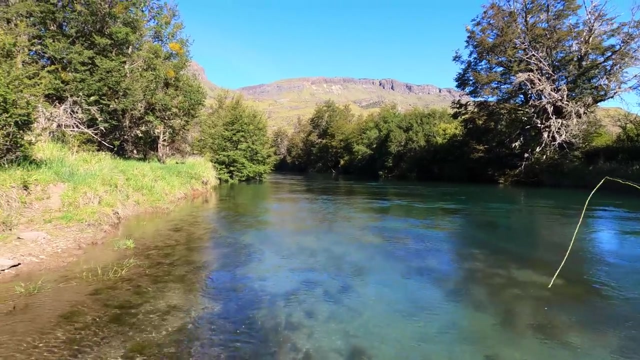 Dave, because that's where he keeps feeding. yeah, but you're gonna line them okay, I'll try to go left of him then. um, that's the hope. so I'm gonna wait on on that wind, I will go left, Dave, and it might be closer to five, six feet to his left. that wind is just causing, yeah, it's just causing- way. 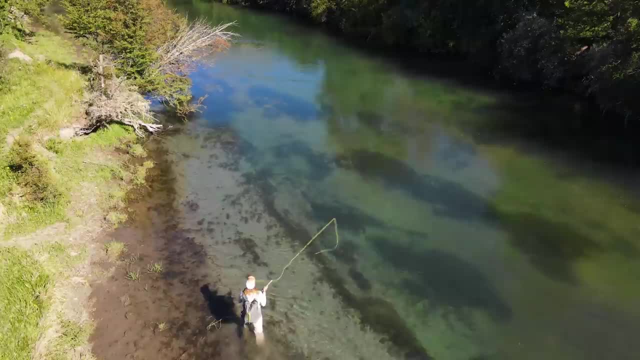 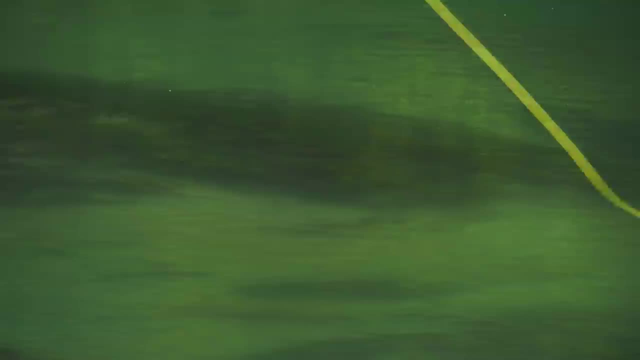 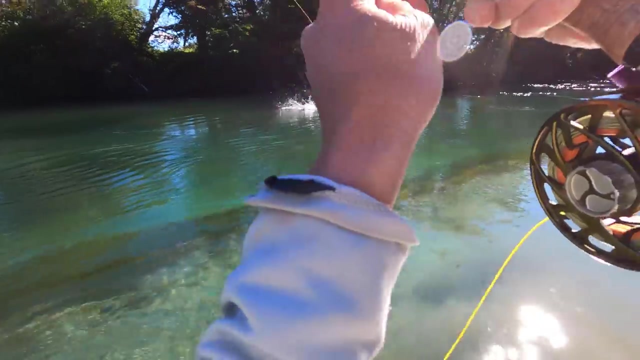 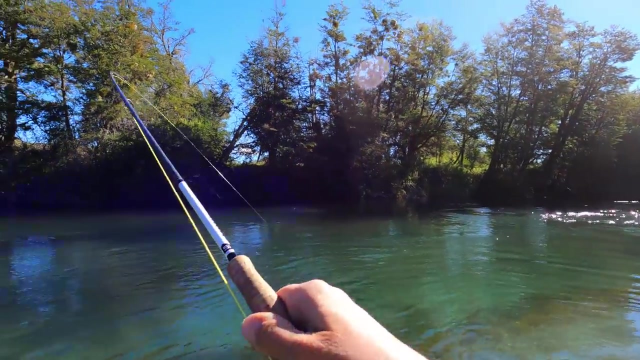 too much disturbance on top, guys, so that I can't see this smudge. here goes Davey, he's still there. yeah, oh yeah, hammered that stone fly, hammered the stone fly, come on, come on. yeah, yeah, yeah, what a fish. whoa, whoa, whoa. what a dance, guys, what a dance. oh my God. okay, let's try to do it here, if we can. 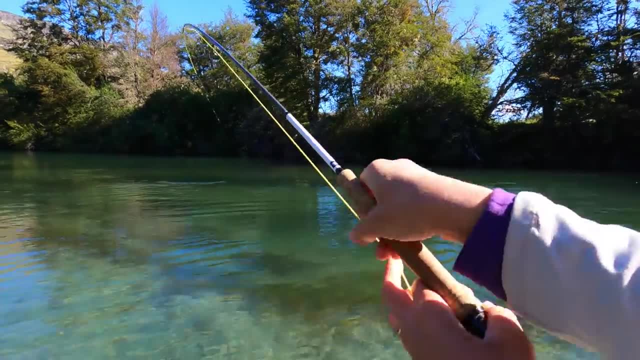 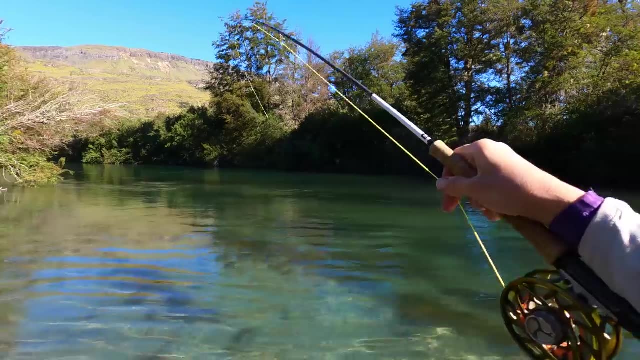 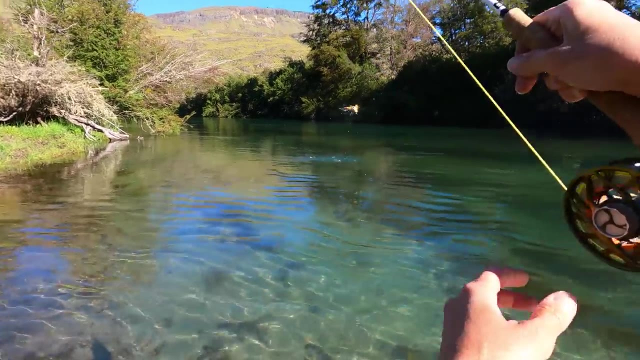 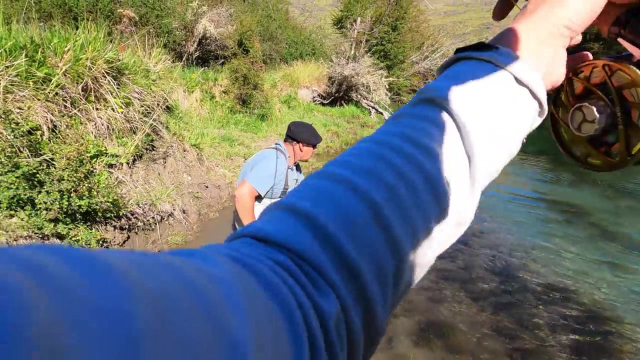 he's not done yet, of course at all, but that's awesome, that was fun. um, I'm gonna try to do. I prefer to do, if he lets me. marcello is up in here. maybe he's not done, he's jumping yet, but let's try in here. no, not to you. no, oh, no, no, no, no, yep, I know okay, whoa. 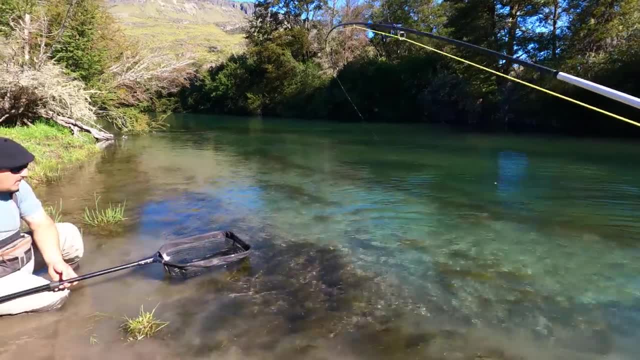 this is spunky, spunky brown. okay, I might get. need you to reach out with the net a little bit. when I'm ready, I'll try to bring him right over there. whoa, I'm gonna go get this fish. I'm gonna go get this fish. 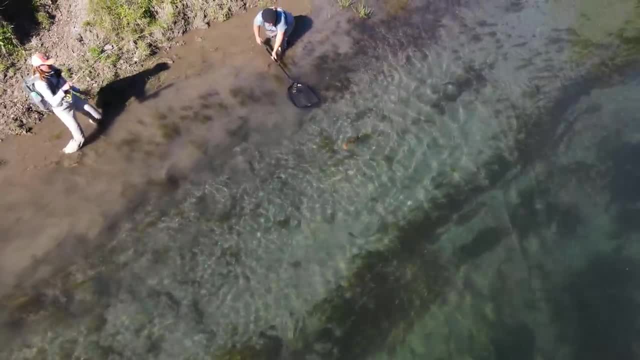 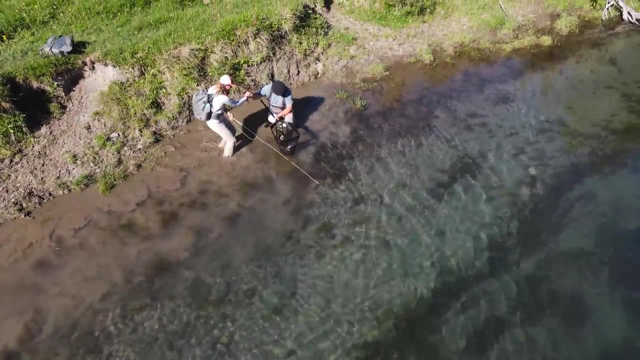 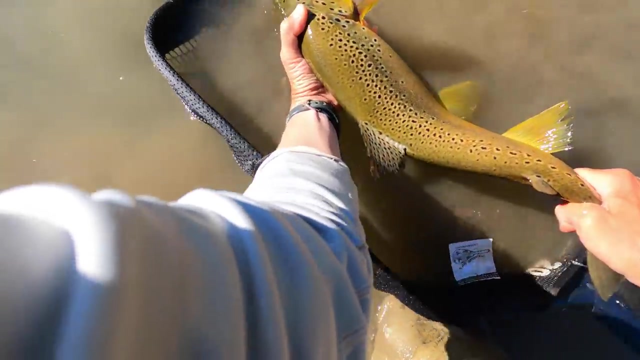 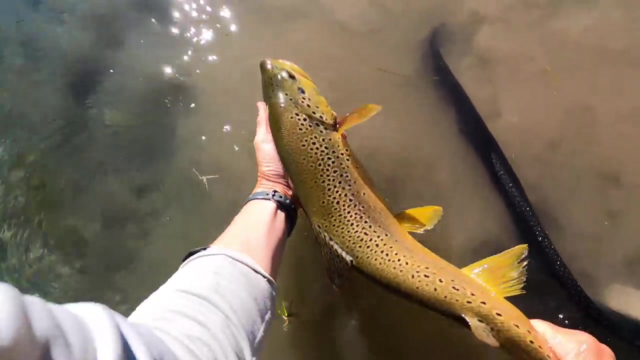 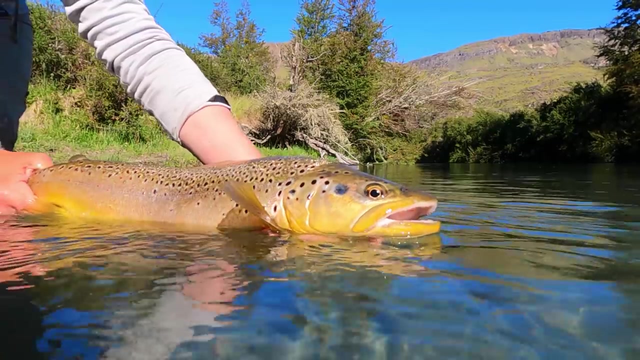 to you. but ain't it, here we go and walk it in, there you go. nice, awesome, wicked man, yeah, bueno, bueno, great fish. hey, Dave, yep, ready, flies are out. beauty, okay, here we go. all right to me, okay. and three, two, one. well, that was a hot fish, wow. 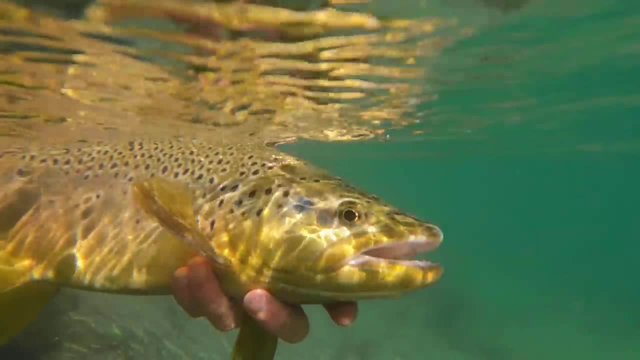 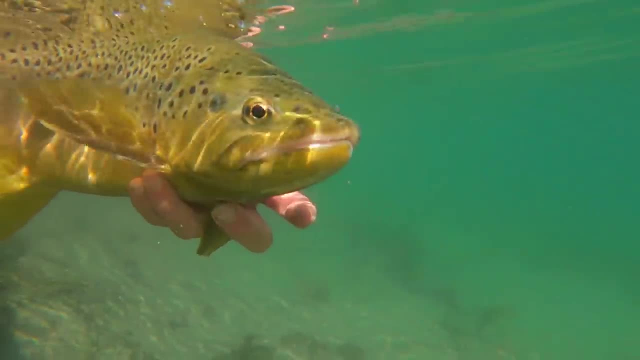 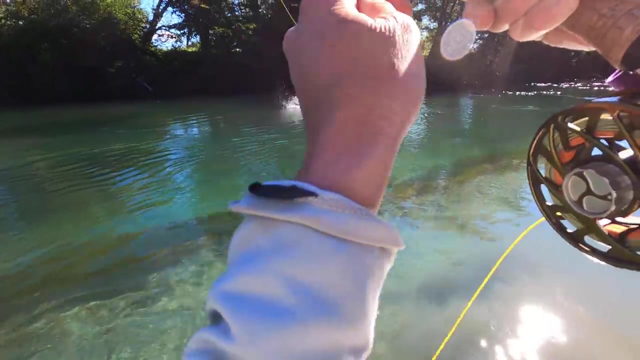 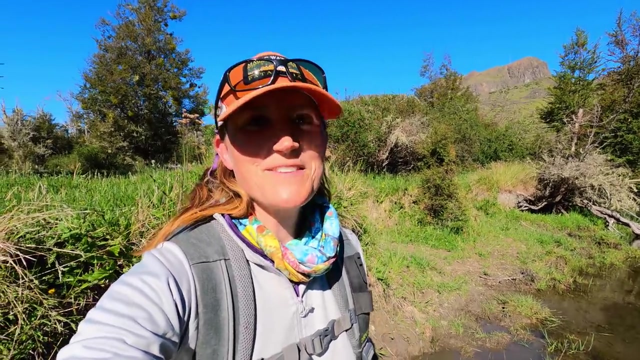 that stone fly, just gorgeous, eat on top. and once i hooked up, wow, that fight just had me going. i mean, talk about just a, a complete skitter right across the surface of the water below and then multiple other jumps. oh you know what? this is the kind of stuff that. 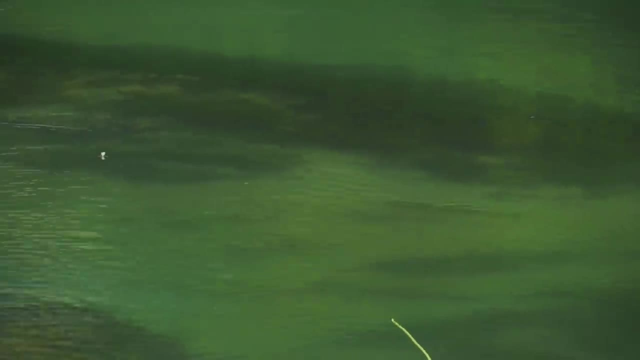 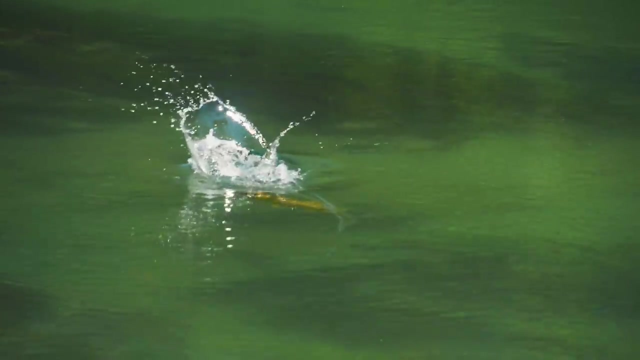 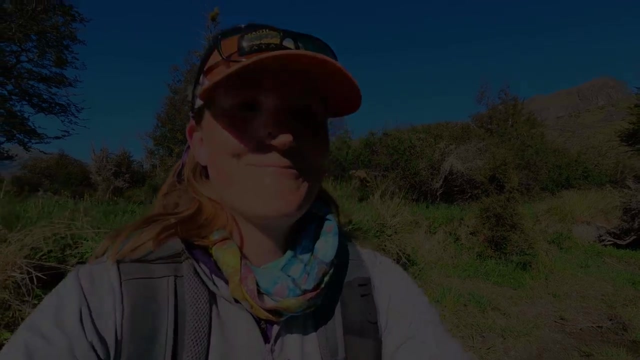 we've come here for, um, really love this particular water, piece of water that we're on, like a giant spring creek, very, very special spot to come and, yeah, just that was a moment that you just love every bit of it. you can't not, yeah, yeah, awesome. 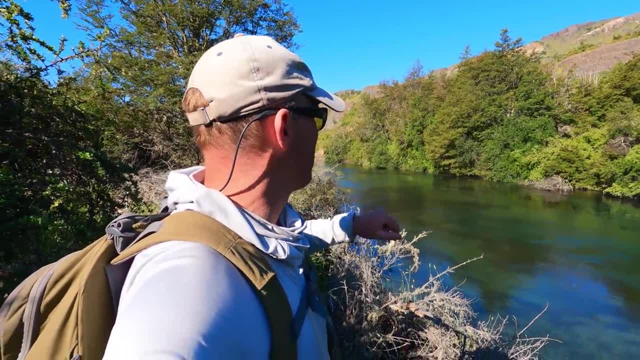 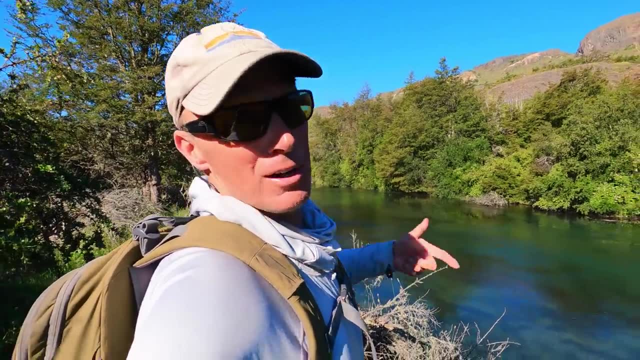 okay, guys. so i'm, i'm here. we're getting late in the in the day here, way out in the middle here. uh, it's kind of soupy, swamp stuff right in front of me and well, lucky for me, i spotted myself a rising fish way across the way. 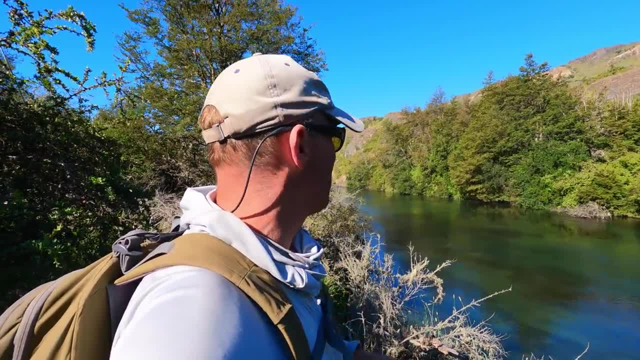 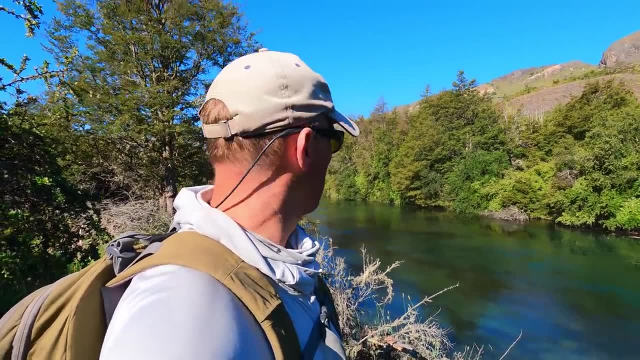 so, um, maybe a cast, maybe two. if it doesn't come, we'll move on. but i think i see him way across there, kind of. i bet you when i get out there, uh, waist deep in the water, it won't be a way across there, but it's a long ways. i'm just gonna get out here. i've got my 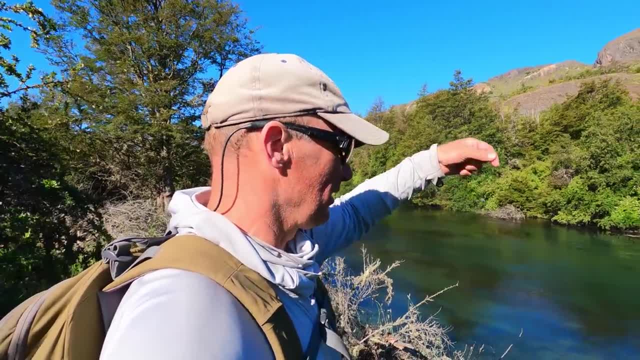 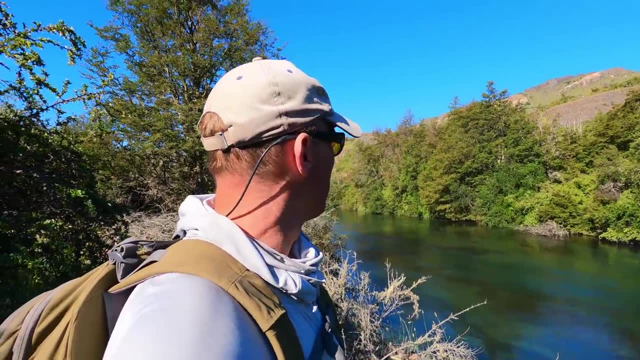 grace polywing stonefly on. i went with a little extra foot and a half of 4x just because i don't know where this fish is and i'm going to be crossing the sun as i land there. he is okay, good, um, yeah, that, just around that, that one patch of. 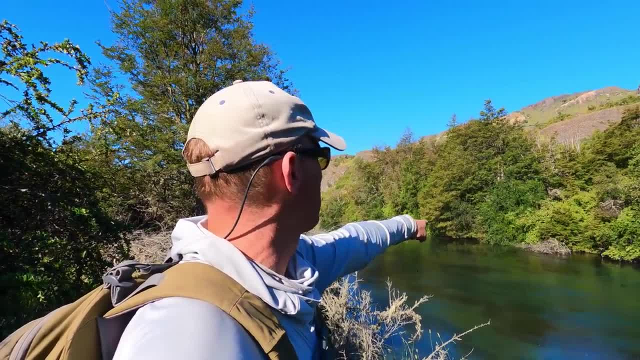 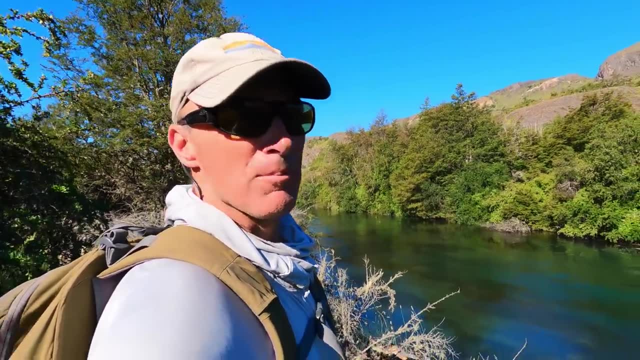 weed. the only one i'll be able to see from out there is that big heavy one. so i kind of have to try to cast, use the wind and kind of push across with a little reach and see what. we'll see what happens. in theory it should go fairly. 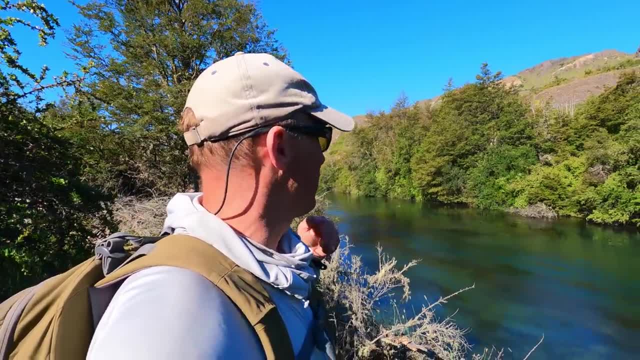 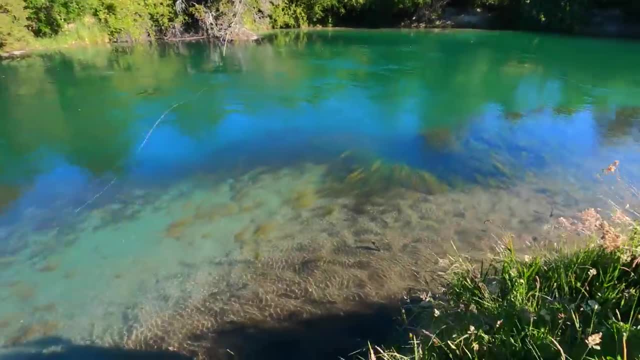 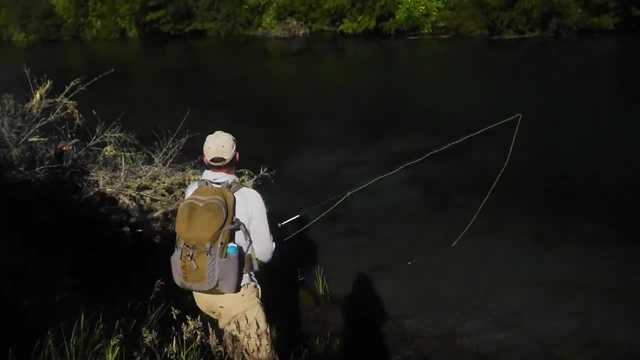 well, but uh, if it comes this way, when i go that way, it'll be over just as quick. so let's go give it a go, okay, it's easy spotting from here. when he comes up, oh boy, yeah, okay, and there's the soup. oh yeah, soup, soup too. 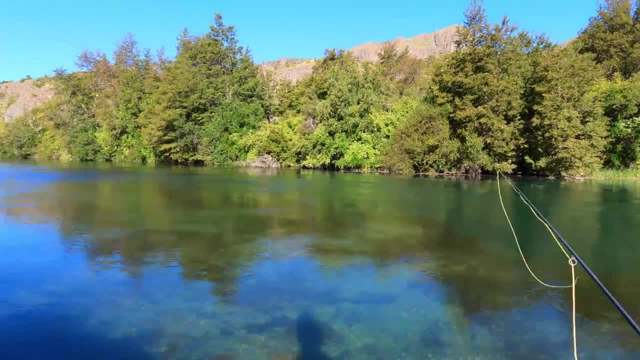 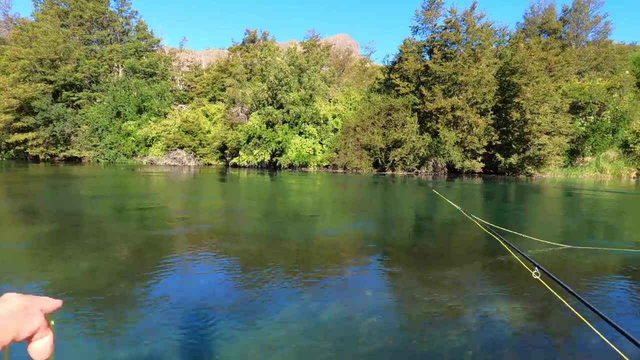 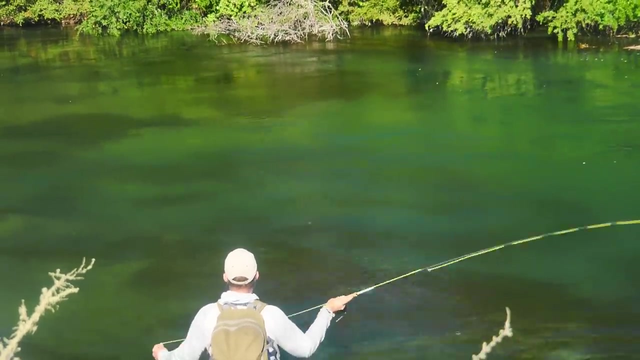 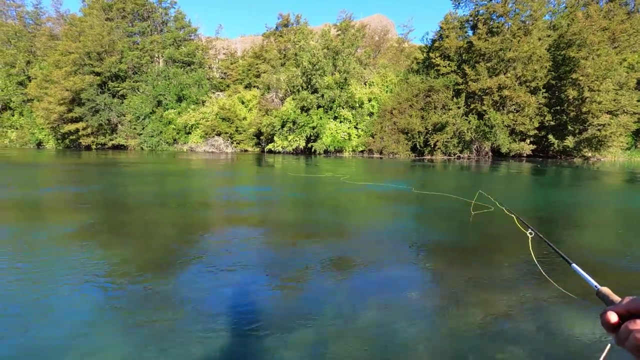 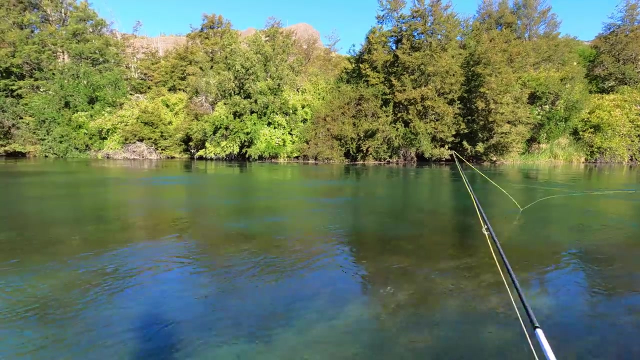 oh yeah, well, i'm waist deep right where that leaf is now. right, you ready, love, i'll give it a go. i'm gonna start short, as always. you know what i mean. i think that was what a foot, three feet, shy that way, and two feet up. 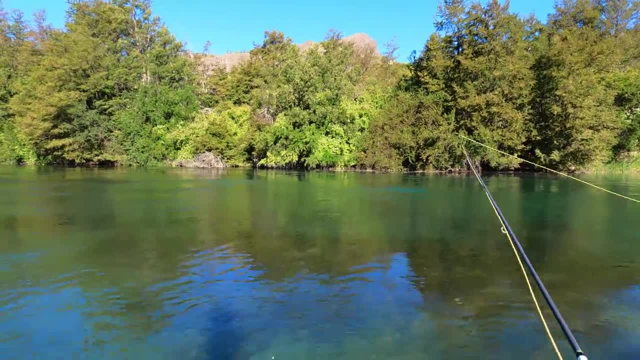 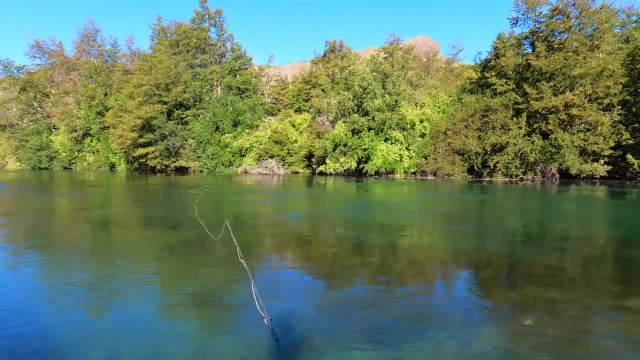 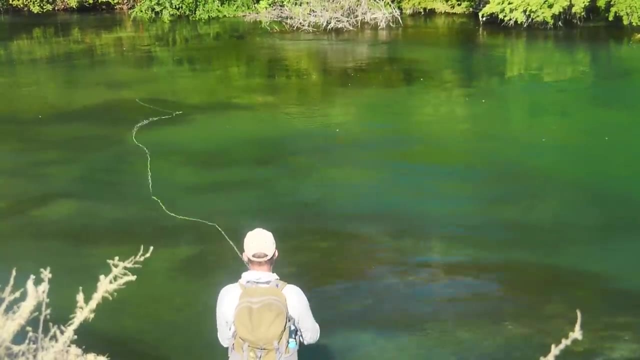 yeah, okay, um, trying to trying to see my way in there. okay, here we go. that should do it. strip like a son of a gun. start short, work your way in, and if you're too short, so be it, but if you're too long, it's over, right. 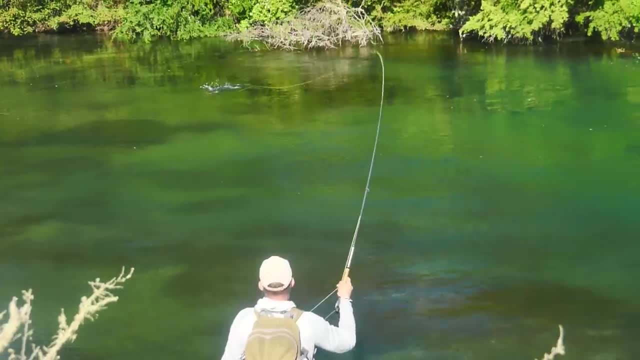 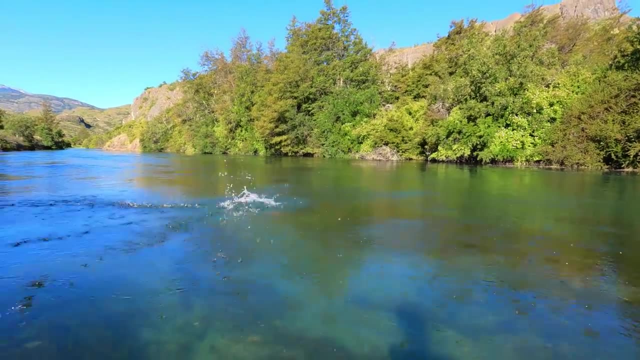 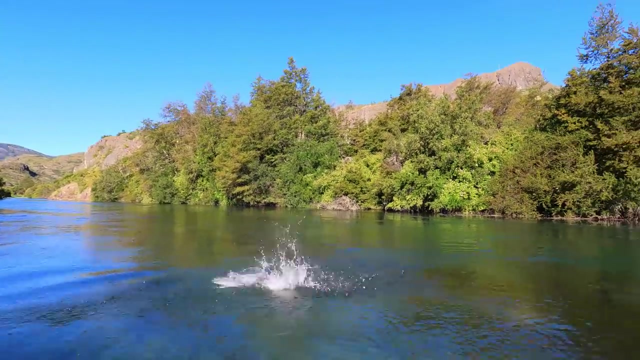 that's the whole kick of it all. i'm just gonna get my line- i don't know, yeah, i don't know- up. it's not that big after all. okay, i take that back. hot hello, yeah, maybe right here. let's see what he does, and he does that. 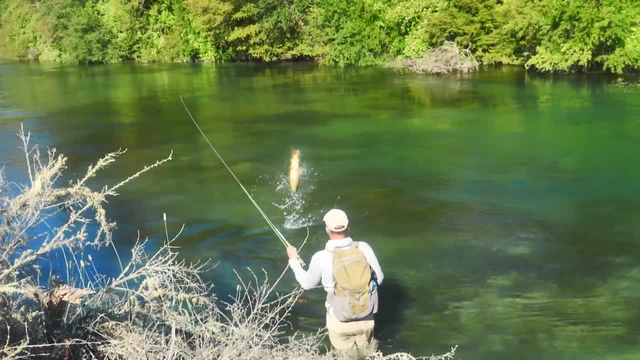 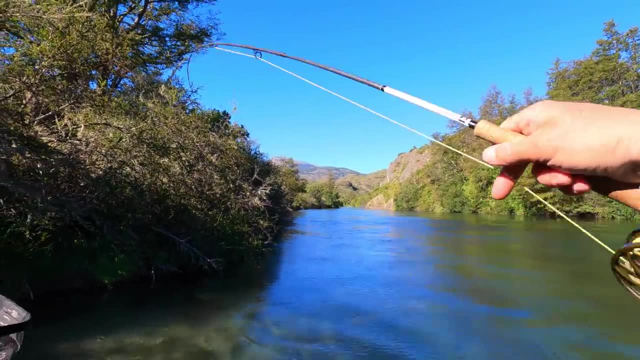 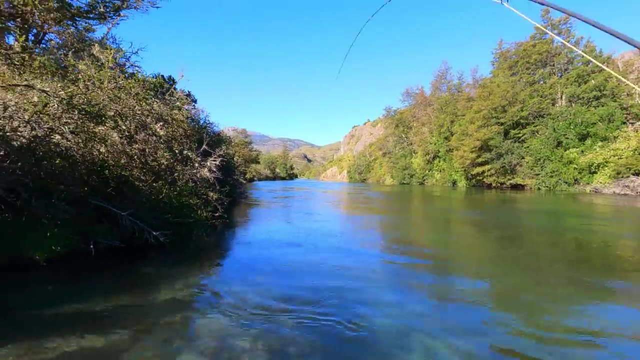 he does. he does flips, he does tricks, he does cartwheels. and if, if he holds there, this would be brilliant. oh, don't go in there, buddy, let's fold you this way. no, okay, let's fold you this way. come on, this is where that 4x might bite me in the ass. but see if i lift, i'm going to go. 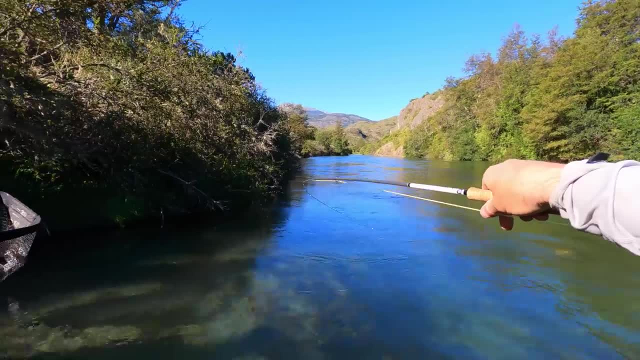 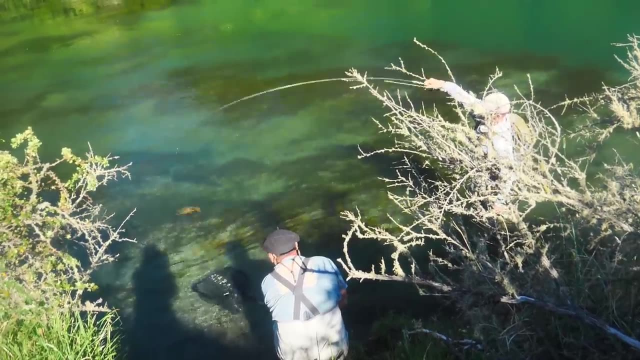 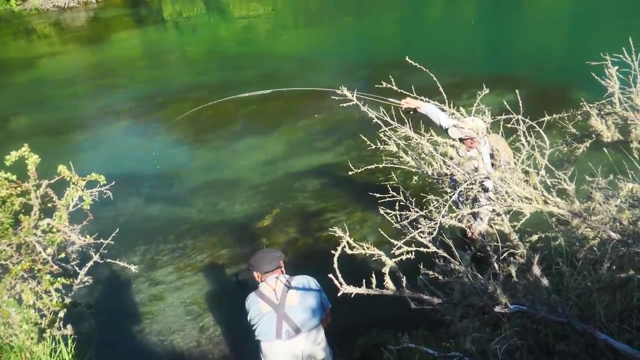 like this and try to fold them. no, he's not ready. he wanted to kick there again. okay, let's keep this low. put your net right there and in, in theory, in theory. no, he's gonna not like that. he has to fold. he almost folded there. there we go. come on, fold this way, bud. come on, you don't always want to fold. 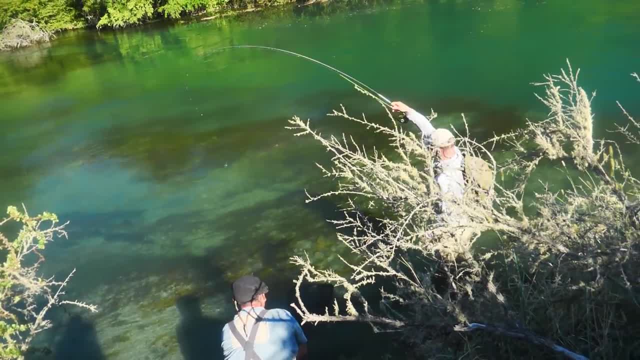 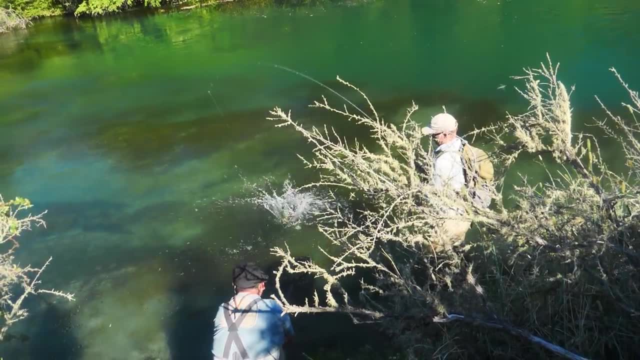 upstream. oh, you don't want to drag your fish upstream, always? okay, hang your line up there, take. okay, let's just get that over with um. really okay, one more, try, i'll do this. yeah, maybe try to walk them. i'll try to walk them and do a loop here. 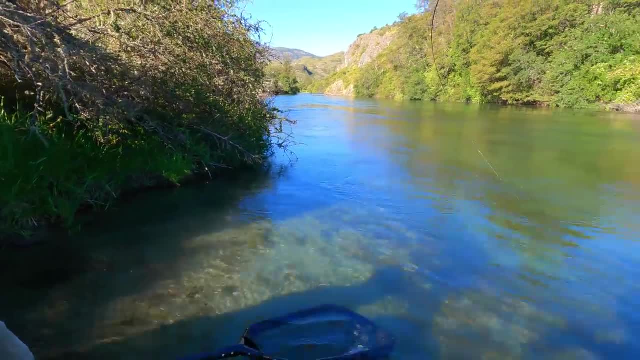 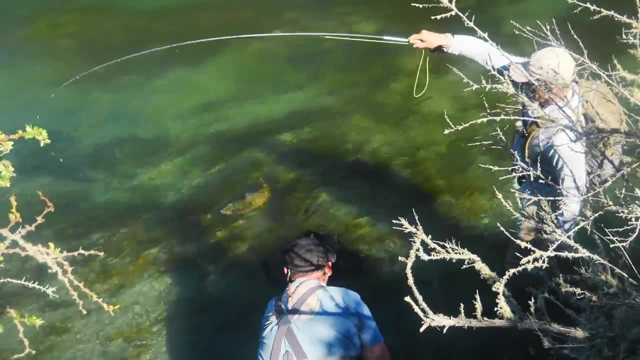 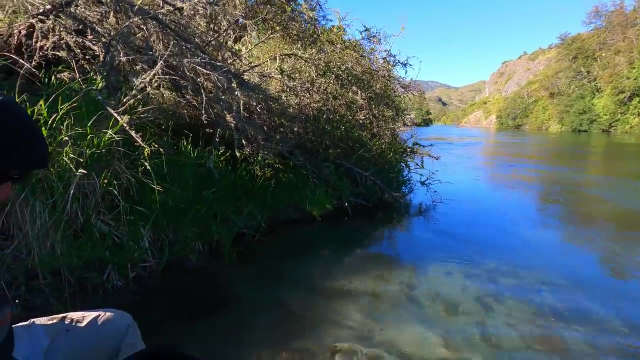 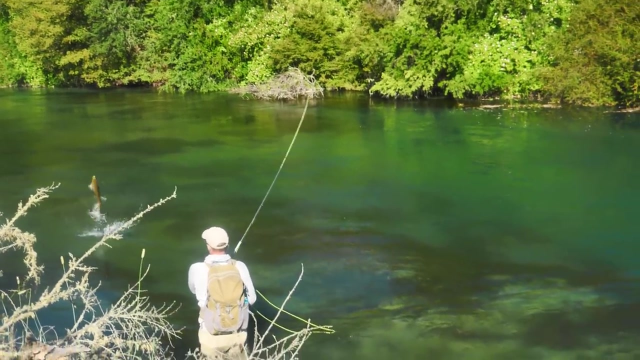 what do you think? will you let me do a low loop? one more try. i don't want to bend this hook out. come on, we're going to fold them. will they fold right? there there we go. wicked nice job, mister. thank you, ah gracias. very good day again, jeepers. hey, amazing fish. 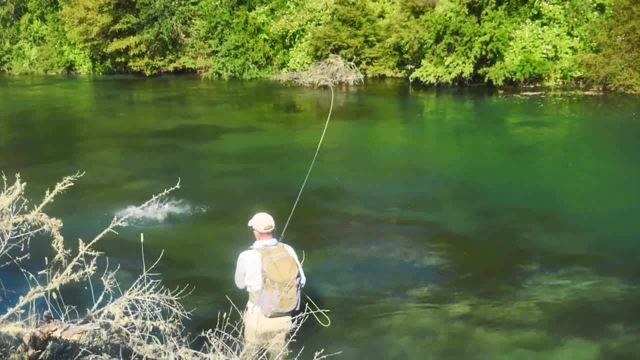 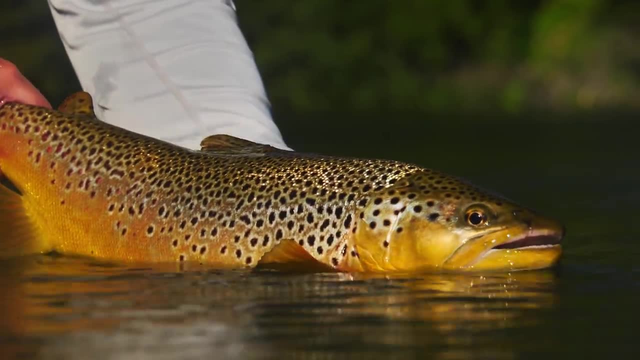 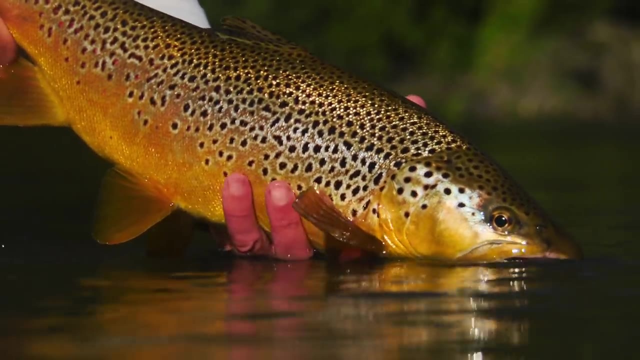 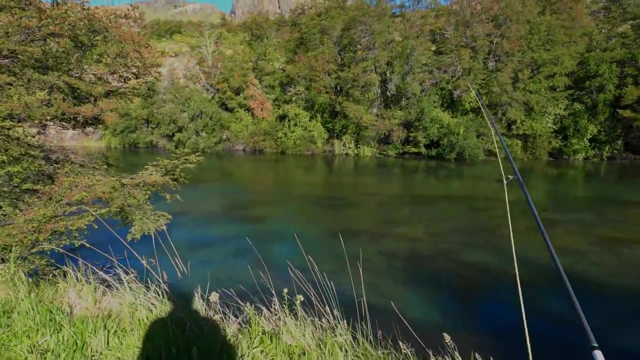 gorgeous, gorgeous fish. i am now. what a fish. hey, okay, get up for me to try to get. okay, one, two, three. it's absolutely stunning. okay, i'm gonna go down. you ready? yeah, here we go. what a stunning fish. yeah, gorgeous fish guys. our poor guy marcelo thought he was gonna have a coke here soon, but 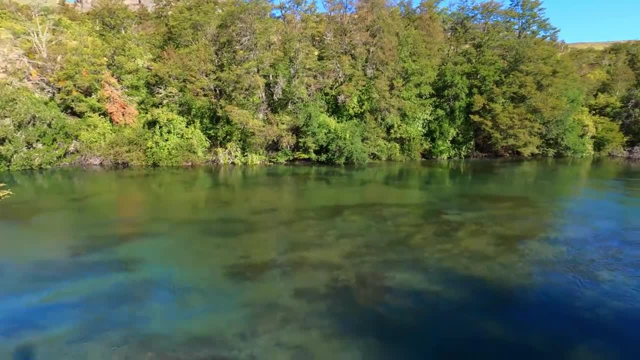 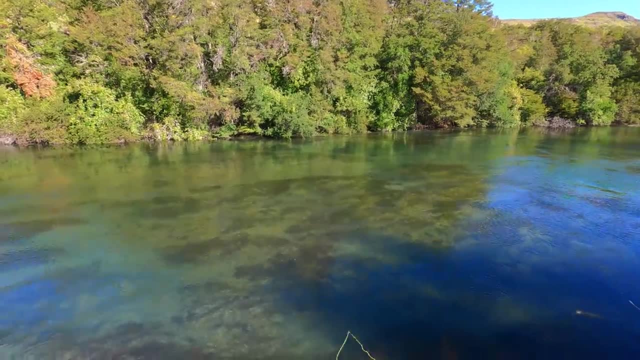 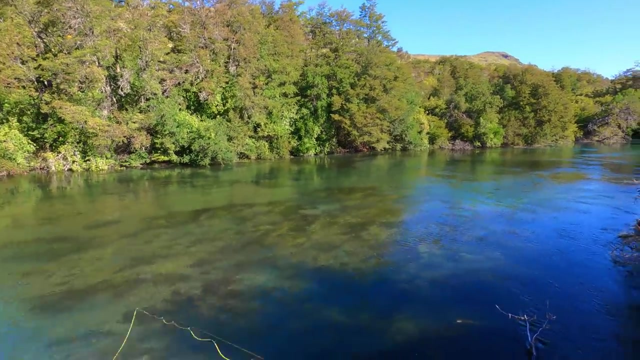 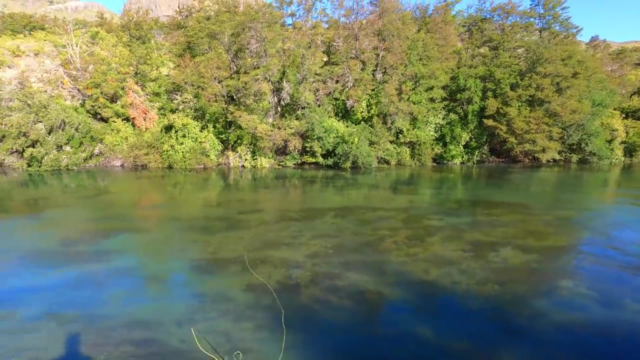 nope, there's another fish. and when there's another fish, no coke for you there. oh see, that's what i mean, okay, um, yeah, that's that's a long ass cast, isn't it? well, that's the same fish, yeah, okay, well, might have to keep coming around here. oh, now, look at that thing go. 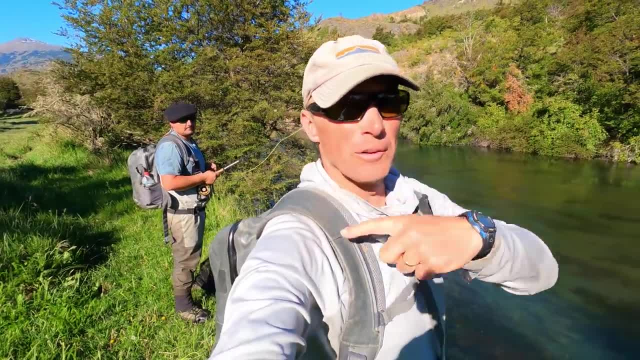 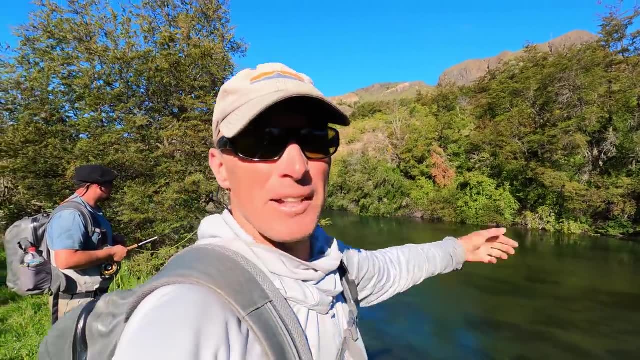 okay, guys. so as i was just saying, hey, um, he thought we were gonna go home and get ourselves a coca-cola, but no, i'm gonna. there's a fish over there. i could launch a bomb and cast, but i'm not gonna get there. so easiest way to. 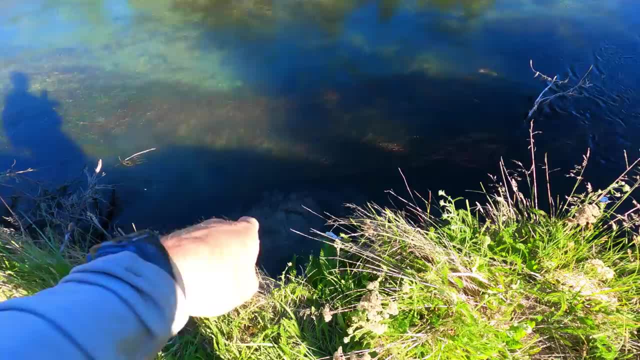 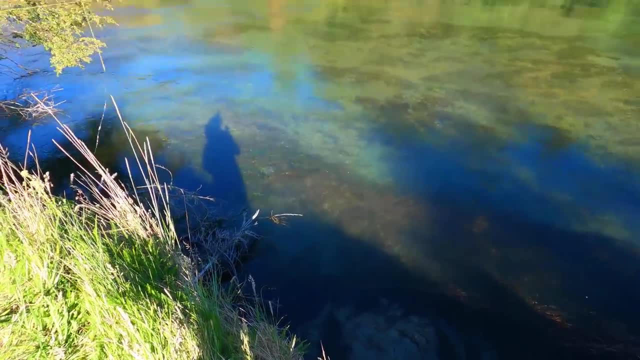 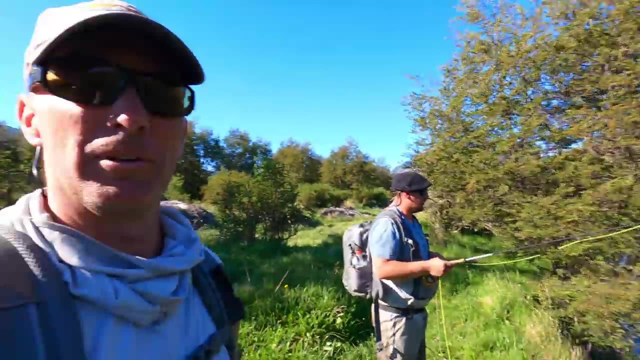 is to get closer, move my feet. trouble is i'm gonna be well through here. somewhere is over waist deep, yeah, whereabouts, where? oh, the original one? yeah, okay, so there's still two fish there. let's- uh, i gotta get out here. stole emilia's waterproof backpack so i could clip on the gopro. 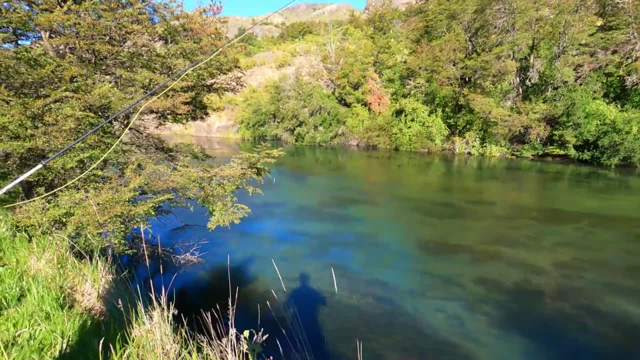 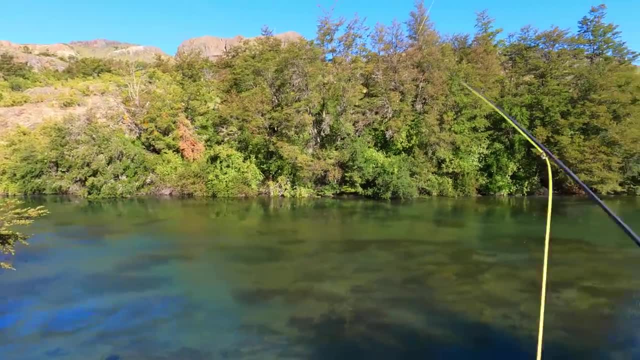 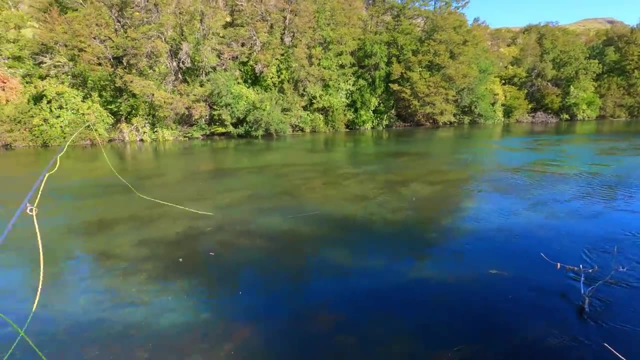 let's, uh, let's- try this. see if, moving my feet and swimming at the fish, you're gonna come out with me and swim, right, marcelo? no, let it go. boom, boom, boom, yeah, right about now with a coke, hey holy, yeah, there could be smarter ways of getting in the river, but that's a good way to go. 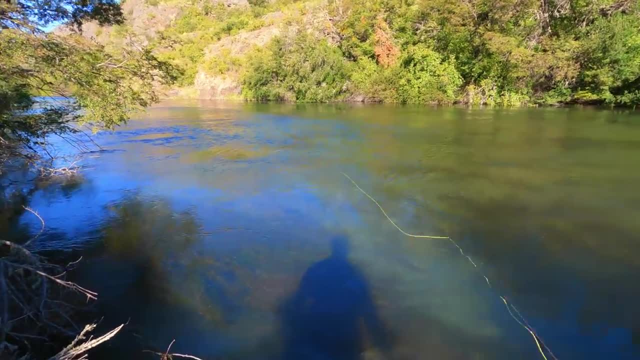 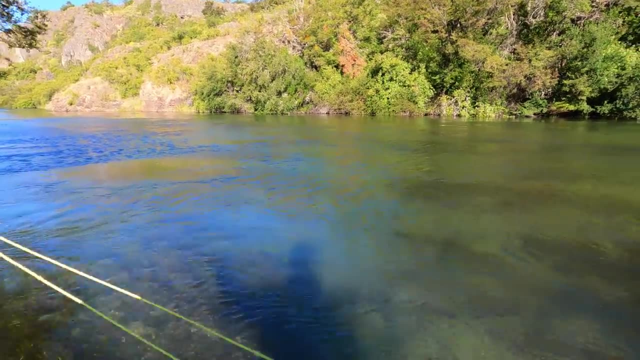 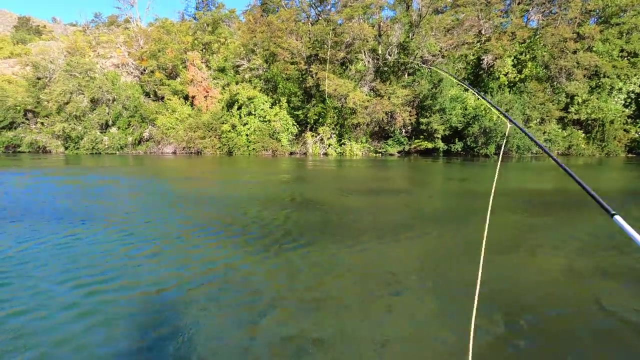 that's the most big rise, you, okay? so that's step one and i'm just going to ski down that slope. okay, i'm not going to take too long, i hope. okay, i've got to try start short. right, just keep working my way across, because we know there's a second one. 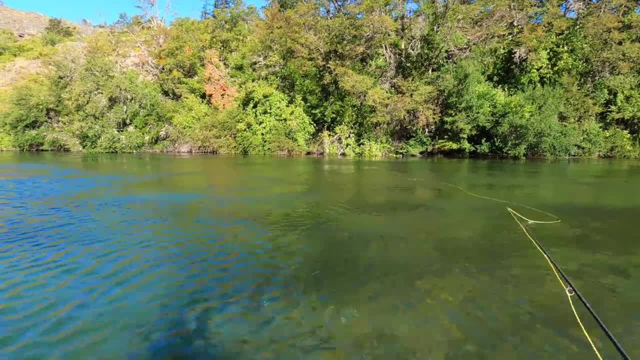 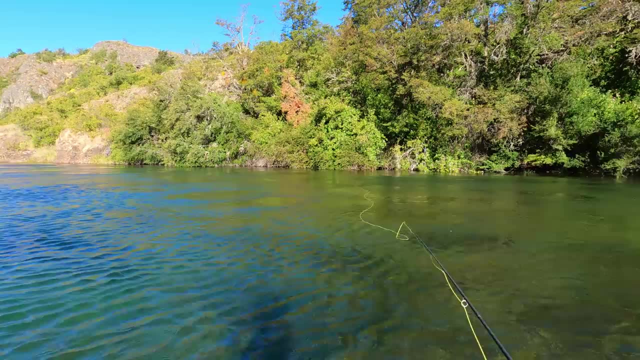 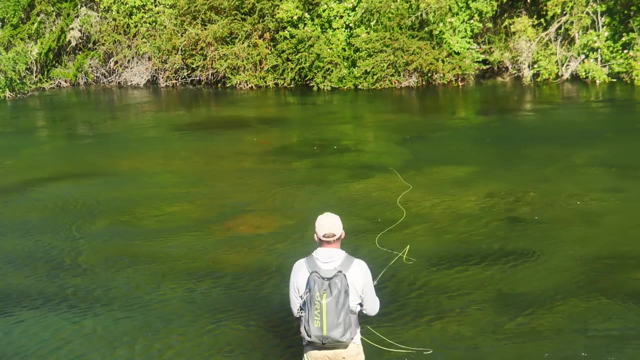 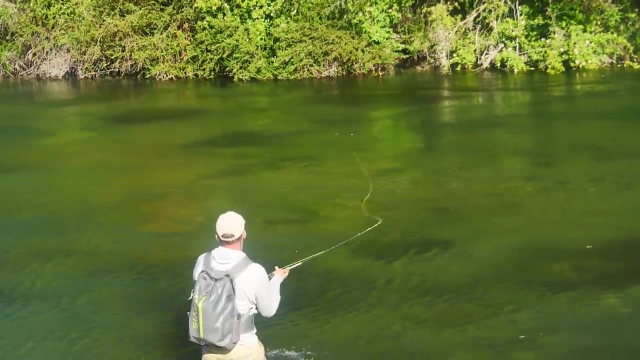 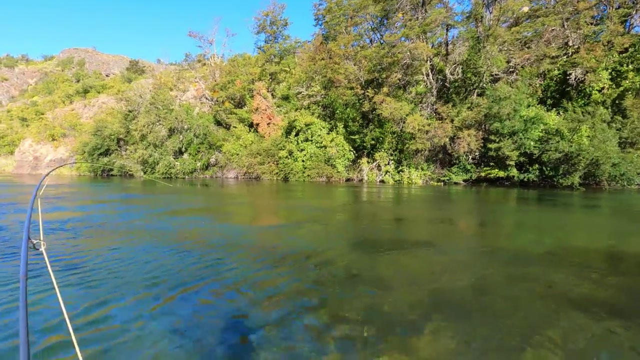 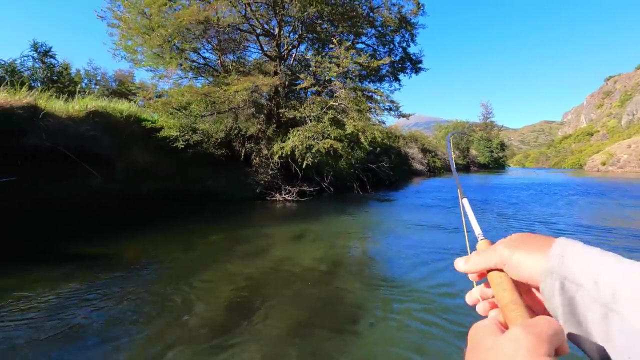 somewhere out there a little further upstream, kind of like fish that one got, ah well, that pooch. the second one. okay, come back, come back, here we go. yeah, i'll try to get them over, just back walking backwards. it's the kiwi way, okay, no, no, i don't just extend your net. 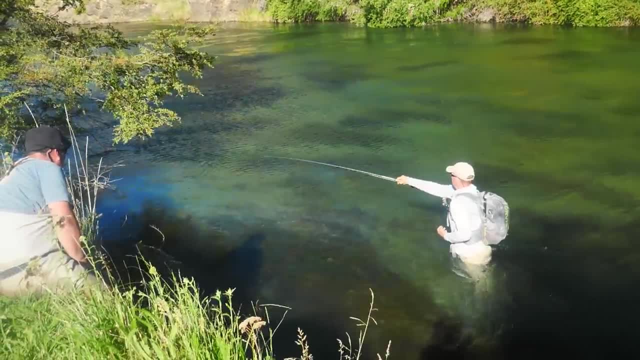 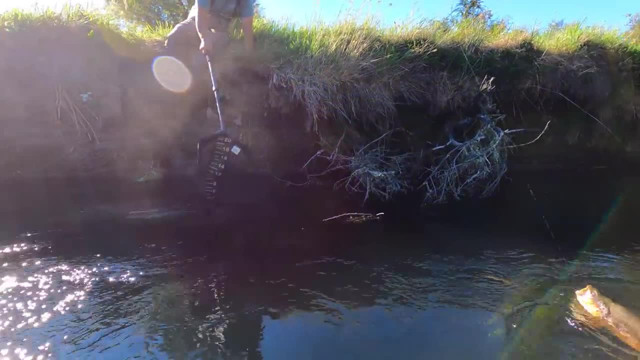 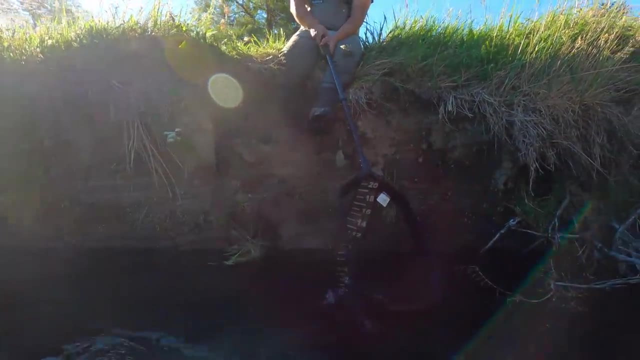 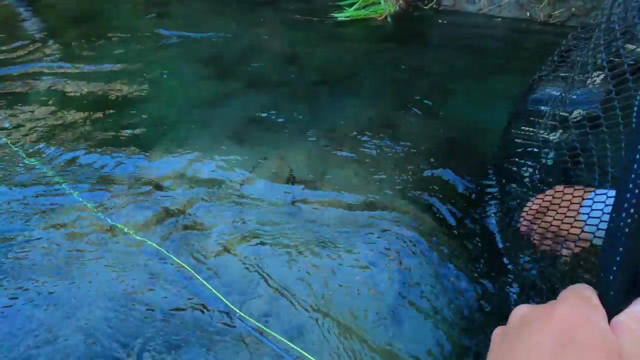 we'll see. it's not that big. no, we'll get there. let's just see. don't worry too much, right, yeah, there in the net. thank you, sir, here let me do you just stay there. mills, yeah, and here, yeah, i'm gonna. that's a gorgeous take.